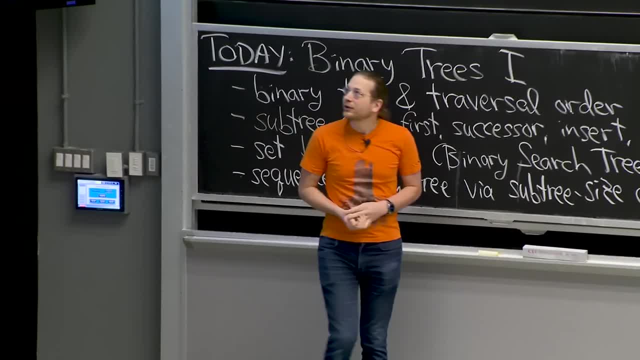 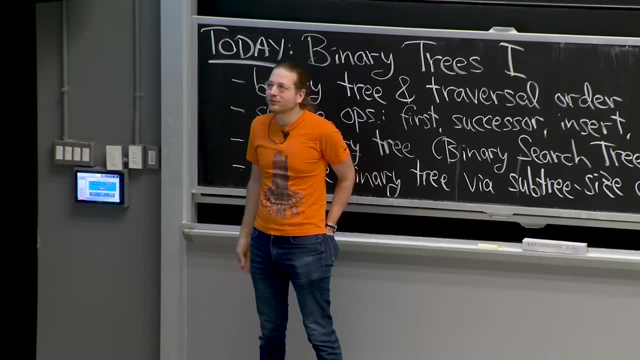 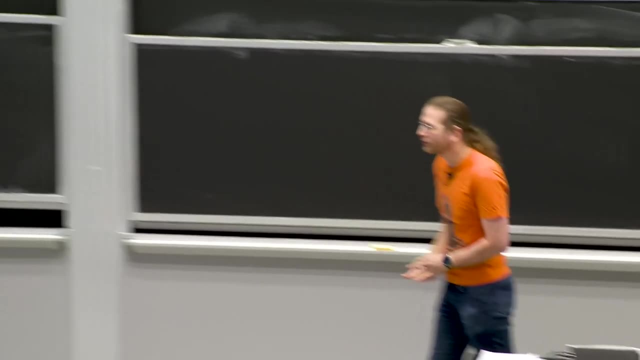 if you make any changes, you have to do the shift, which is very expensive. So today, or sorry, next lecture, for the first time we will see all of those operations efficient. I'll mention our goal. We're efficient means logarithmic, So we're not quite as good as linked list and dynamic. 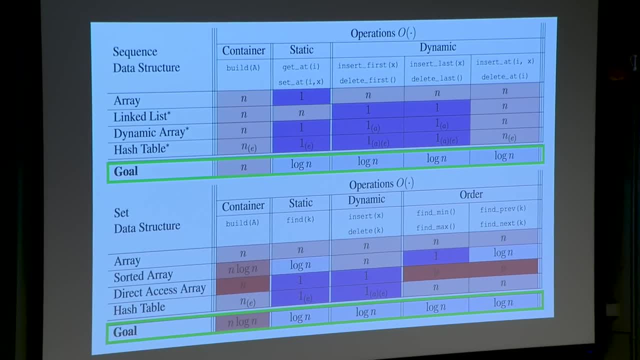 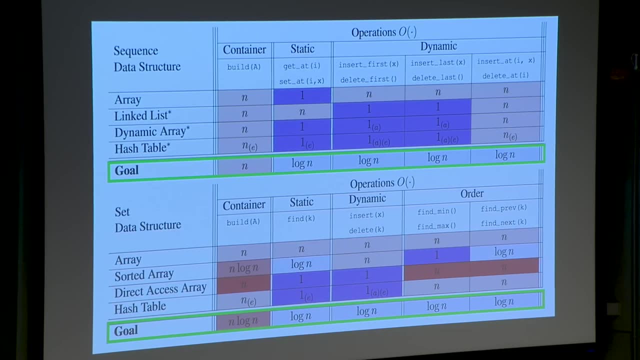 arrays, at inserting and deleting at the ends, those there that we achieve constant or constant amortized time. But up to this log factor we're going to get the best of all worlds where we can solve all the things, all the operations that don't build or iterate through. 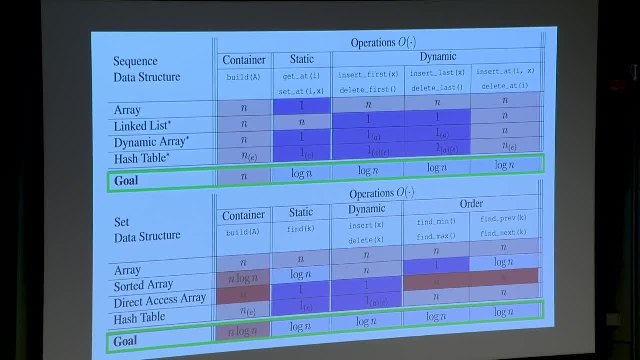 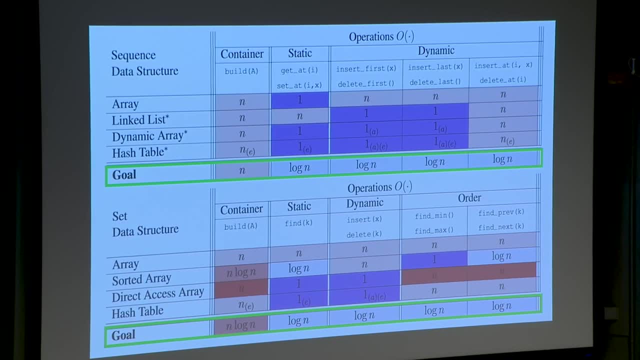 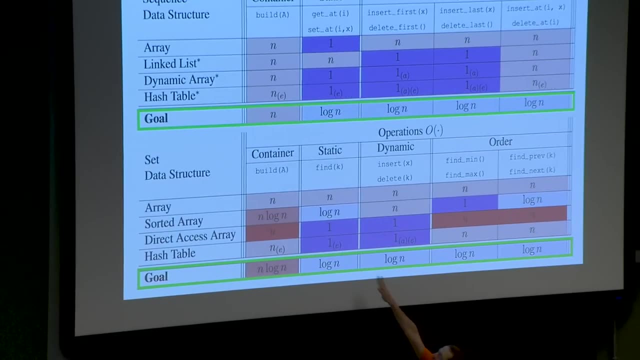 sure that we're doing the best we can. We're making sure that we're doing the best we can. We're maintaining a bunch of items which have intrinsic keys and we want to search by key. So hash tables are great if you're only doing exact searches, If you want to find a key. 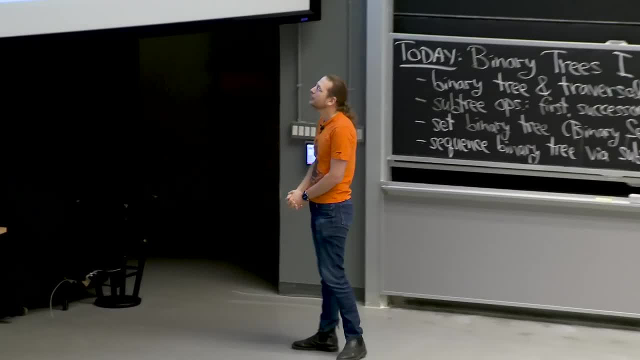 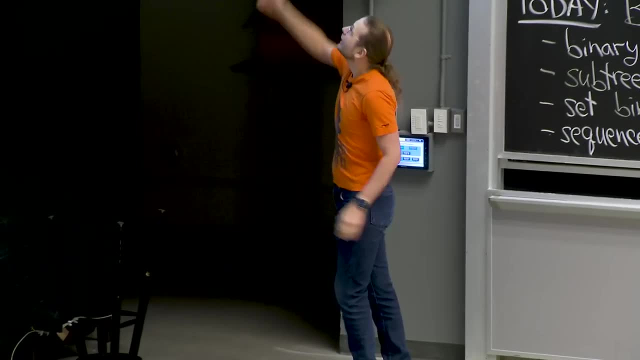 and get yes or no. is it in there? And if it's in there, give me the item. That's what Python dictionaries do, And they're great at inserting and deleting, but they're really bad at find previous and find next. This is the unsuccessful case If I search for a key. 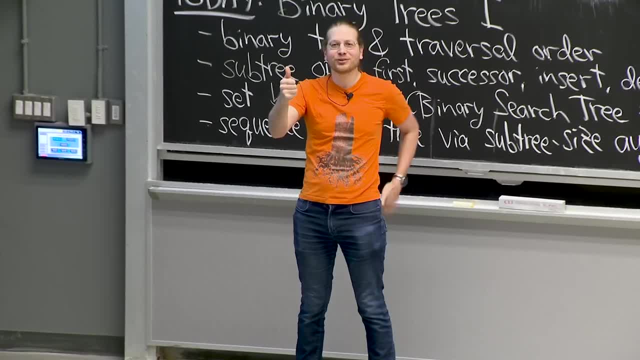 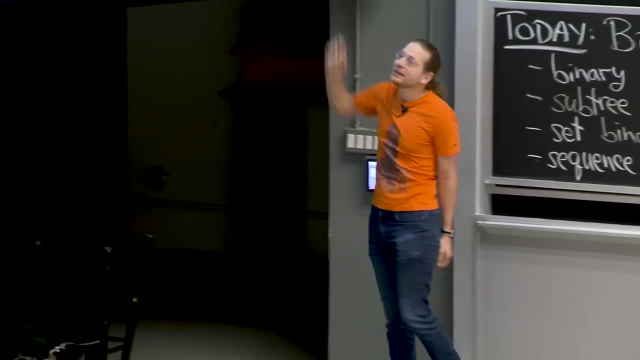 and it's not in my structure. I would like to know more than just the answer. no, I'd like to know what the previous and next items that are actually in the structure. So what are my nearest matches when I search by key? That's a natural query and the only data. 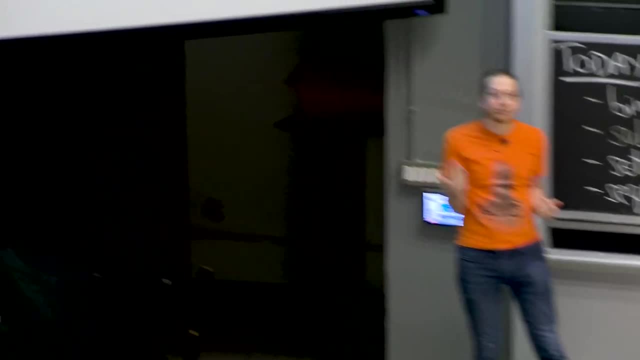 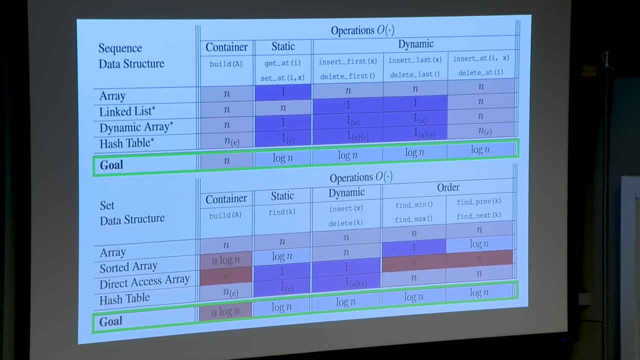 structure we have. that's good at. it is a sorted array, because binary search gives this to us. If we search for a key by binary search and we don't find it, the position that we end up at is right between the previous and next one. But of course, sorted arrays are. 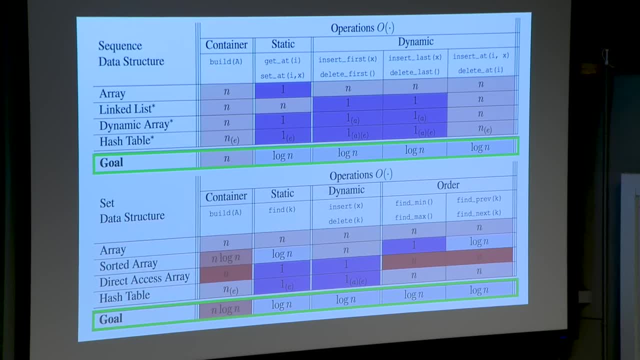 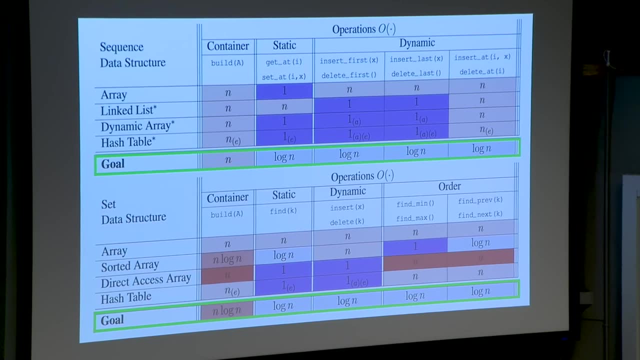 terrible for dynamic operations. We don't know how to maintain, we can't maintain a sorted array without any gaps when we're doing insertions and deletions In some sense today and next class binary trees. let us represent a sorted order or, in general, an order of. 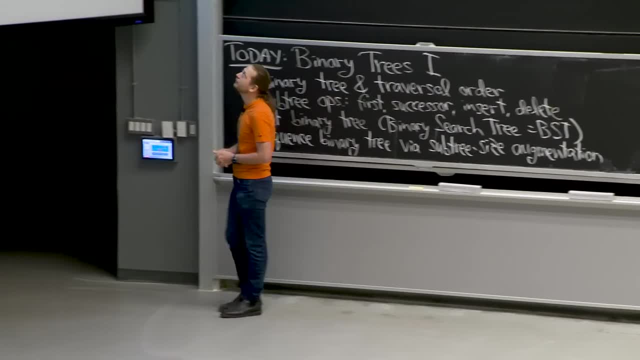 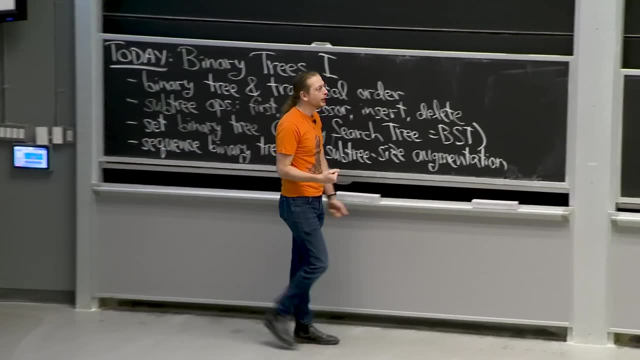 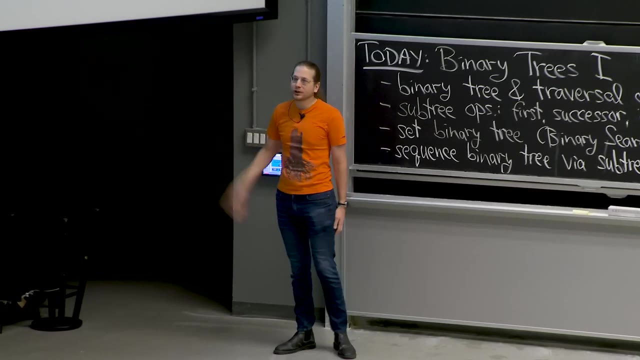 items dynamically and still allow us to do very fast things like get at of i and find previous of the key. So that's our goal. We're not going to quite get to this goal today. We're going to get An incomparable thing called the height of the tree, and then on Thursday we'll be able. 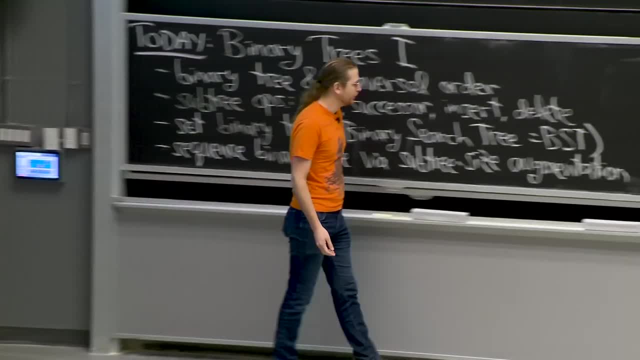 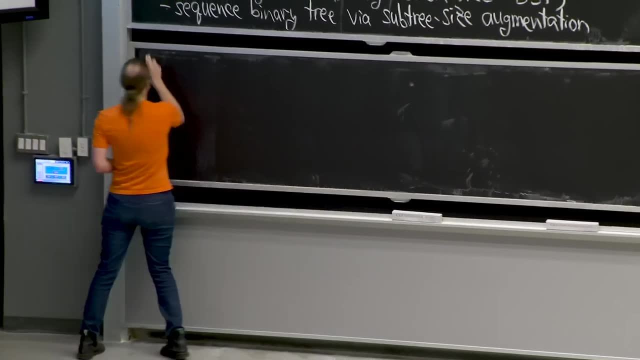 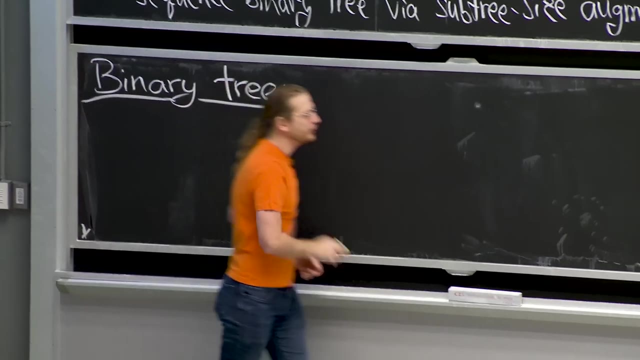 to finish and achieve this goal. Today is just in service to that goal. So what is a binary tree? Let me draw an example and then define it more precisely. Mathematicians will call this a rooted binary tree. in case you've seen that in 042, say: 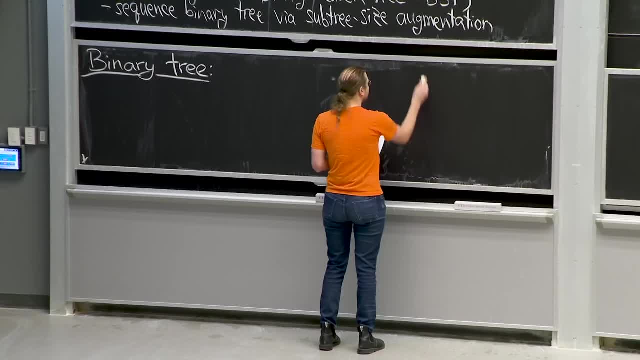 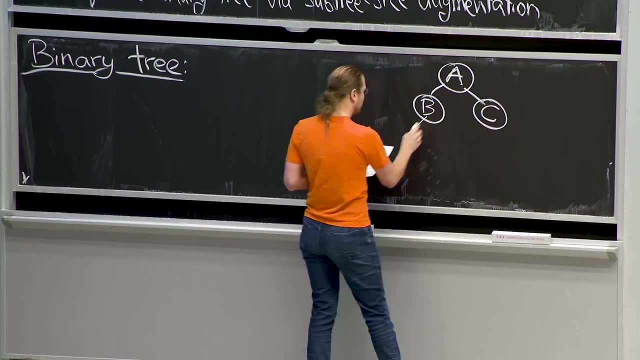 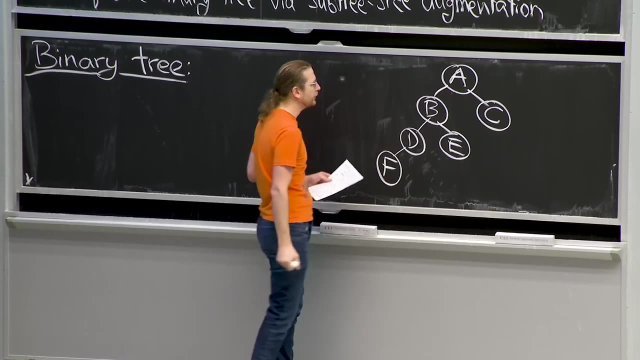 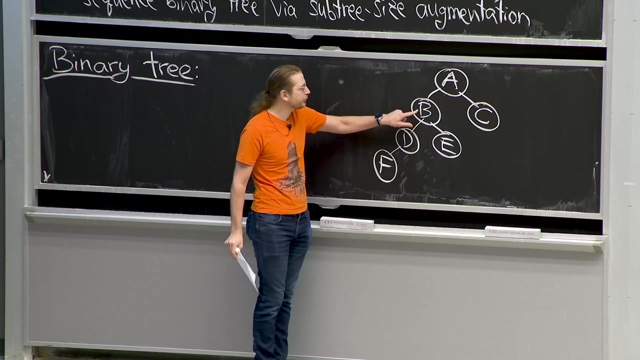 Just turn this back like it's проверed. Here is a picture. This is an example of a binary tree. It has a bunch of nodes which we're drawing in circles. It has items in the nodes which I'm writing as letters here. So this is item A. item B: item C And it has a bunch ofTurnedOrdrealscom which is an example of a B nós Un Edinburgh and becomes really difficult because it knows things like that All the time. when we take ce komun合分 we see I'm leaving this mouse button and my cursor who comes in and we imagine: that you give some kind of error, that will appear in this box where I've got a n-th, our exclamation mark. Like I do that, like literally count the visits of users, like: OK, see my answer on the next question, next one, and, and this one comes in and probably the next part goes. 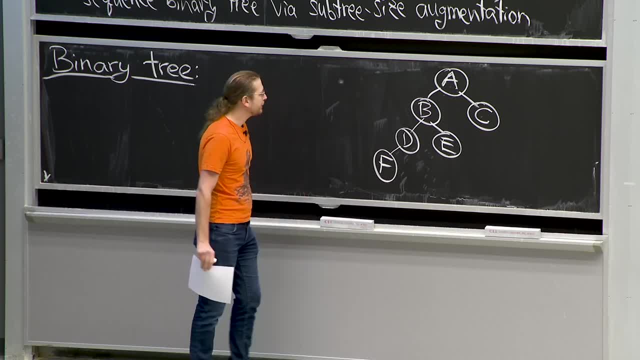 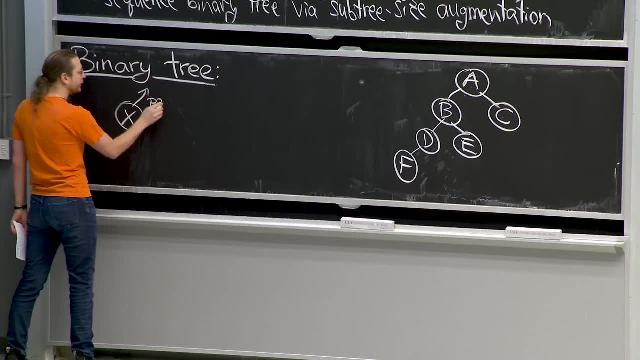 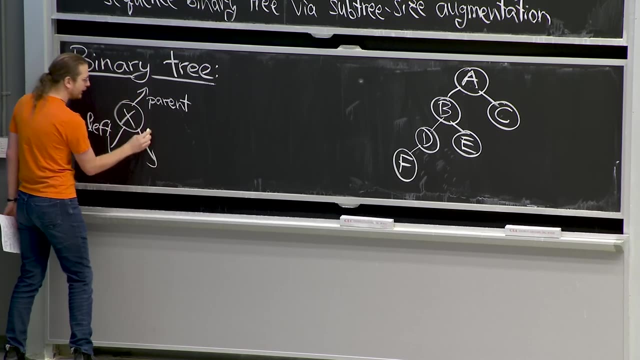 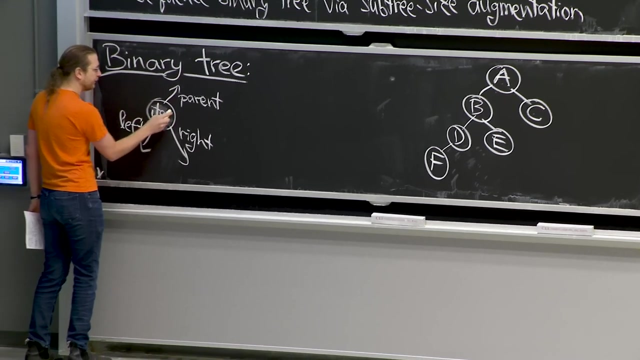 has these links between them. This is like linked lists, But in general a node x is going to have a parent pointer, a left child- left pointer and a right child right pointer, And it also has an item inside of it. 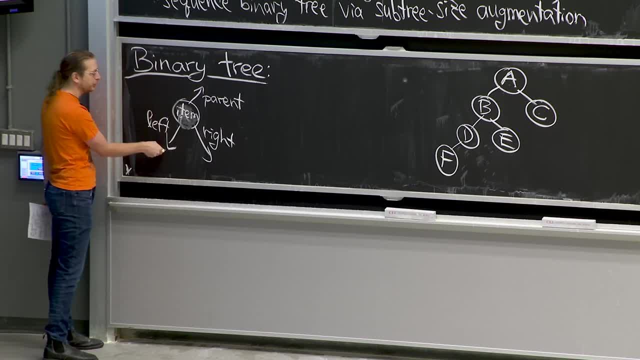 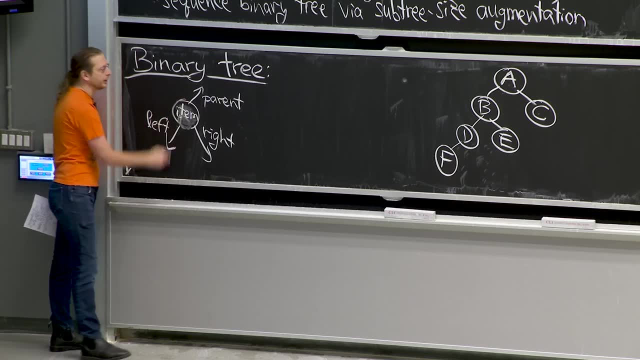 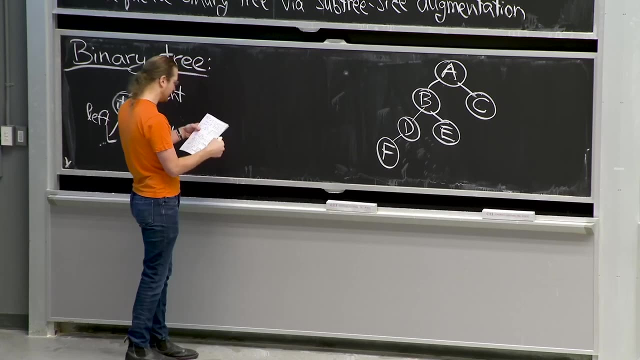 So I'm going to talk about. nodeleft is a pointer to the node down here. Noderight nodeparent nodeitem gives me. So if I look at the node A, its item is A. So let me draw for you some examples. 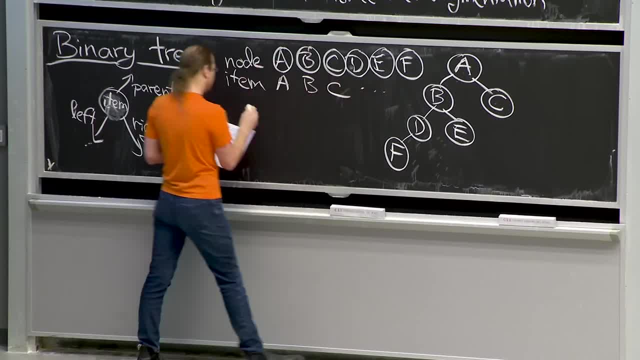 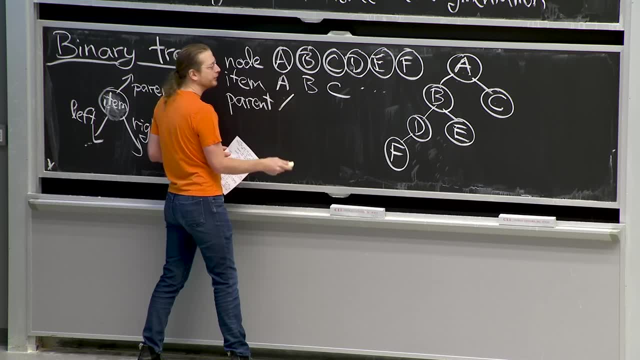 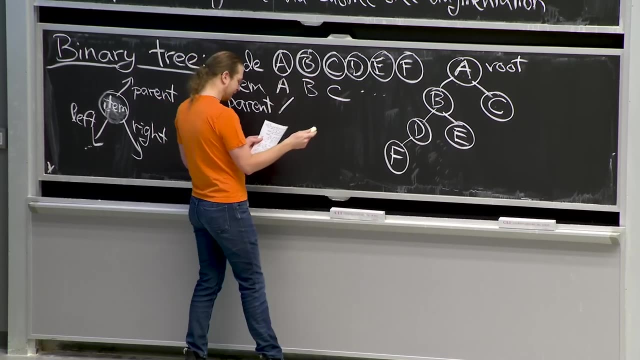 OK, the parent of A is nothing, So we call A the root node. There's going to be a unique node that has no parent. It's sad to have no parents, but there you go. Then we have node B, whose parent is A, node C: 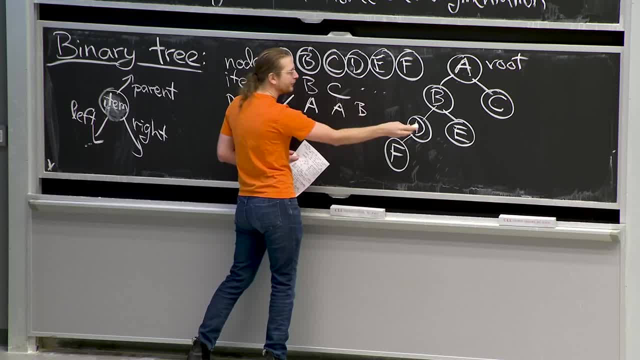 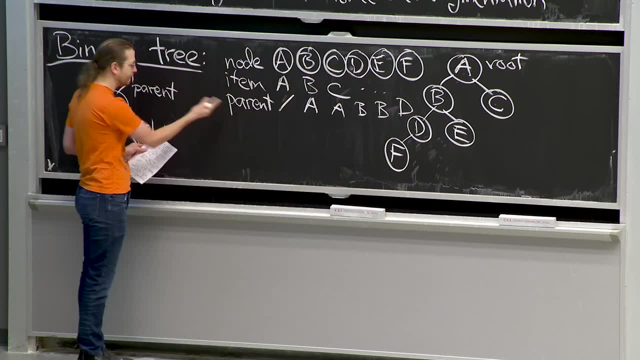 its parent is A, node D, its parent is B, node E, its parent is B and node F its parent is D. The alphabetical order here happens to be ordered by parent. Then we have left pointers. I'll just do a few of them. 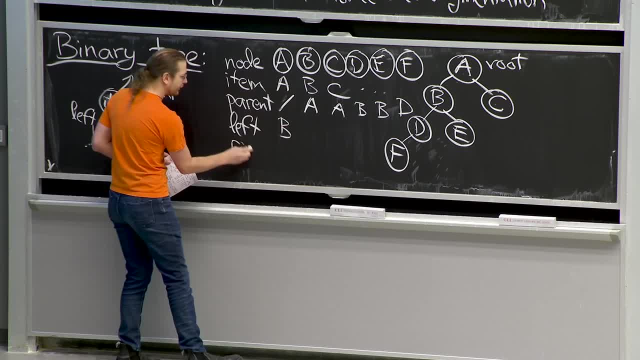 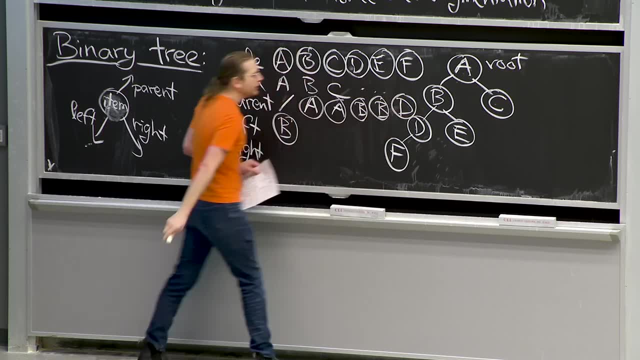 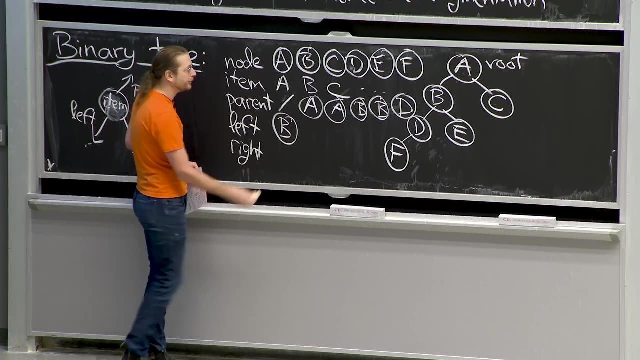 So left pointer of A is B, Right pointer of A. sorry, B the node. These should all be nodes. I'm circling for nodes and just writing the letter for the item to make it clear that those are different things. The right pointer for A is C, Left pointer for B. 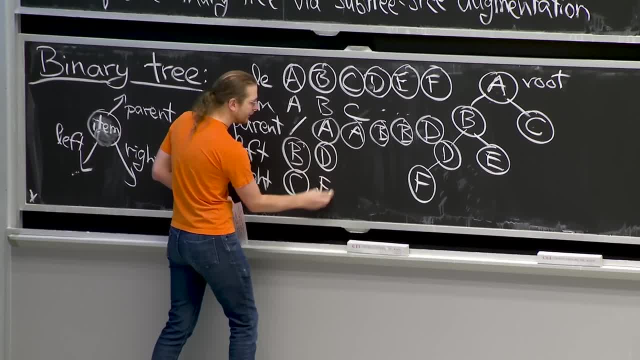 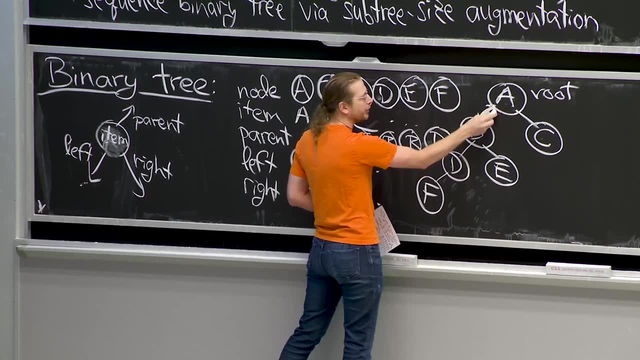 is D. Right pointer for B is E, and so on. So, in other words, each of these lines is a bi-directional pointer. In this direction, it's the parent direction. In this direction, it's left, in this case. 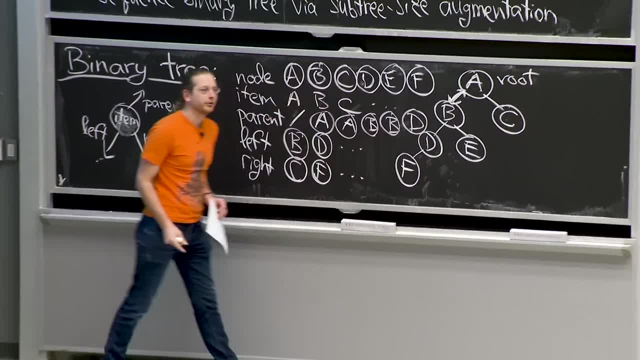 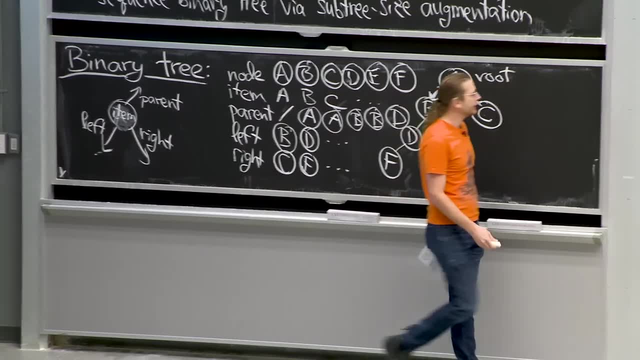 Because it's bi-directional. we don't draw the arrows, We just draw undirected lines. This is, in general, what a binary tree looks like. A key invariant is that if you take a node and say, go to it. 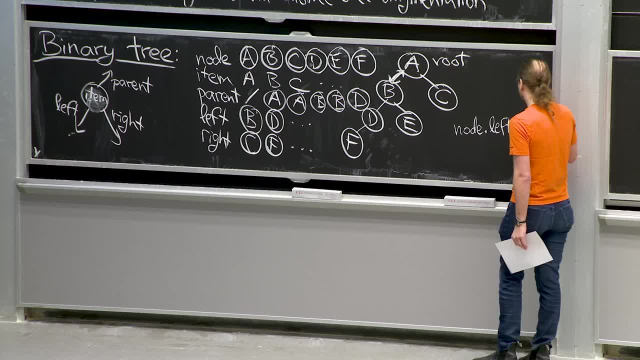 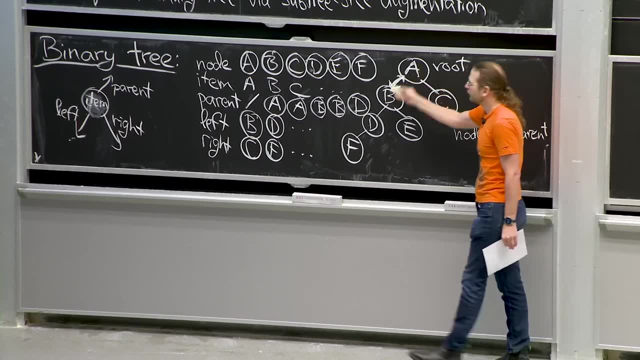 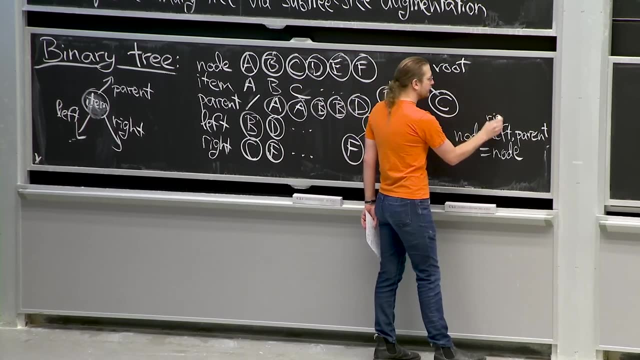 It's left pointer left child- And then go to that node's parent. This should be the same as node, So that's just saying parent is always the inverse of a left or right operation. This is also true for right, And that's a binary tree. 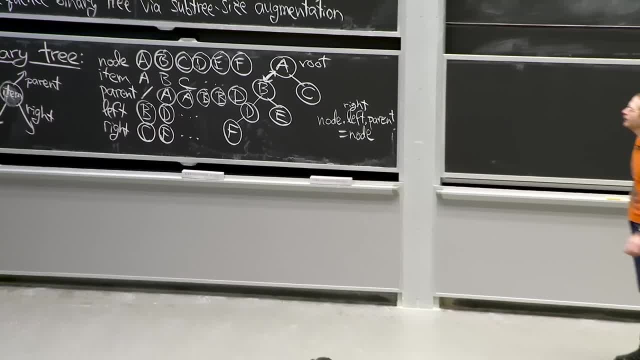 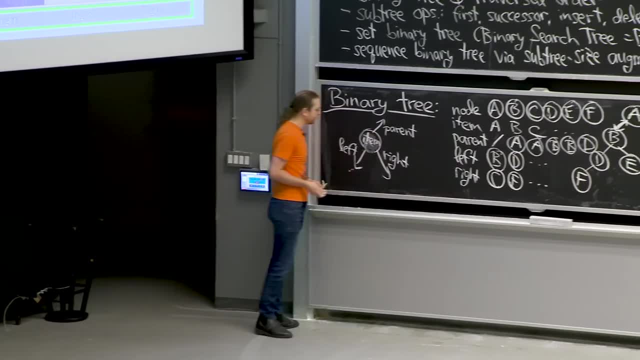 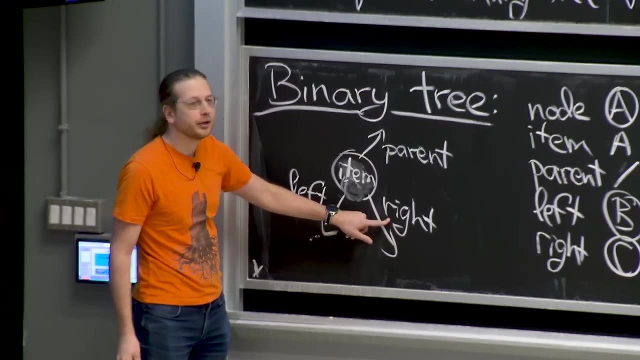 Now, the intuition of what's going on here is, you could say, we're inspired by a linked list. Linked list had a very similar structure, Maybe an item, or there's a node. it had an item in it And it had a next pointer. 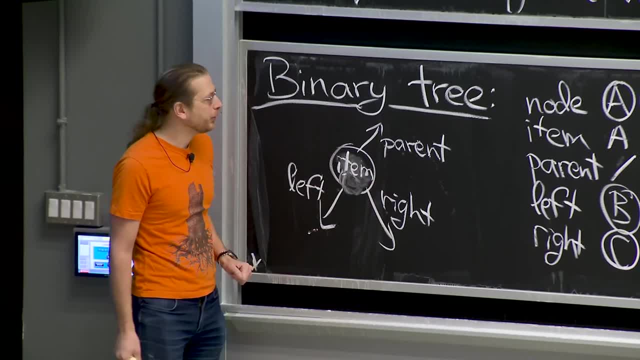 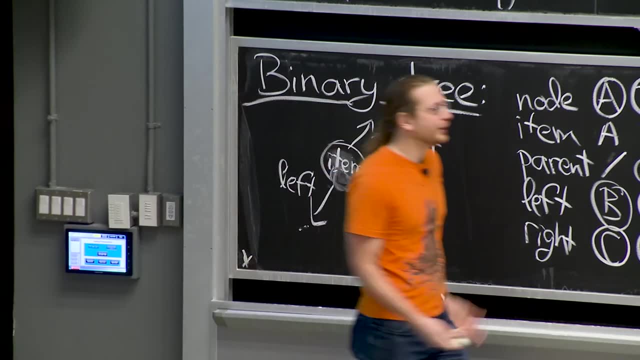 And it had a previous pointer. So in some sense, if it's doubly linked, we had a previous pointer. If it was singly linked, we only had a next pointer. And if you think about the limits of linked lists, especially singly linked lists, if you just 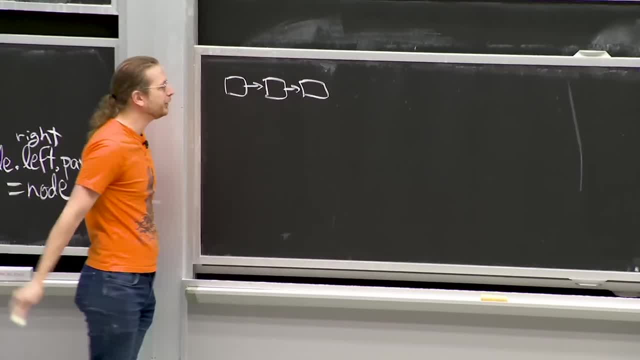 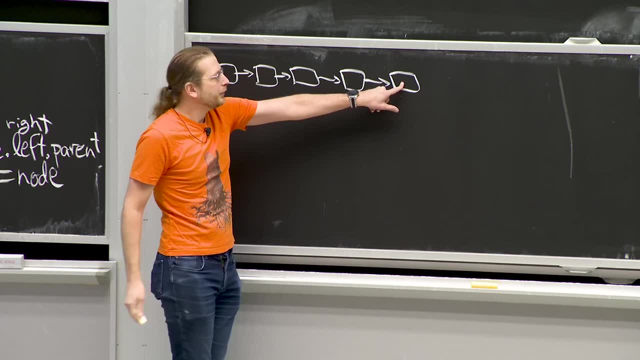 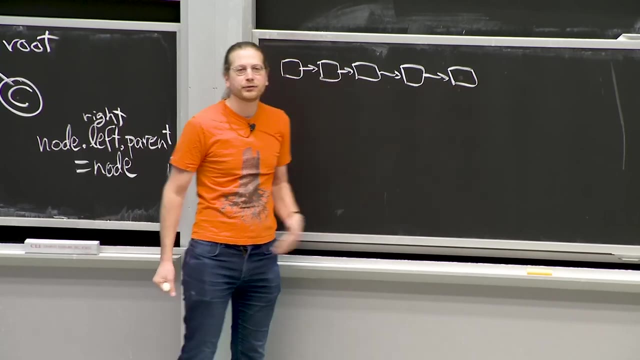 have one pointer per node. you can only build a list, And so the result is: You know this node is going to have depth. linear Depth means how many pointers do I have to follow to get here From the root of the structure, which for linked lists? 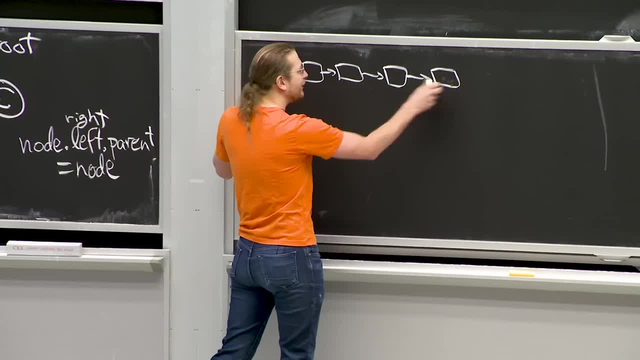 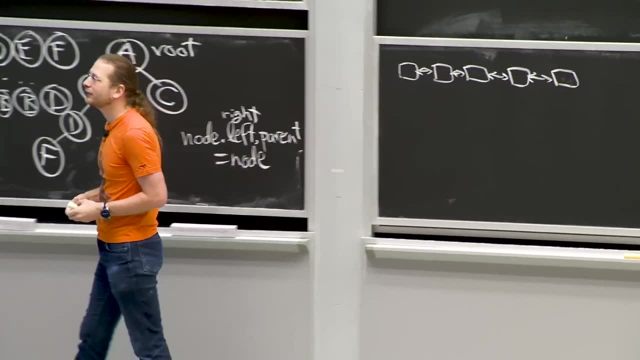 was the head was doubly linked. OK, I can have a head and a tail And I can put bidirections on here, But then still the middle item has depth- linear. So there's no way to get there in less than linear time. 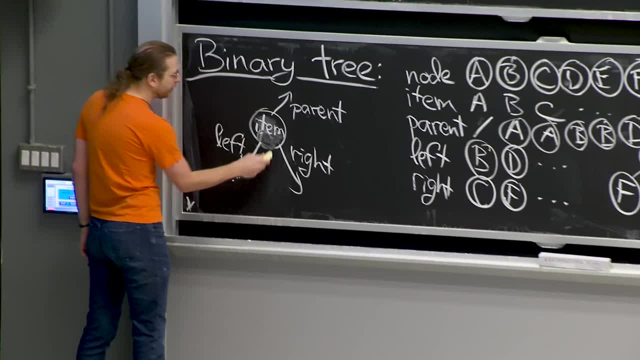 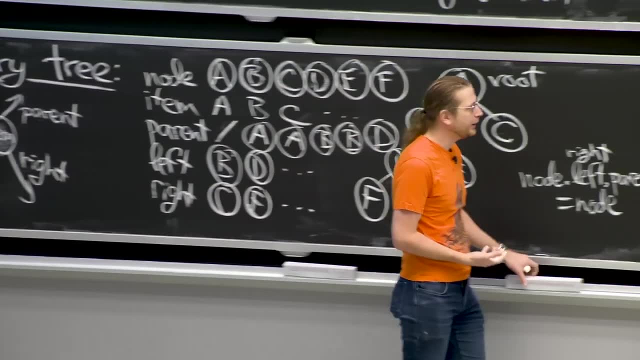 With binary trees because we use two types of next pointers: left and right. Right, We can build a tree And we know trees in general have logarithmic, can have logarithmic height, And so it's possible in a tree to get to any node starting. 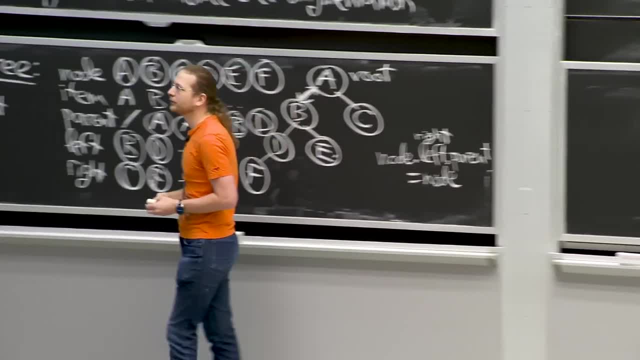 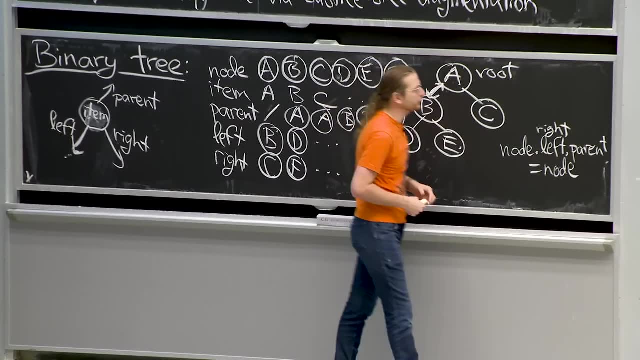 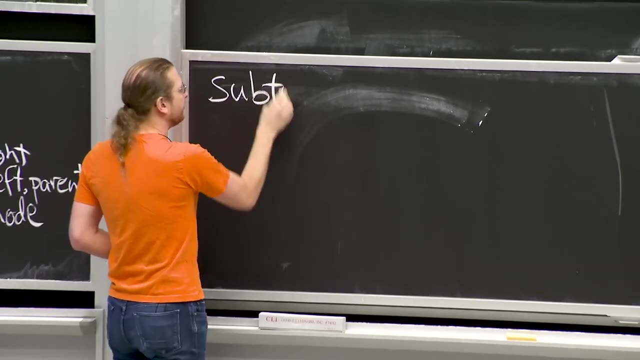 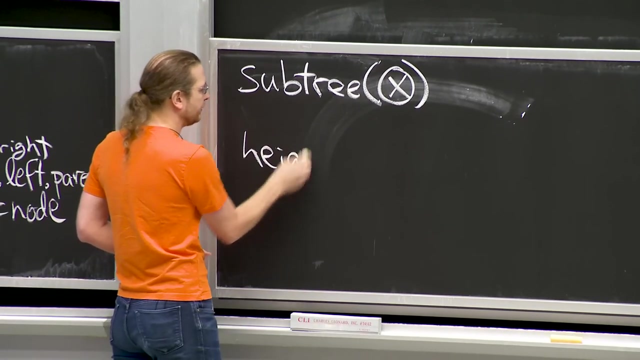 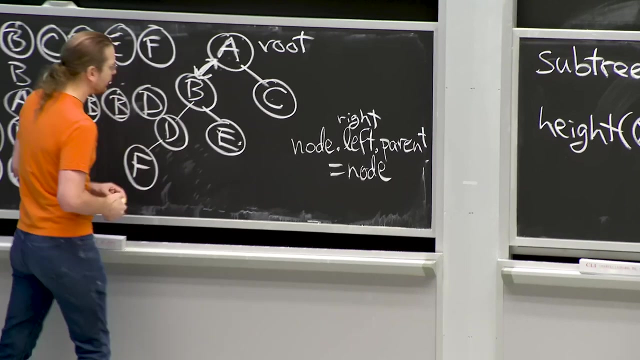 from the root in only log n traversals. So that's the intuition of what's going on Now. today we're going to talk about the height of a tree. So let me define a couple of definitions here: Subtree and height of a node. so a tree decomposes into subtrees. 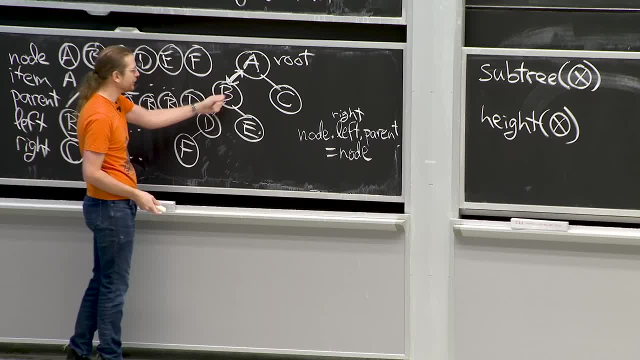 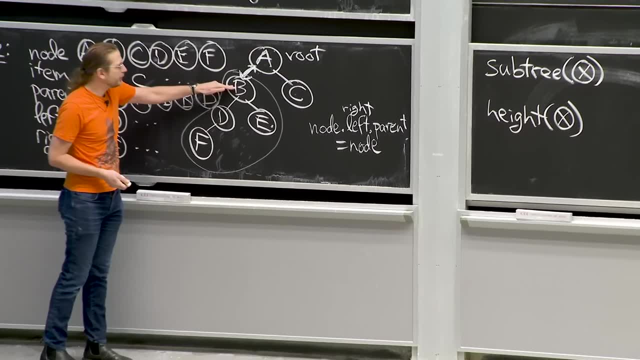 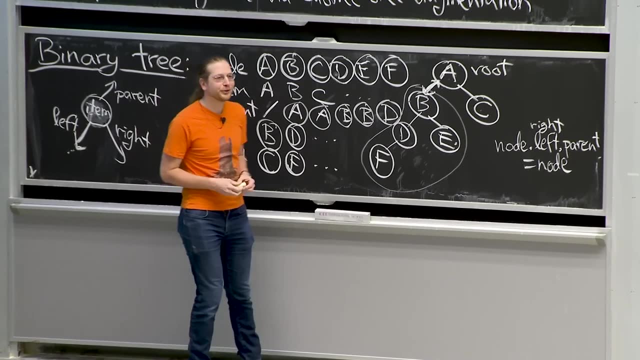 So, for example, the subtree rooted at b or the subtree of b is this portion of the tree, So it's that node and all of the descendants of this node. So because we have parents And children, we can generalize in the familial tree sense. 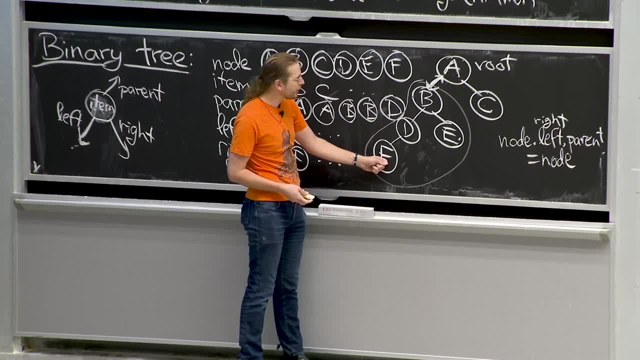 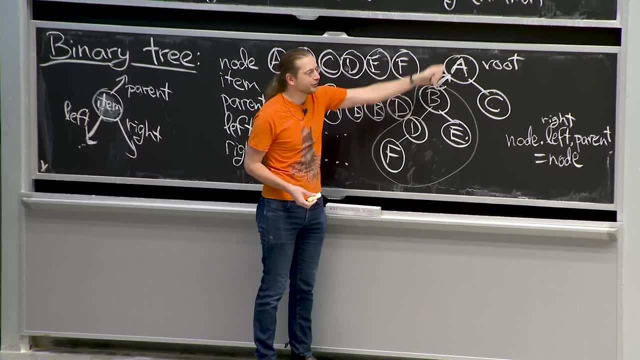 We can talk about ancestors of a node. So the ancestors of f are its parent, its grandparent, its great grandparents and so on. Together all of these are called ancestors. It doesn't quite correspond to familiar trees because familial trees- you have two parents. 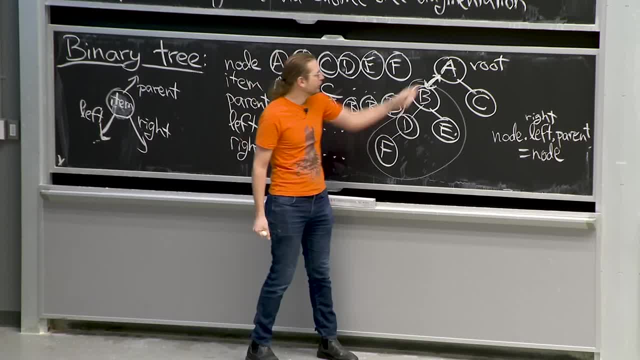 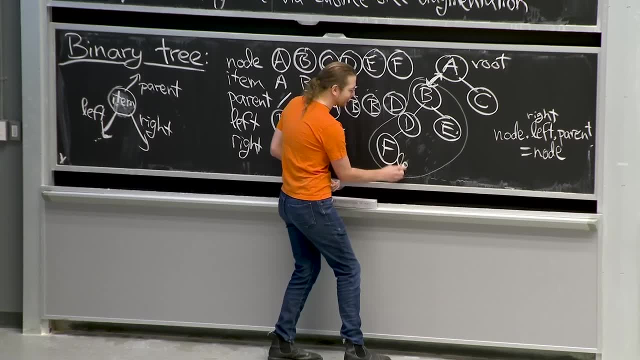 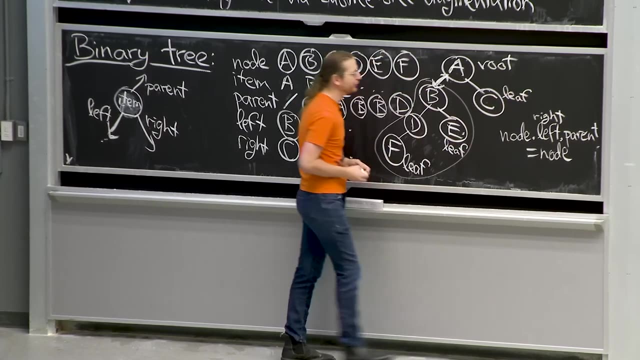 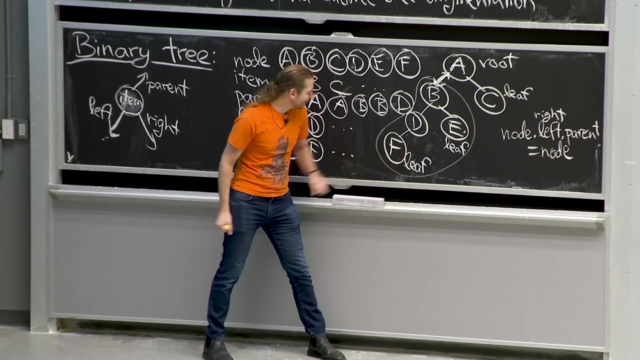 Here you only have a unique parent, Or the poor root has no parent. We also talk about- This is like mixed metaphors- Leaves of the tree. these are people with no children. Parents will complain about this, Like many of us in this room. we have no children yet. 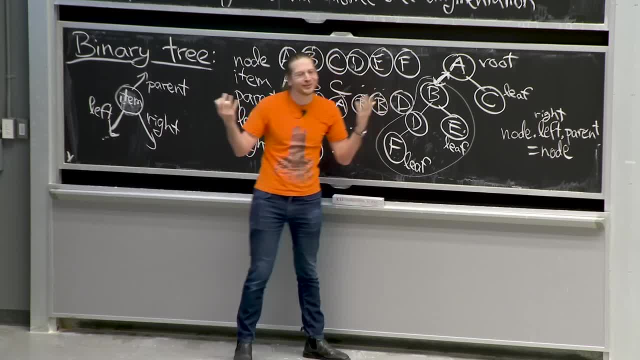 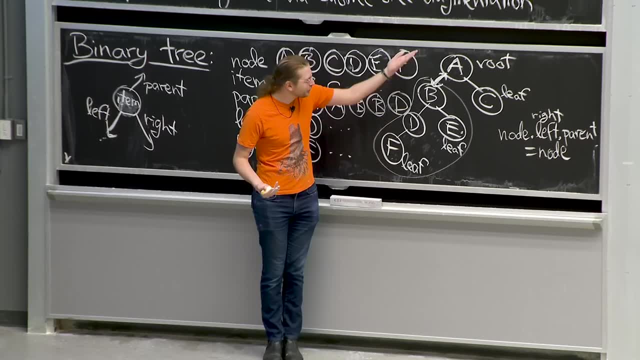 so we were called leaves. You can tell your parent, hey, I'm just a leaf, you know, blown in the wind. It's so many mixed metaphors, but we always draw trees downwards, like the root structure of a tree. 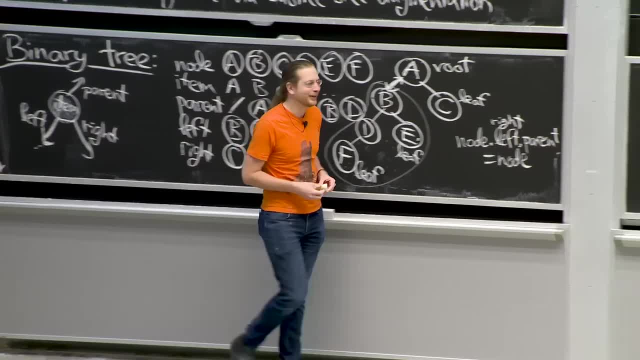 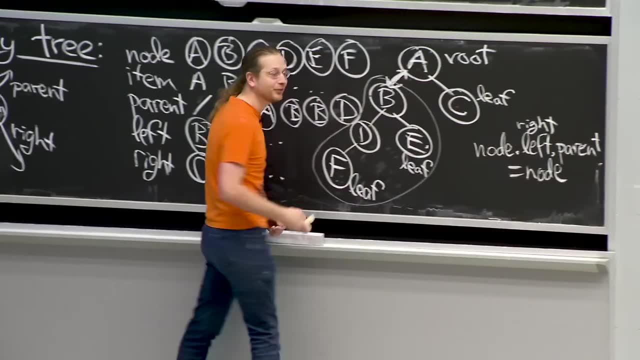 yet we call the ends of the roots leaves, which is upside down. Anyway, that's trees for you. Lots of entertaining analogies. OK, but ancestors are useful, Descendants are also useful. So the descendants of B are all of its children. 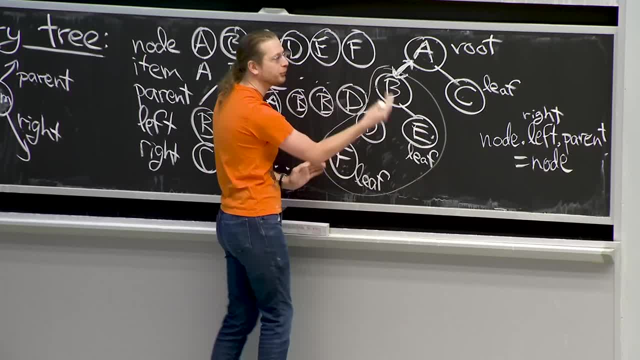 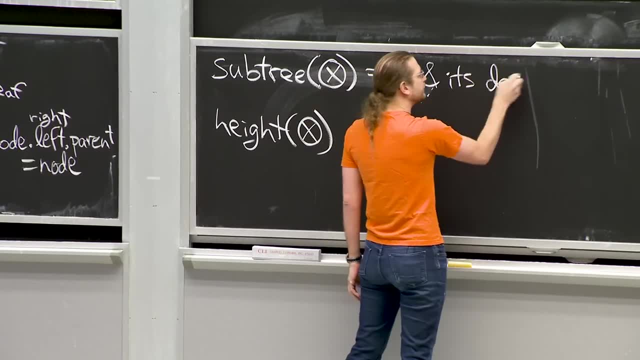 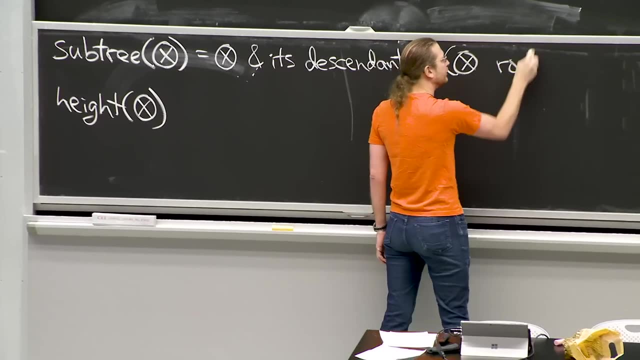 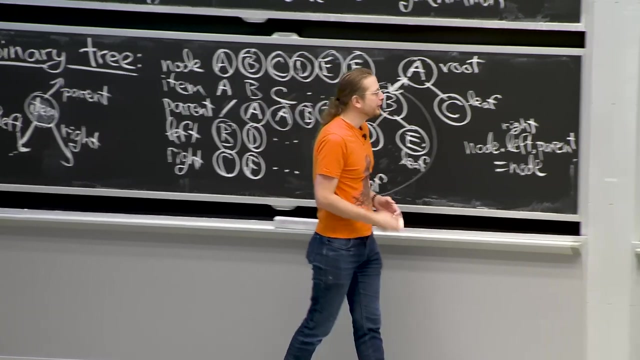 and all of its grandchildren and all the way down but just within the subtree. So subtree of x consists of x and its descendants and we think of x being the root of that subtree. So we're kind of forgetting about everything outside of the subtree when we talk about subtree of x. 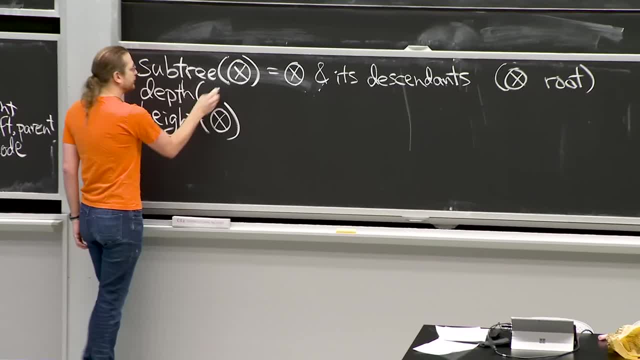 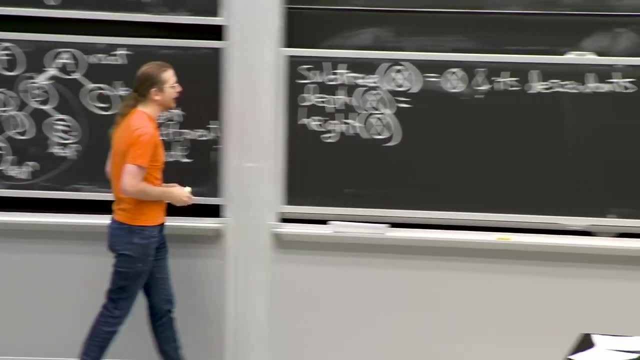 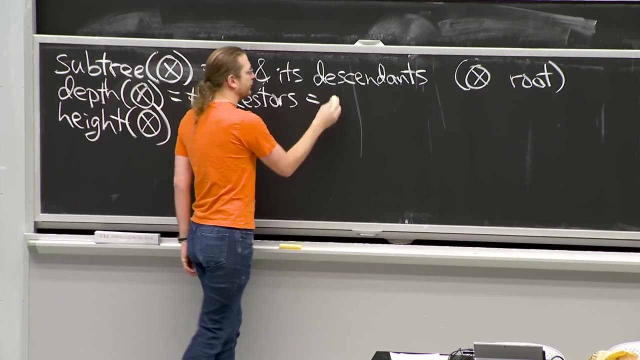 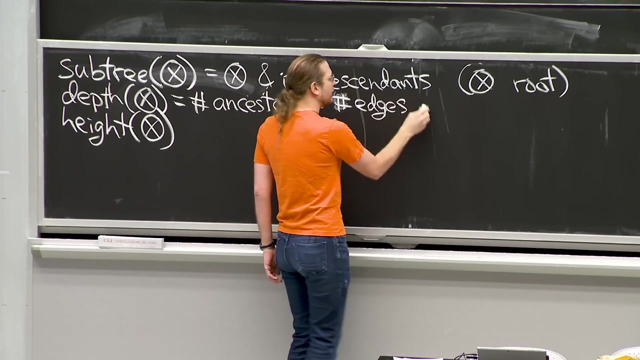 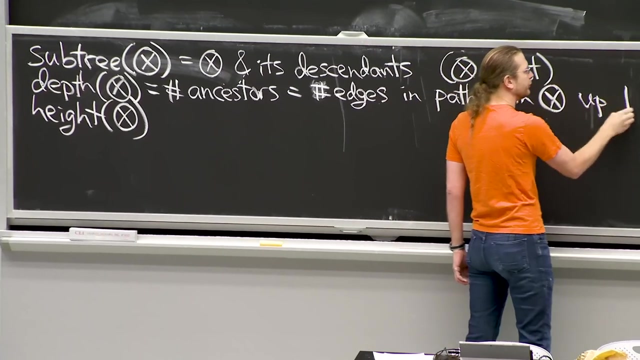 Let's talk about the depth of a node. Depth of the node is, I guess, the depth of a node. I guess the number of its ancestors. that's right, But the way I usually think of it is the number of edges and the path from x up to the root. 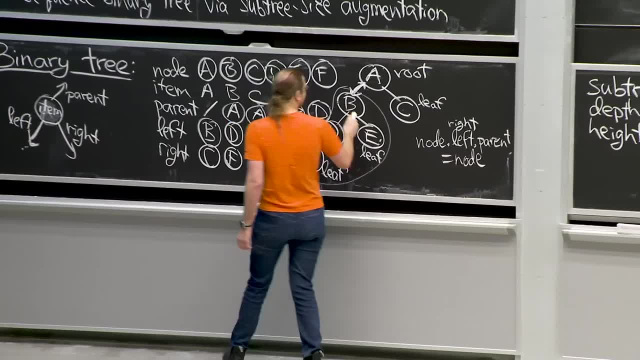 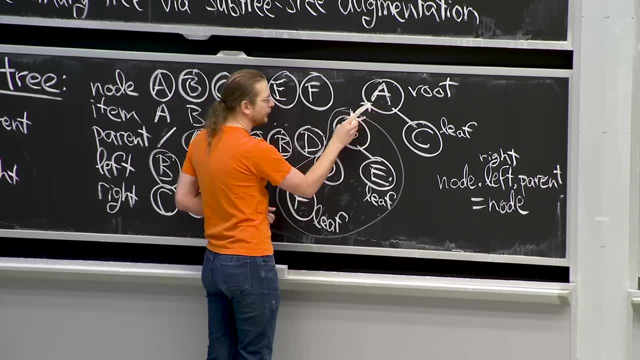 So every node has a unique path that goes upwards. until it can't go up, It can't go up anymore. So the depth of e is 2 because there are two edges- 1, 2, in the path from the root a to e. 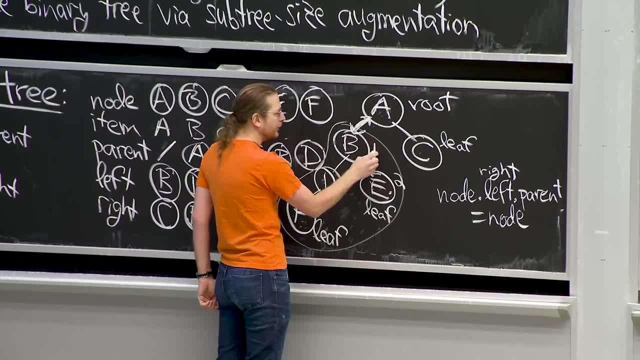 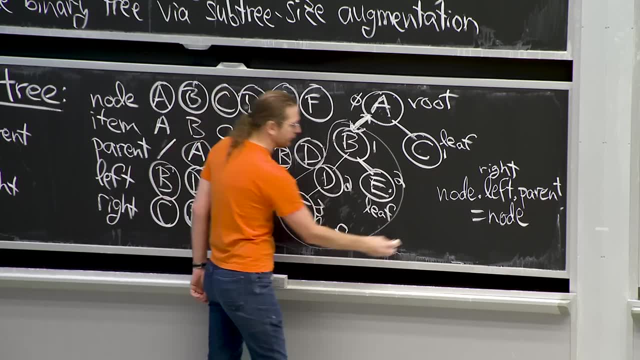 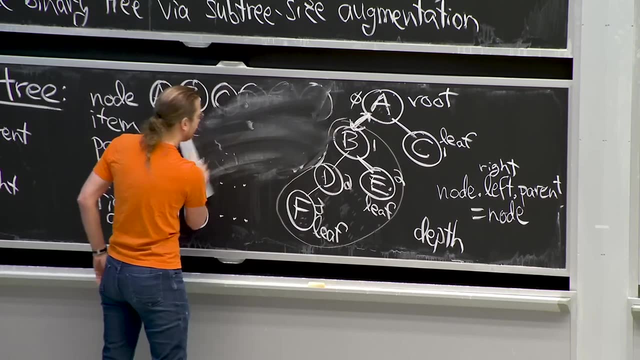 So maybe I'll write some depths. Depth of e is 2.. Depth of these guys is 1.. Depth of the root is 0,, 2,, 3.. So those are depths. I'm going to clean this up a little bit. 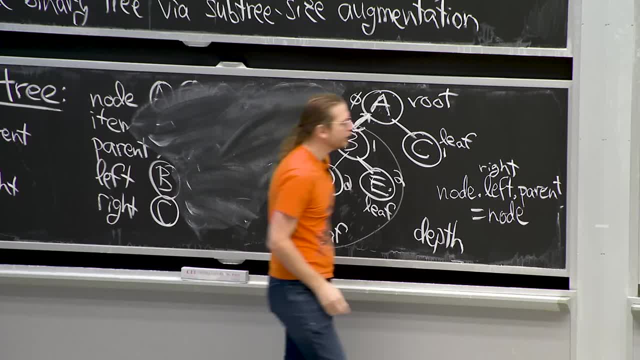 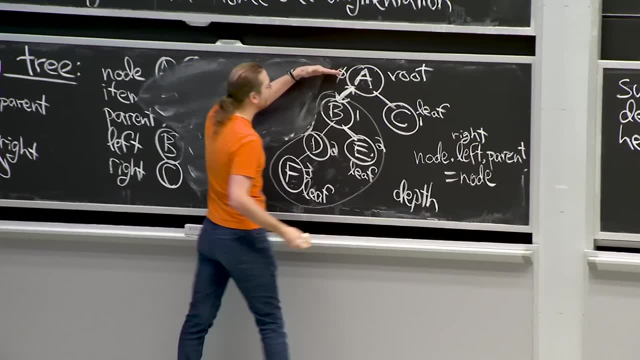 So I can focus on the image. All right, height, so depth is measuring downwards, Because if you imagine depth within water, this is the surface of the water And then we measure how deep you are from the surface. Height is in the reverse direction. 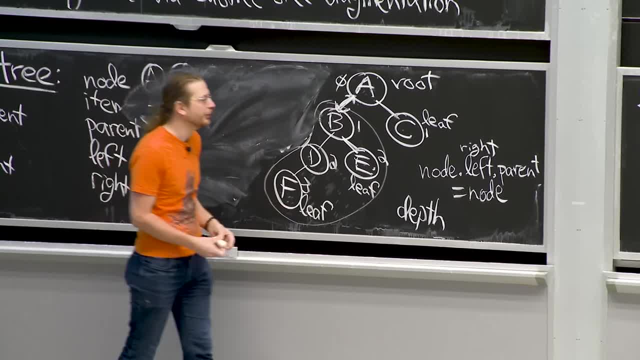 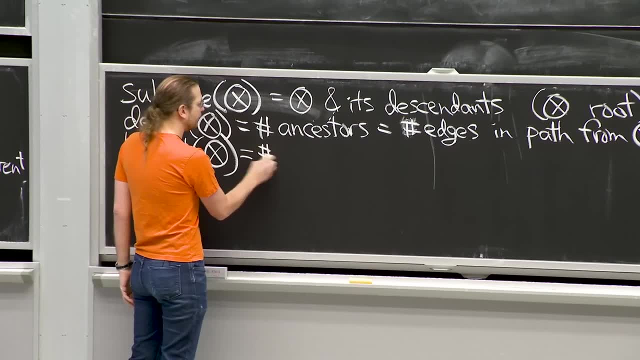 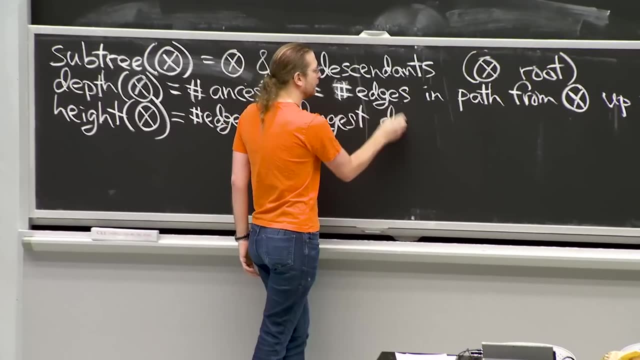 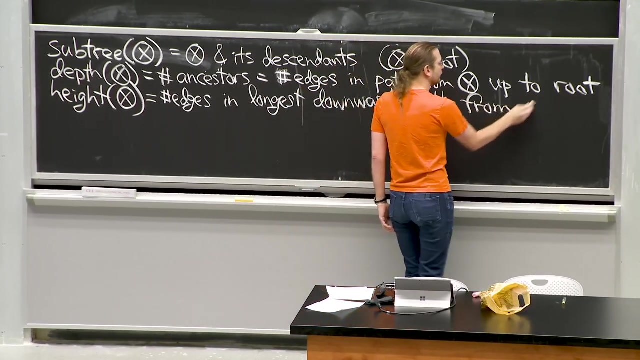 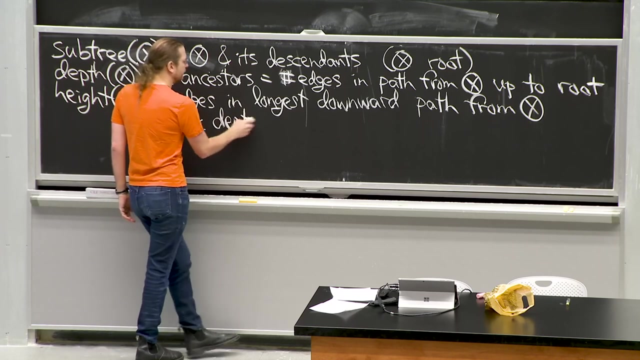 We're going to measure from the leaf level up, because leaves are the bottom of the tree. So height of a node is going to be the number of edges And the longest downward path, which is the same thing as the maximum depth of a node. 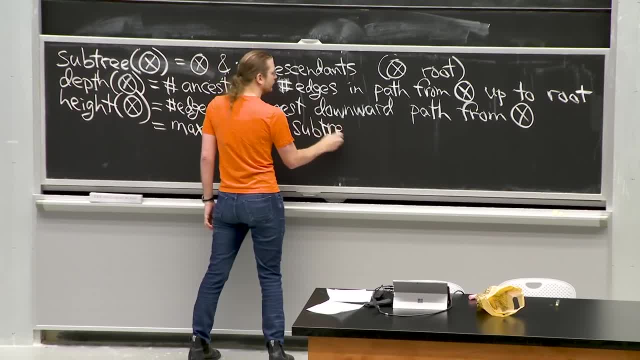 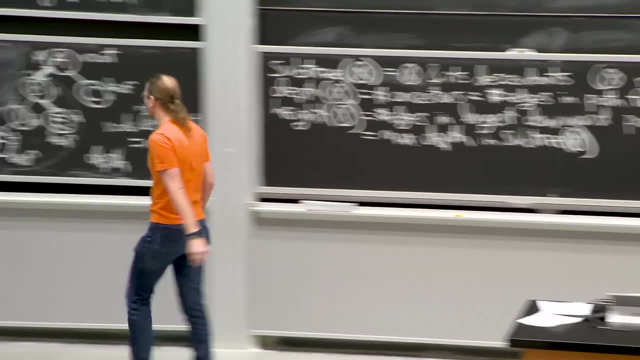 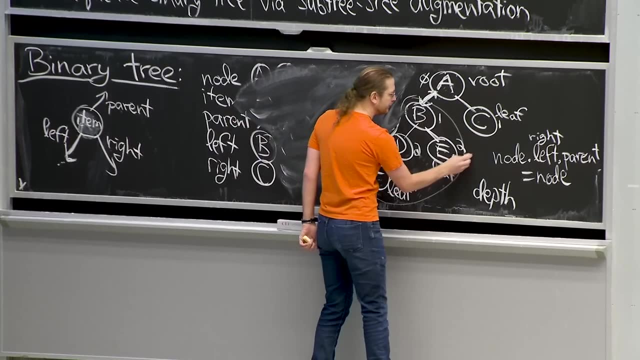 in x's subtree. Let's do height in red. So how long is the longest path from f to a leaf? Well, f is a leaf, So all leaves have depth 0.. Sorry, height 0, if I don't get it backwards. 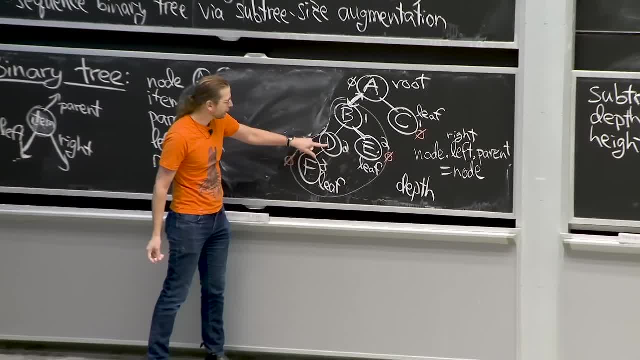 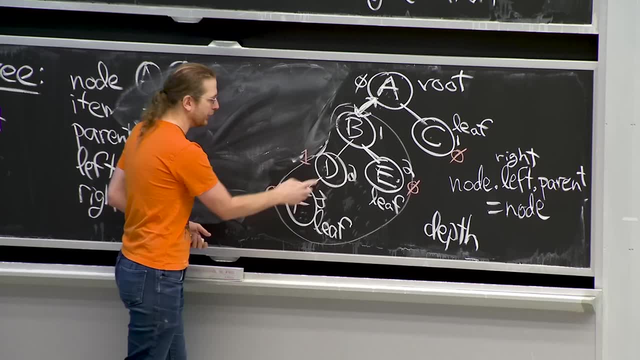 d here. so there are two ways to go down. This doesn't go to a leaf. This one goes to a leaf And its height is 0. So this height is 1.. There's one edge to a leaf here. b has two leaves it can get to. 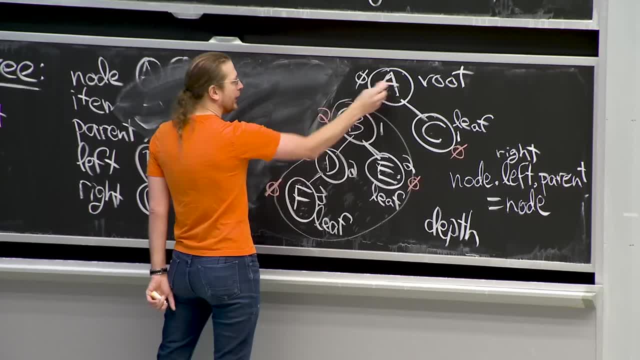 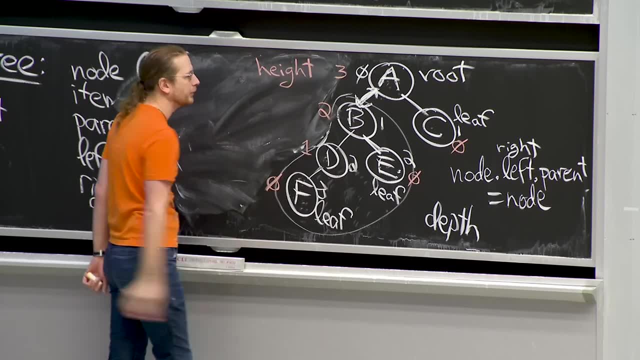 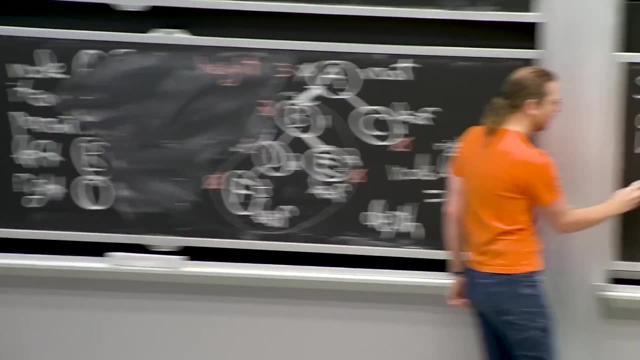 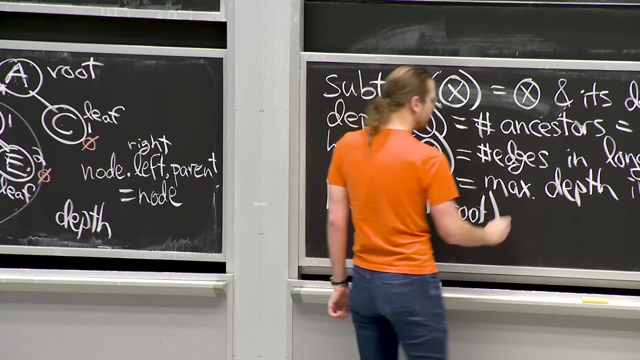 We take the longest one, So that's length. 2. a similarly has height. 3. So height we measure upward, Depth we measure downward. One thing we care about is just the height of the overall tree, which is the height of the root. 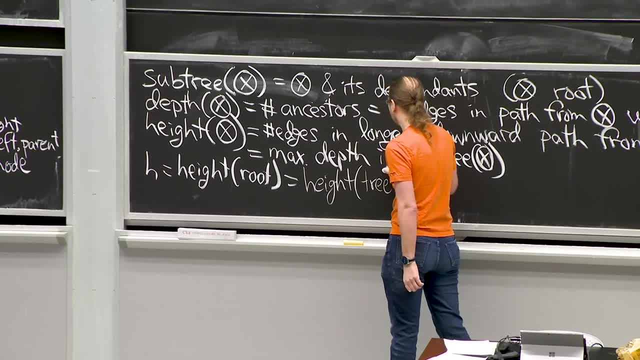 And I'm going to call that h because we're going to use it a lot And you can see how the h is going to be the same over time, over time. But it's going to be the same over time, over time. So this is going to be the height and the length of the leaf. 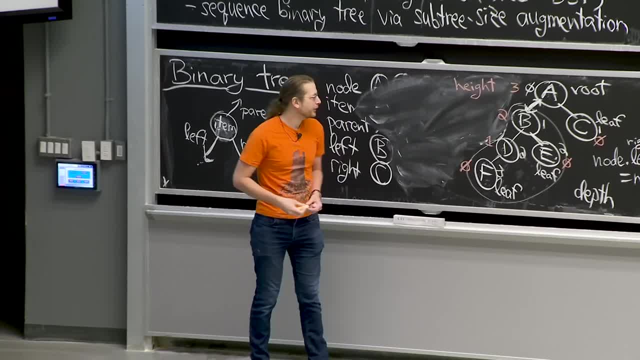 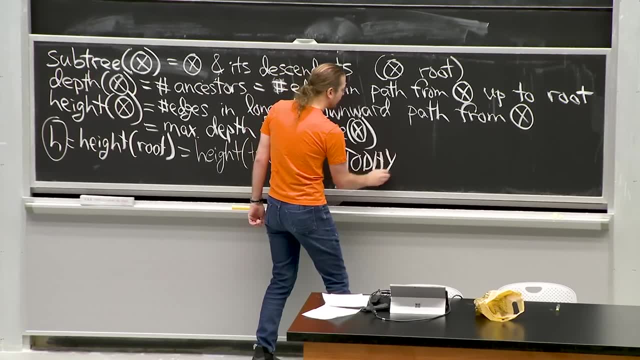 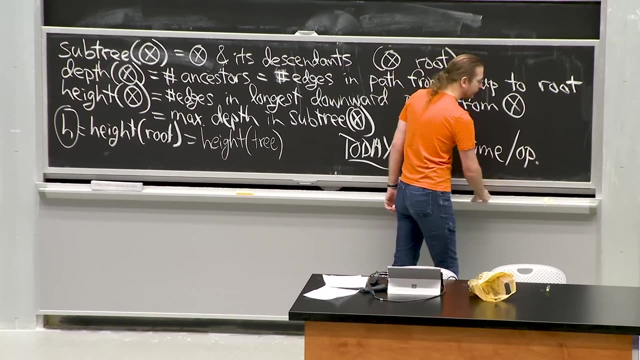 And what we're going to achieve today is all of these running times. instead of being log n, they're going to be order h. So today our goal is to get all the operations we care about in order h time, And then next lecture, we're going. 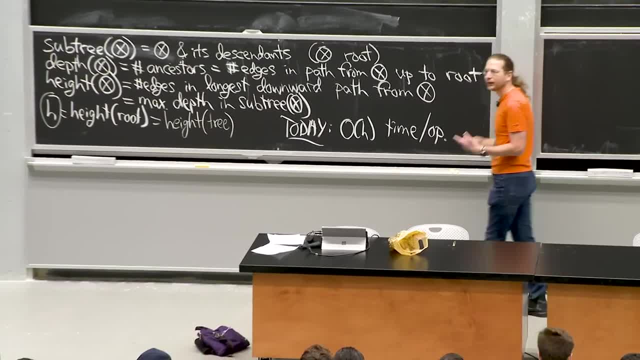 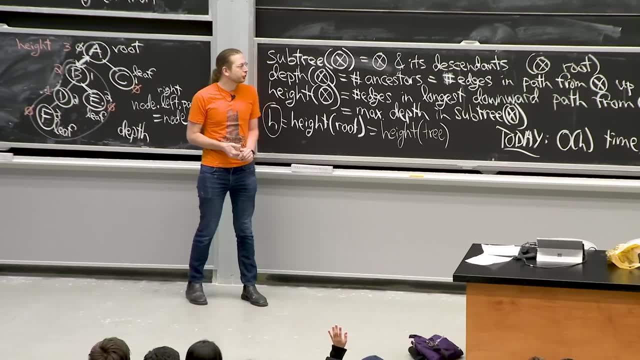 to guarantee that h is always log n and then we'll get log n time. So we need to do a bunch of work to achieve log n today. We'll do the work that's always log n- all the tree manipulation And as long as your tree is nice and shallow. 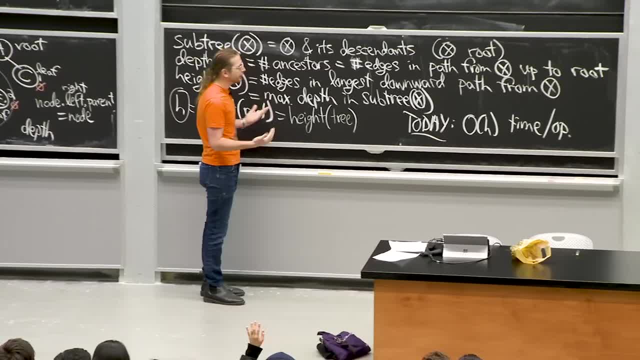 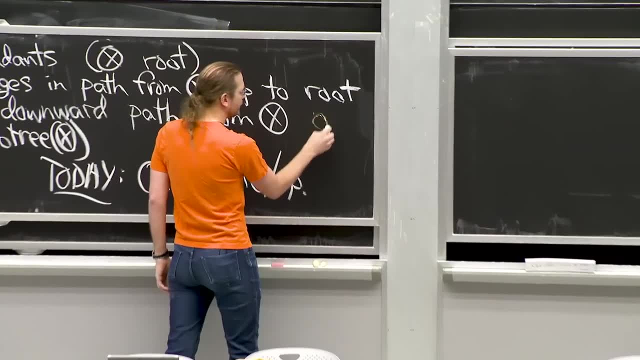 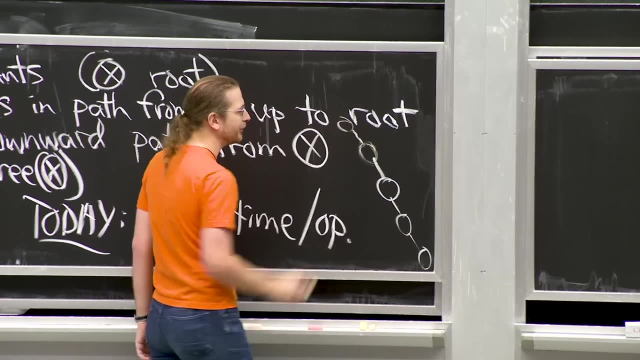 it doesn't have high height. If it has logarithmic height, everything will be log n. Of course, there are trees that are really bad. We can have a tree like this, which is basically a linked list where we only use right pointers. 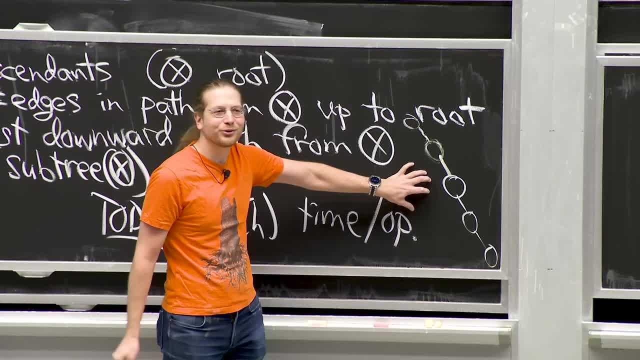 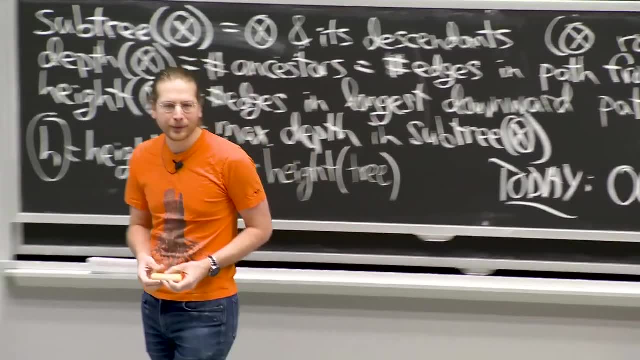 and all the left pointers are not. So there are trees that are very high, have high height. We want to avoid these, but we won't worry about that until next lecture Question. The question is: is the height of node c zero? 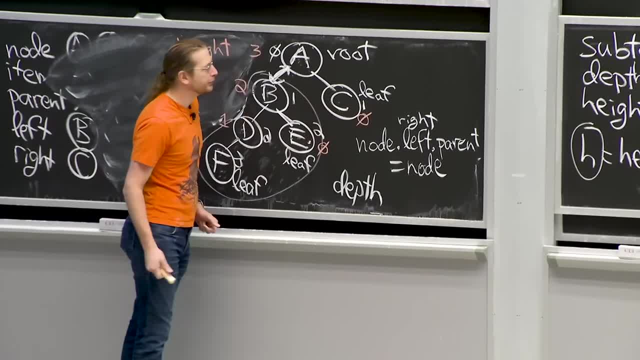 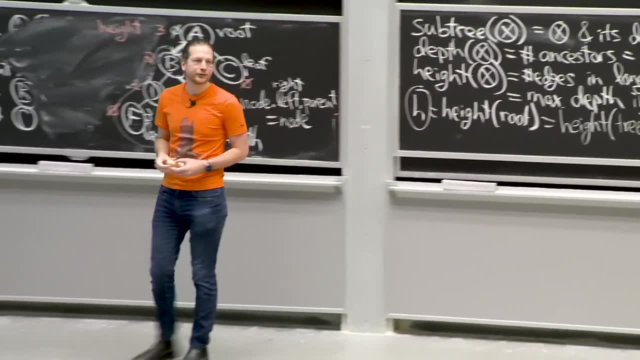 What is the height of node c? Height of node c is zero because the length of the longest path, the number of edges in the longest downward path, is zero. We're counting edges, not vertices, So the height of the tree is, of course, 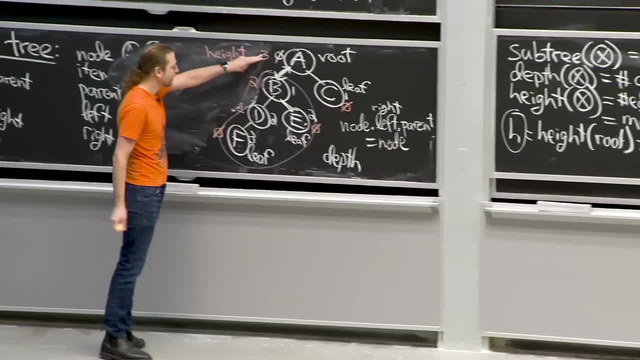 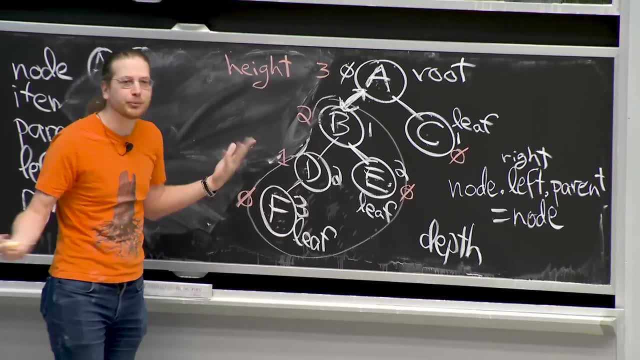 just the depth, the maximum depth. I think that's right. So the height here is 3, and the maximum depth is this terribly drawn 3.. So these happen to correspond in the maximum case, But we use height to always mean maximum. 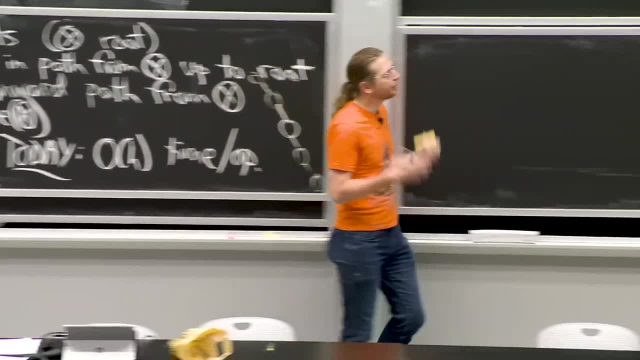 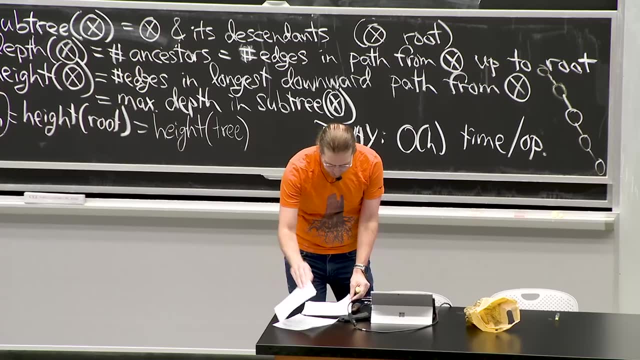 and so that's why we talk about the height of the tree. Depth of the tree is not defined, just depths of nodes. OK, How do we use these trees to represent either a sequence or a set? OK, OK, OK, OK. 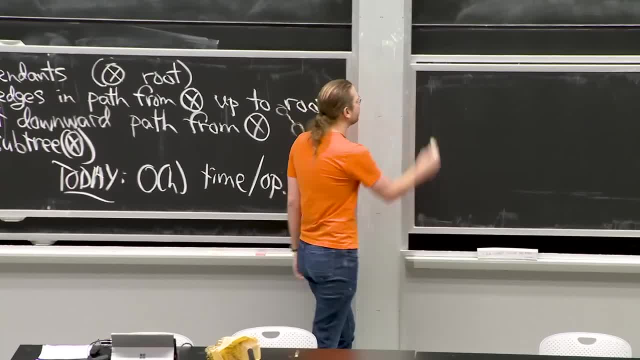 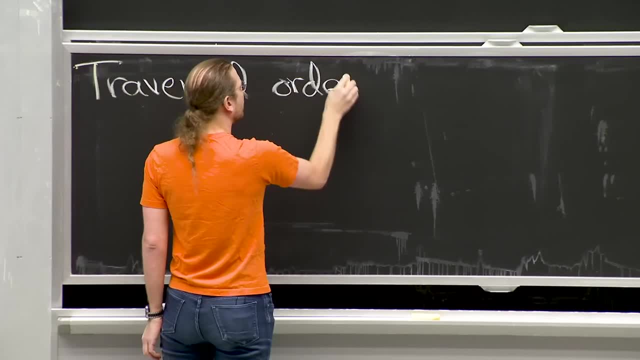 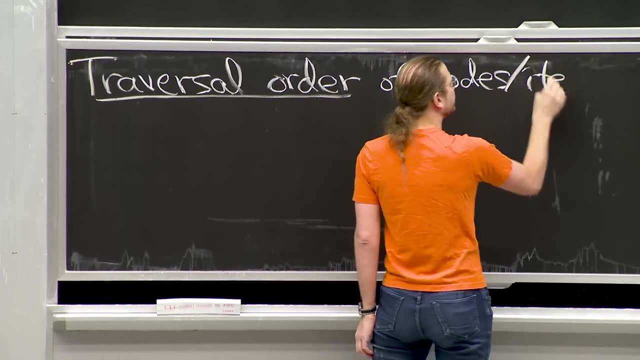 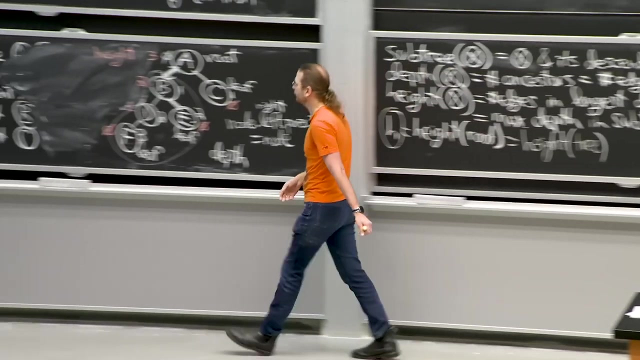 I claim that there is a natural order in trees called the traversal order of nodes or items in the tree. So I'm going to define a particular order, say in this example, Let's do the example first. Let's go ahead and do the traversal order. 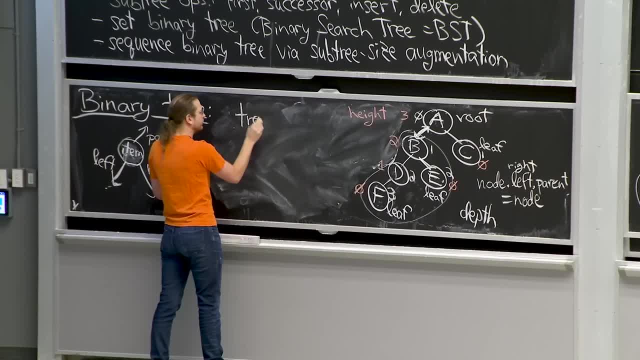 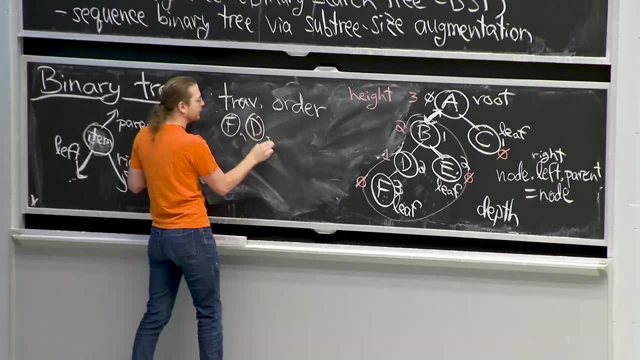 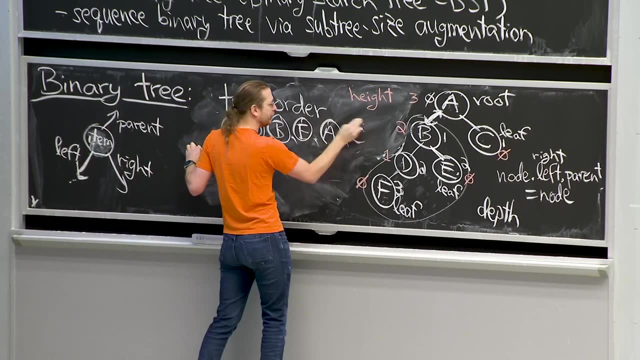 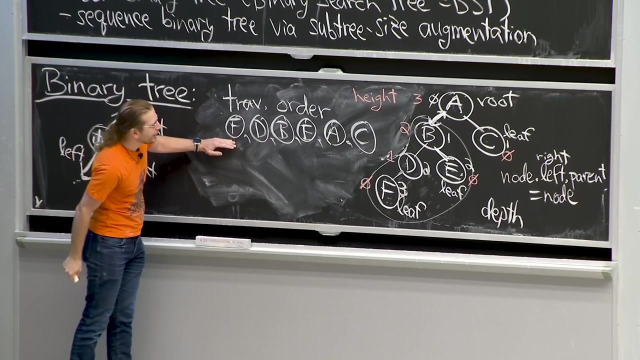 The traversal order is going to be F, D, B, E, A C. I feel like I'm in music class, This is my guitar or something, but it's not. I hope, If it is, it's a coincidence. 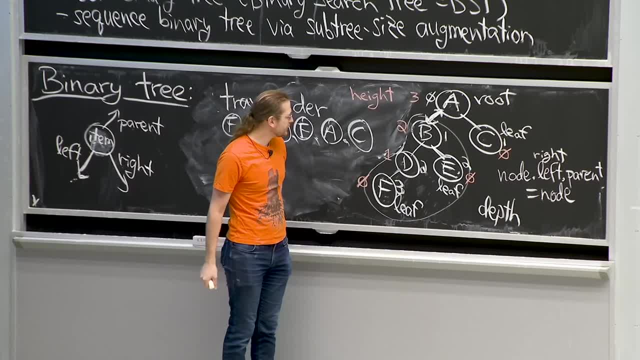 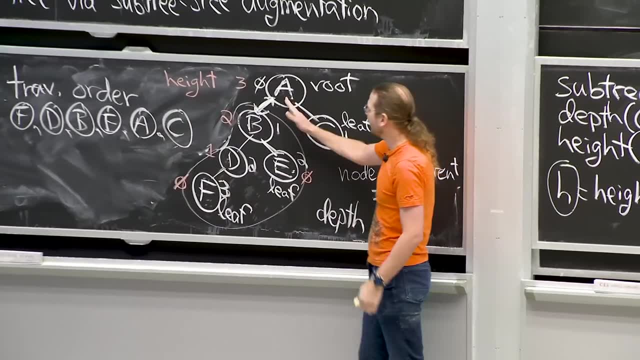 So what is this order? So what is this order? What I'd like to do is recursively define an order where the root of the tree is somewhere in the middle and everything in the left subtree is left earlier in the order than the root. 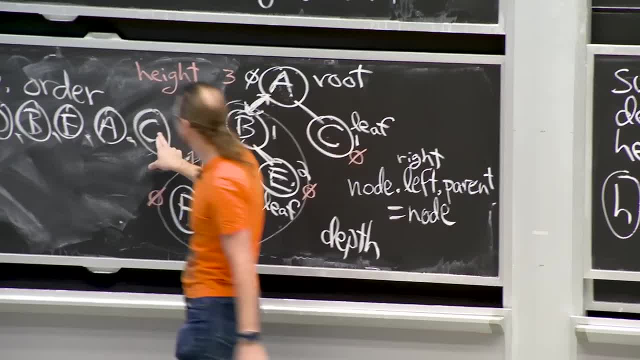 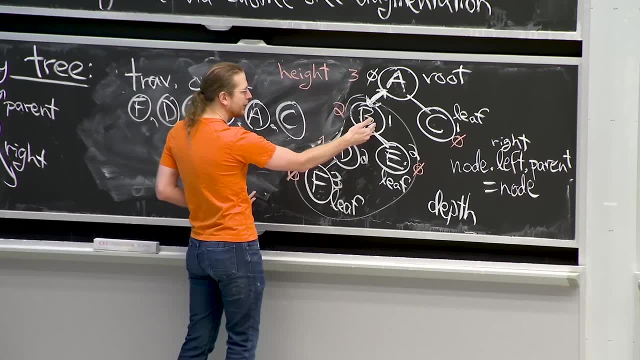 and everything in the right subtree is later. So you can see here C comes after A and then all the other nodes come before A, And recursively. if I look at a node B, this node B which appears over here, E is to the right of it. 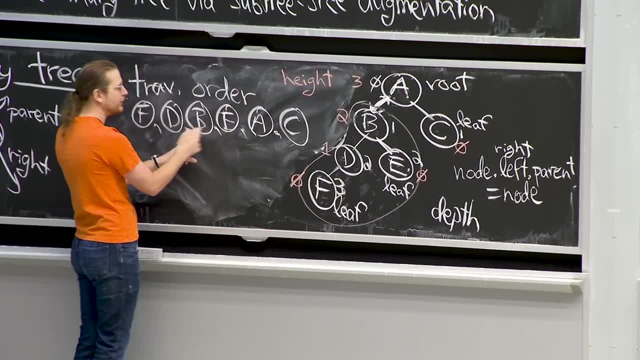 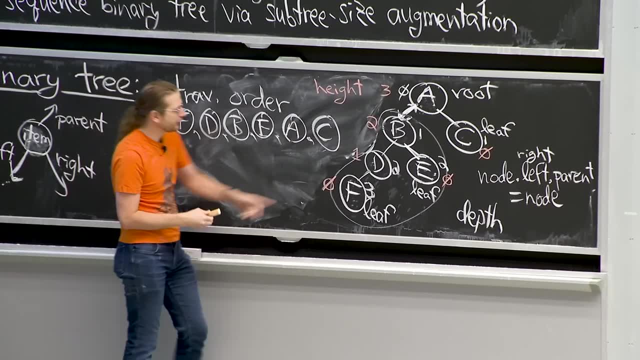 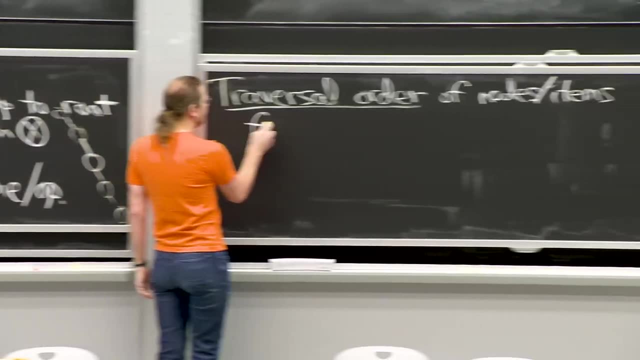 but this is all to the left of A, So E is between B and A, B on the left, and then F and D are to the left of that And again F comes before D because F is in the left subtree of D. So we say for every node: 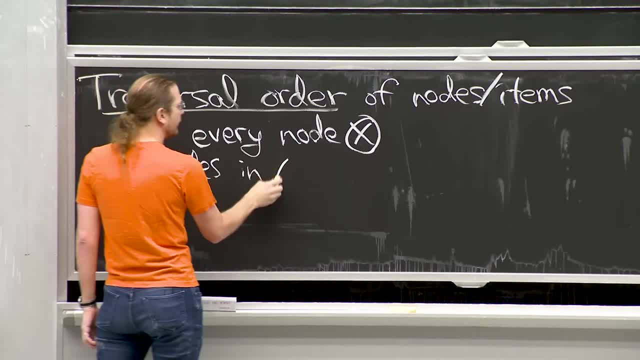 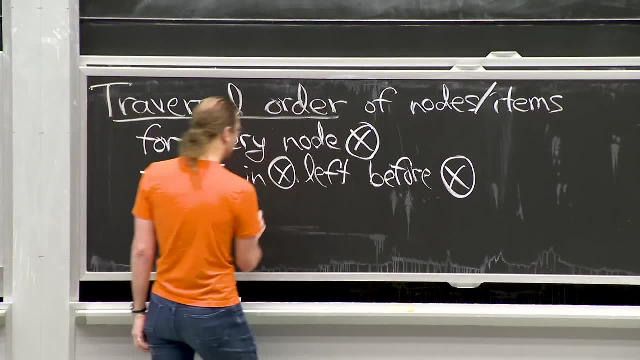 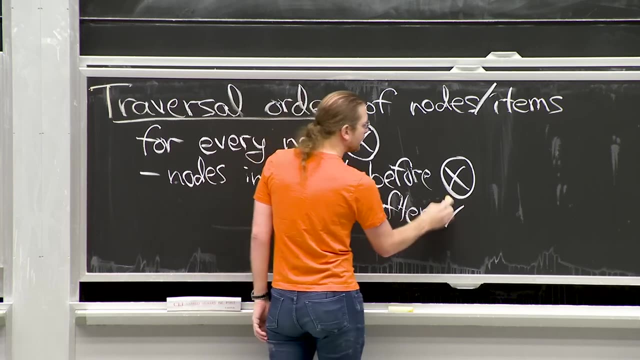 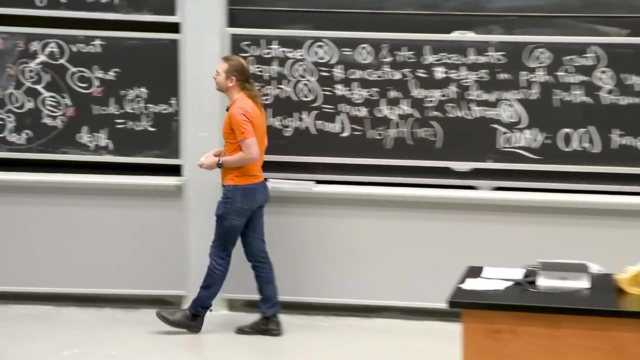 the nodes in x dot left are before x and the nodes in x dot right come after x, And this uniquely defines an order called a traversal order. It's also called the in-order traversal order. It's called in-order because it's in the traversal order. 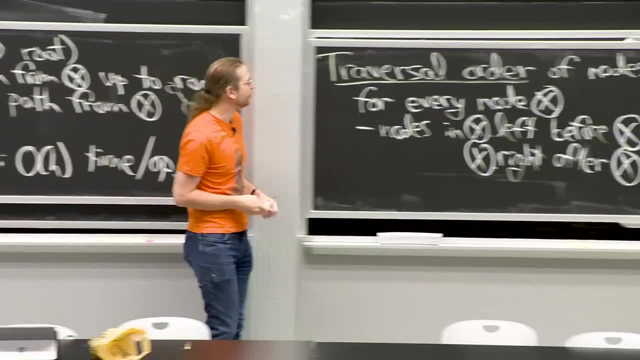 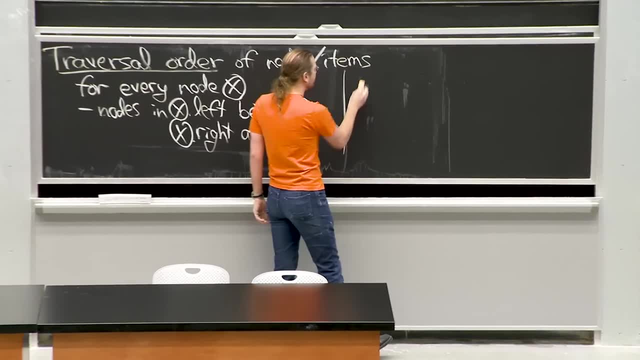 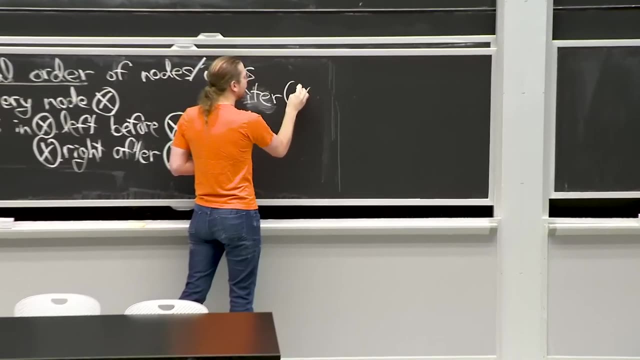 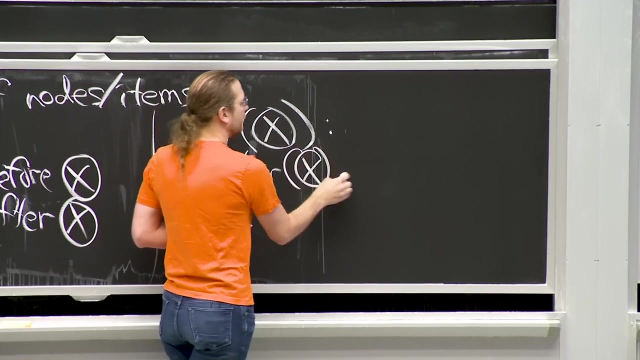 So it's very circular, but you may have seen in-order traversal. This is the same thing. There's a very simple algorithm for computing this. If I want to iterate all the nodes within a subtree x rooted by x, I just iterate on all of the nodes. 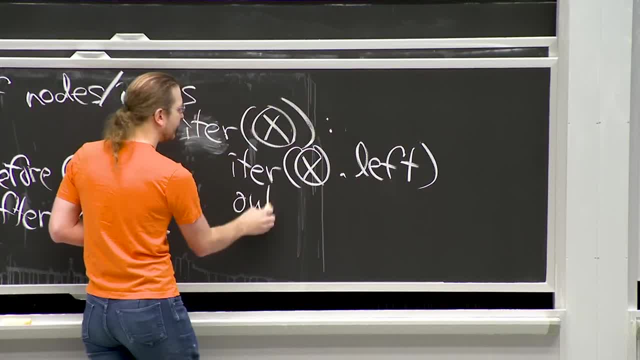 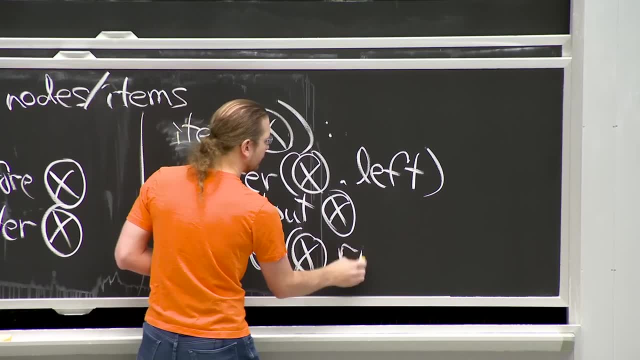 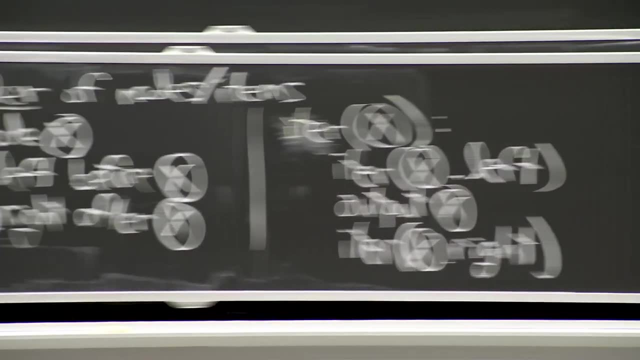 in the left subtree, Then I output x itself, Then I iterate on all the nodes in the right subtree. OK, you may have seen that algorithm before. This is just another way to codify the same thing. The result is all the nodes within a subtree. 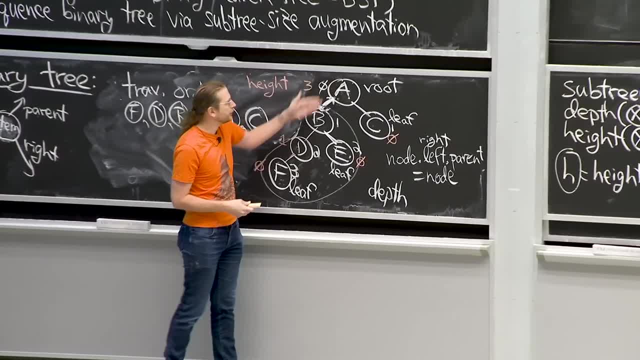 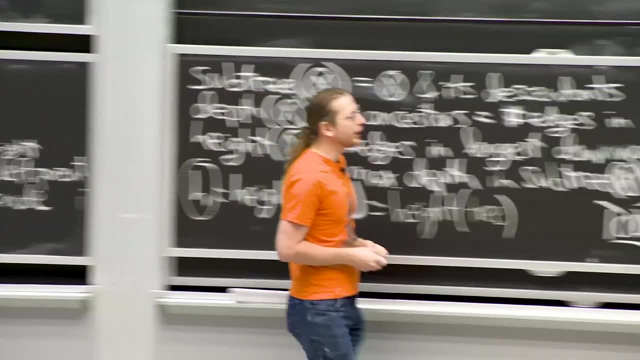 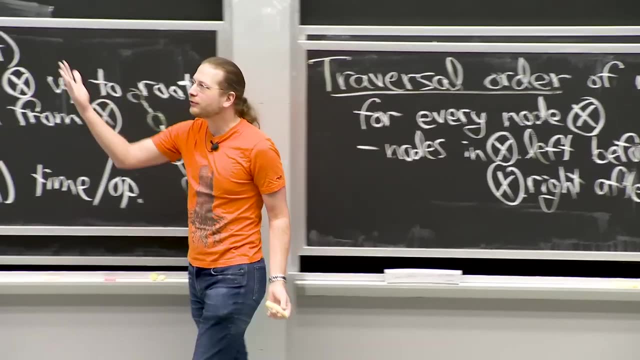 appear continuously with no interruptions, And then the parent's going to come before or after, depending on whether it's the left or right child. OK, and now it's just a matter of connecting the dots, because we're representing an order And, for sequence, that is going to be the sequence order. 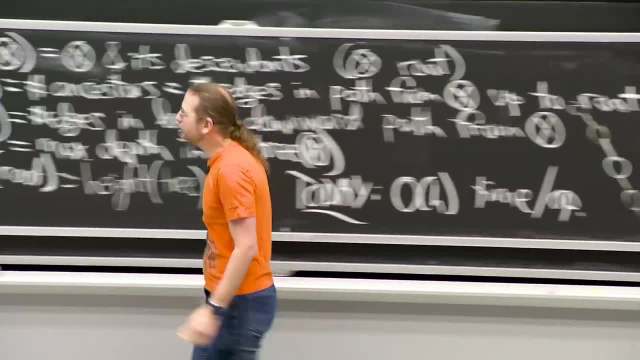 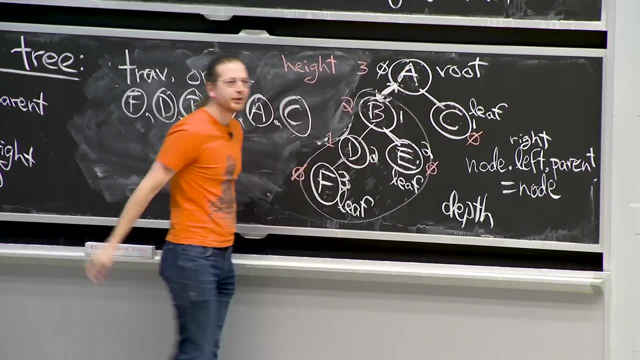 If we want to store n items x0 through x1, we're going to store x0 through x1.. If we want to store n items x0 through x1, we're going to build some kind of tree. We're going to put x0 here, x1 here, x2 here, x3 here, x4 here, x5 here. 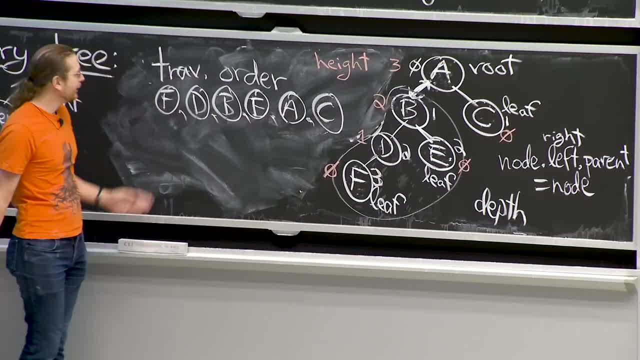 You can see, I'm very used to dealing with traversal orders. It takes a little while. You could also see it here. We're going to put x1 on this node, x2, sorry- x0 here, x1 here, x2 here and so on. 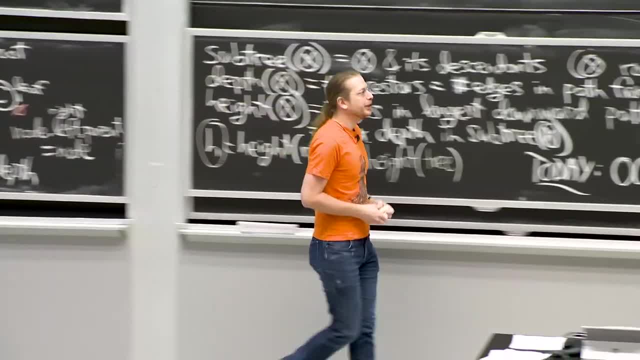 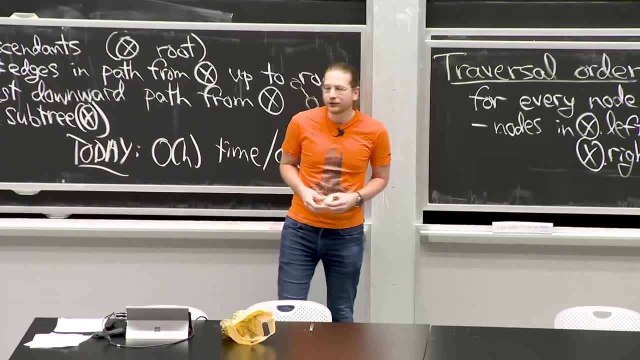 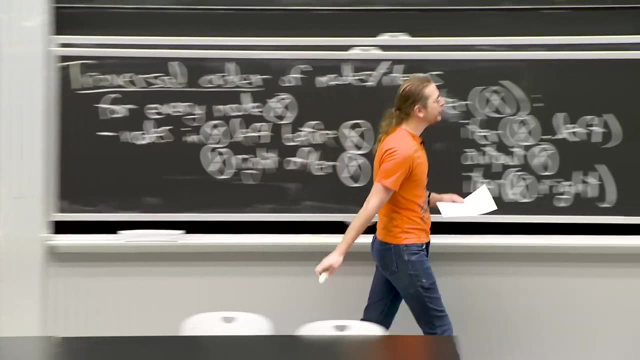 That's the same order that I gave. OK, that's for sequences, For sets. that order is just going to be the sorted order And we're going to be effectively representing the sorted order of keys, Let's say increasing. But before we get to that, let's talk about different operations. we can do just playing. 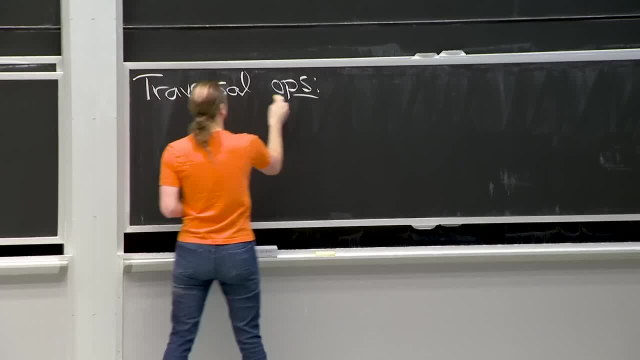 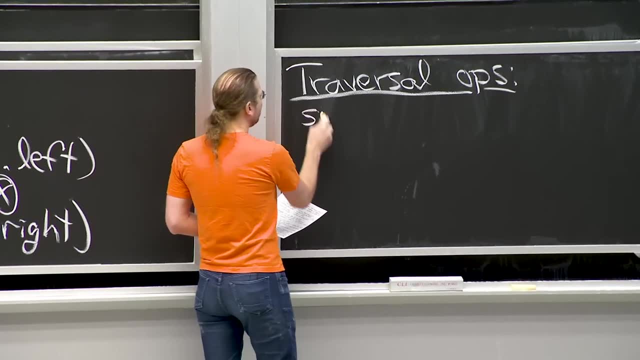 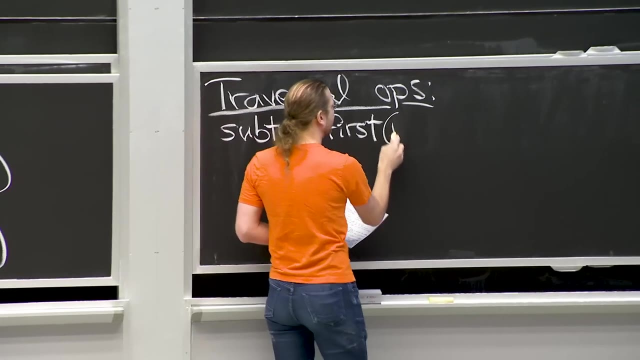 around with traversal order And we're going to use these to build the sequence and set operations that we care about. So first operation: I'll call subtree first seems appropriate, but it's called first. It's the first one, First one. 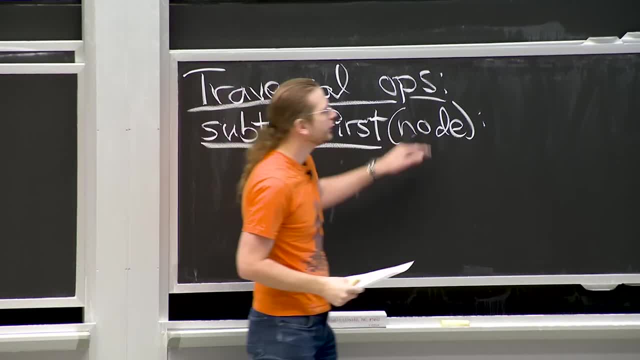 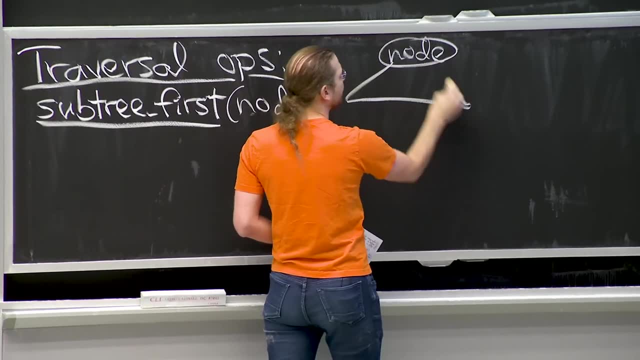 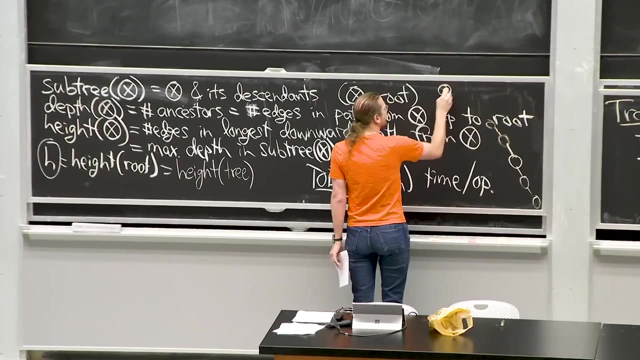 So, given a node which I'll call node, this defines a subtree which usually we draw subtrees as triangles hanging off of the node. So here I would write x, and then there's some subtree of all the descendants of x. 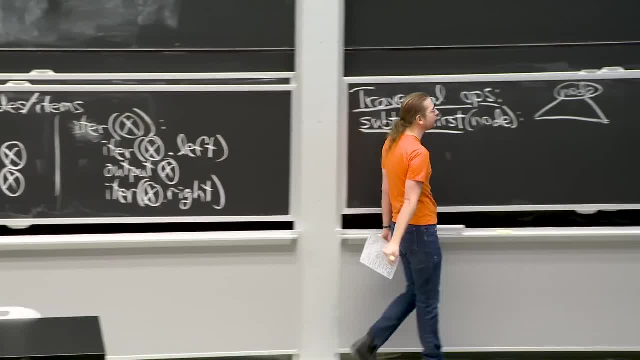 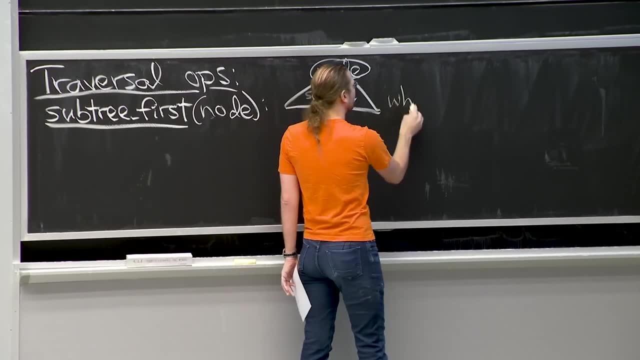 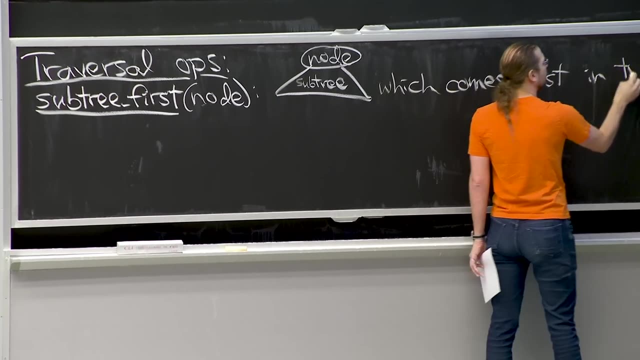 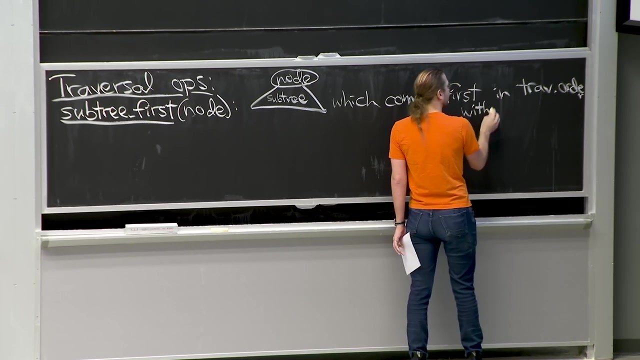 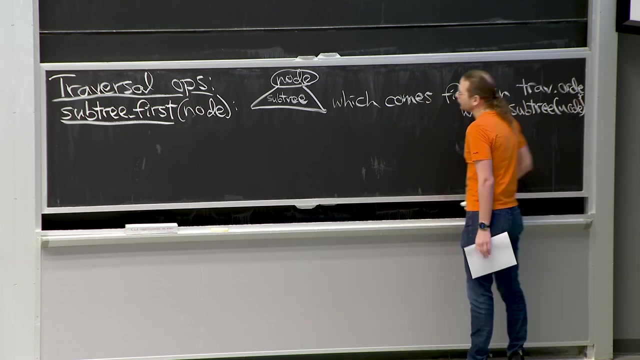 So with subtree first, I would like to say, among all the nodes in this subtree Which comes first in traversal order, So just restricting to that subtree, subtree of that. So where is it in this tree? Yeah, There's a subtree. 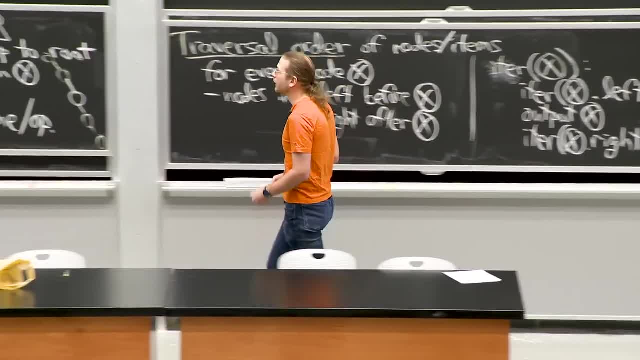 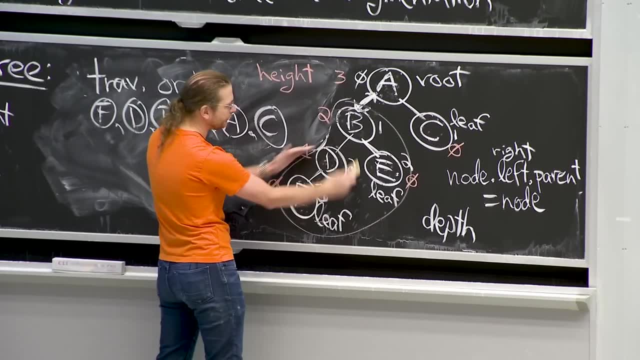 A node can only be part of one subtree. right A node is actually part of many subtrees. Good question. F is in its own in the subtree of F. F is also in the subtree of D. F is in the subtree. 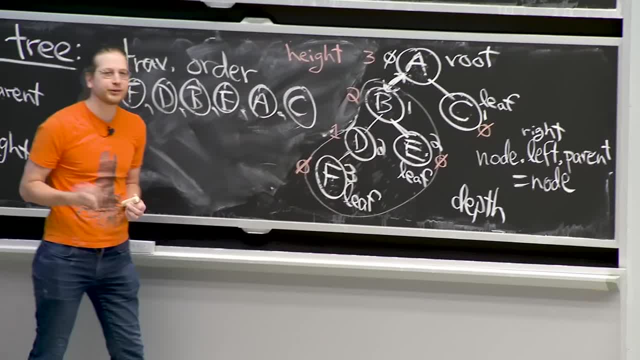 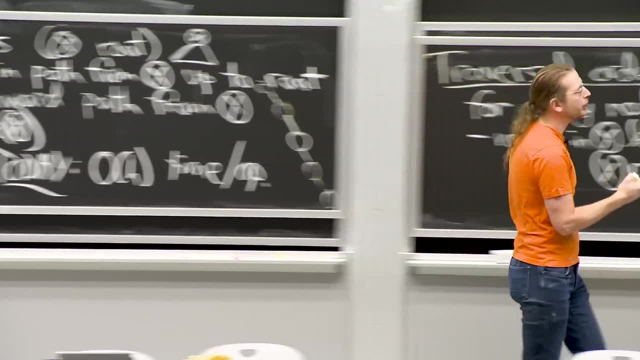 of B, like I drew. F, is in the subtree of A. It's in the subtree of exactly its ancestors. But in this operation, when we define node, our node only defines one subtree. It is the root of only one subtree. 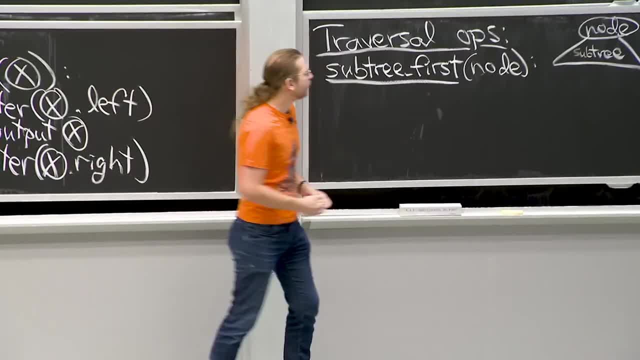 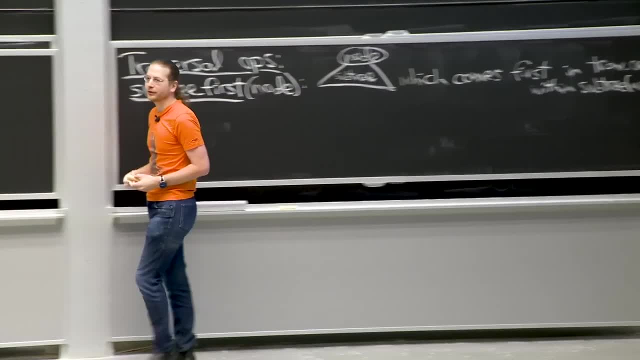 That's the subtree we're talking about. And then I want to know, among all those nodes- which includes node itself and other things- which one comes first in this traversal order. This is like practice with traversal orders, So where should I look for this node? 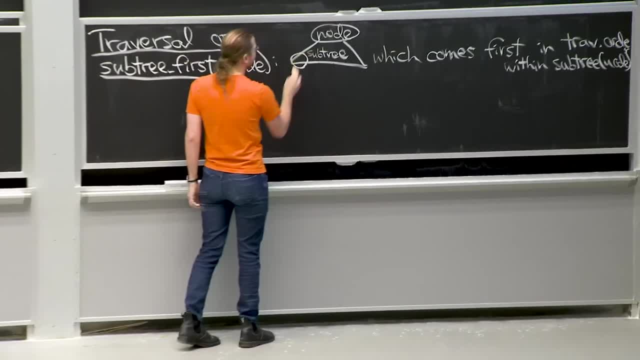 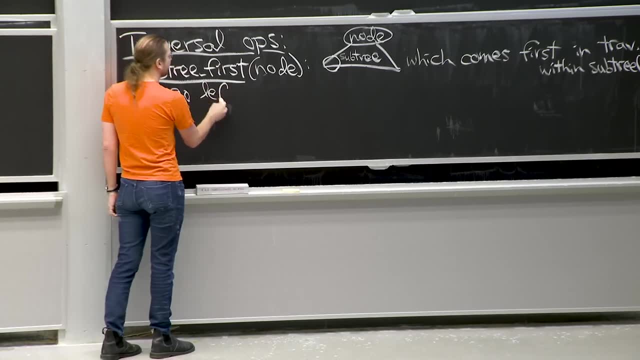 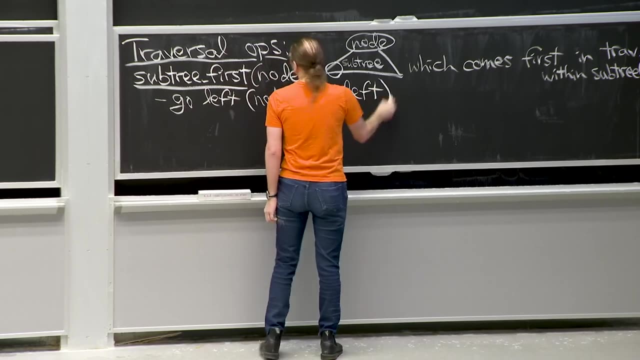 The leftmost leaf In the picture. it's here, but pictures can be deceiving. We just want to go left as much as possible, And when I say go left, I mean this iteration: node equals nodeleft, If you just look at our definition. 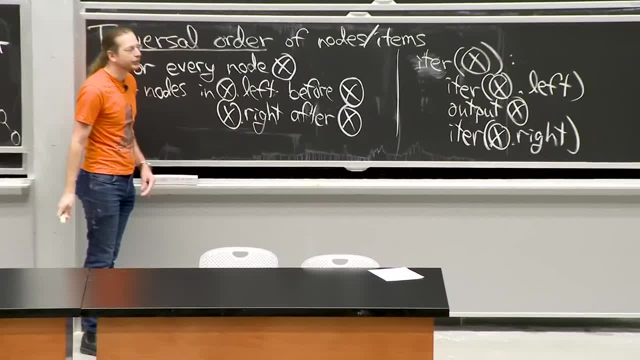 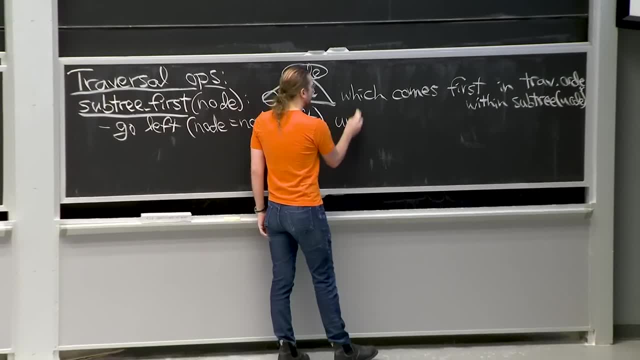 all the nodes on the left come before x and all the nodes on the right, So it's got to be in the left subtree, if there is one. Of course, we can't do this forever, So let's say until we would fall off the tree. 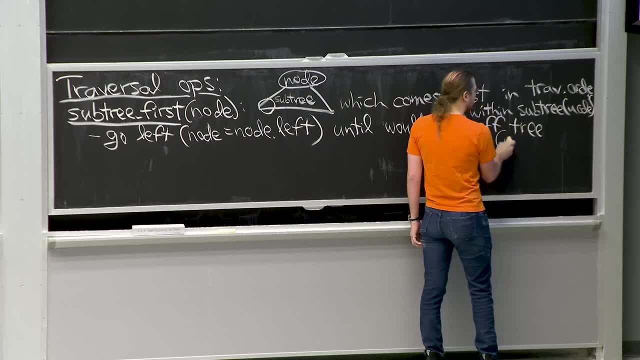 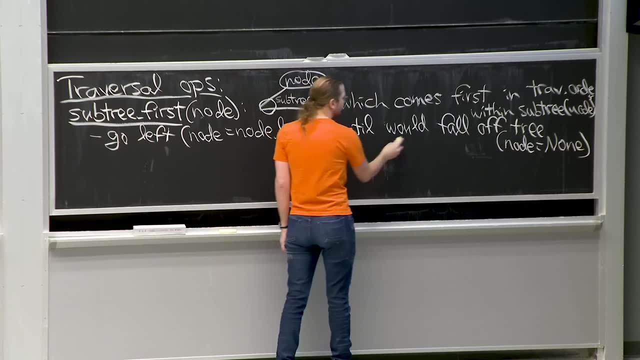 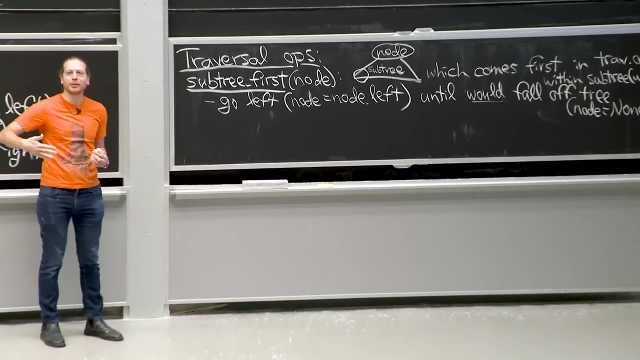 which means node is none, but we stop before. that would happen. So this is like the directions, like, oh, you keep driving until you see this door and it's the block right before that. It's like, well, that's not very helpful. 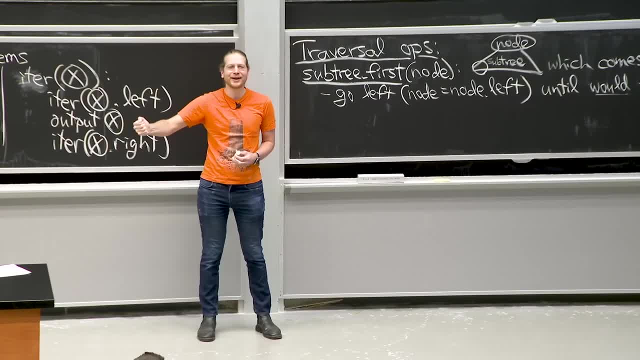 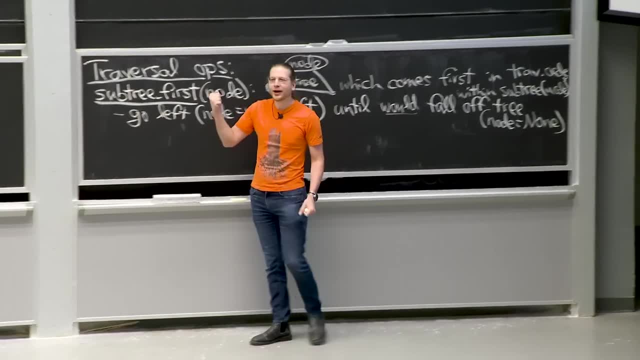 So you keep iterating- node equals nodeleft- until node becomes none, and then you undo one step. You all know how to program that. It's not hard. So that's it, Thank you. So that last non-none node which might actually 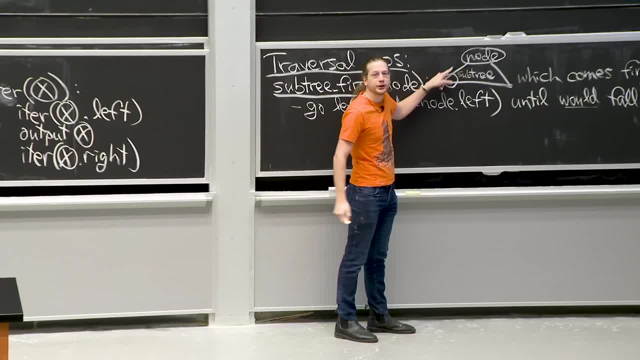 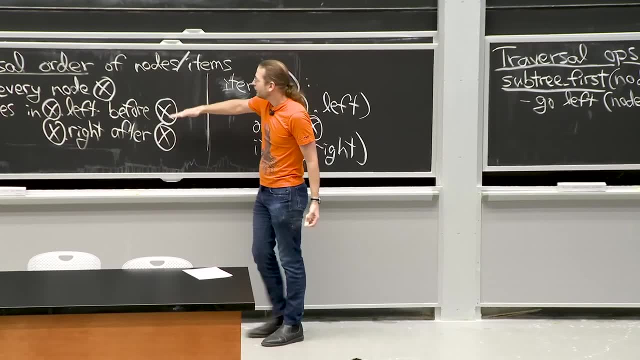 be the root, it might be node, Maybe it has no left children, But in that case I claim node is the very first in its subtree traversal order, because if there are no nodes in the left that come before x, then x is actually first. 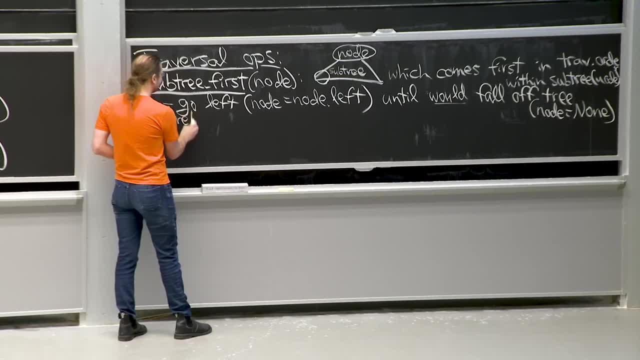 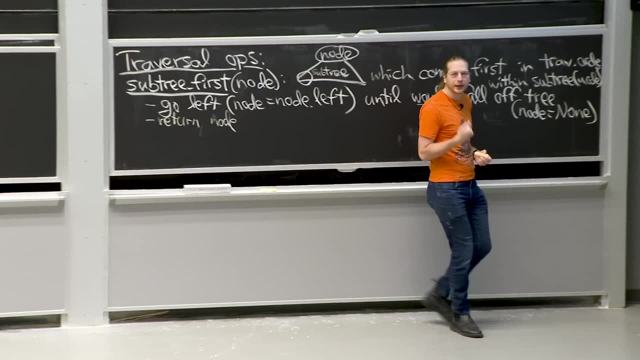 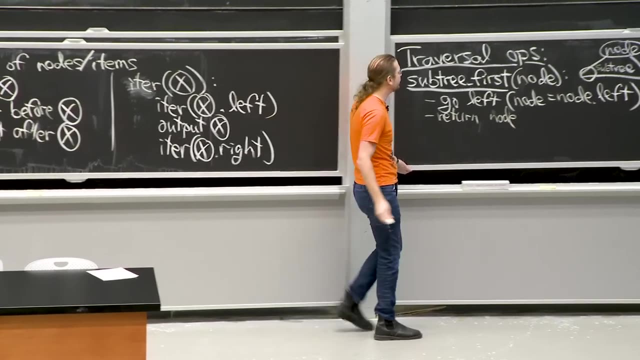 So that's it: Return node. So I'm modifying node in place here And the very last one before I hit none. that's the minimum. That's the first item in the traversal order. Similarly, you can define subtree last. Let's do a more interesting one. 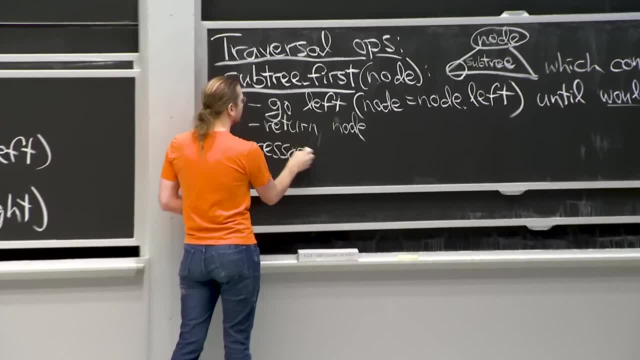 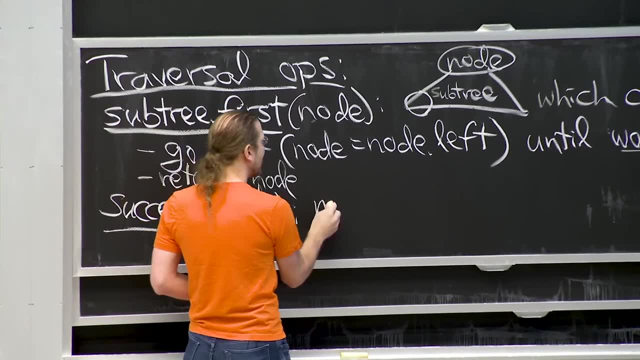 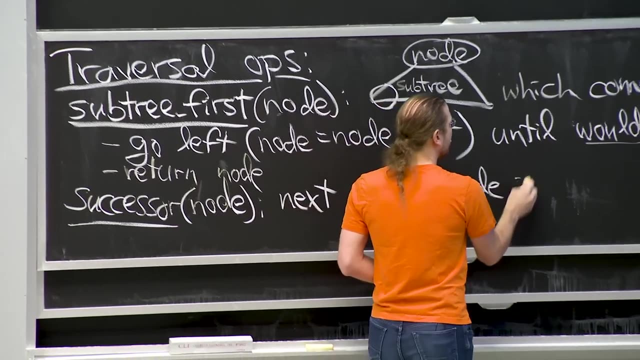 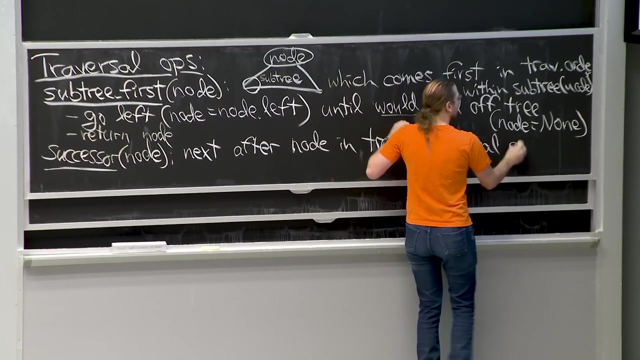 Successor node. So in this case I want to know what is the next after node in the overall tree's traversal order. OK, here I was restricting to a single subtree. Now I'm thinking about the entire tree and the entire traversal order. 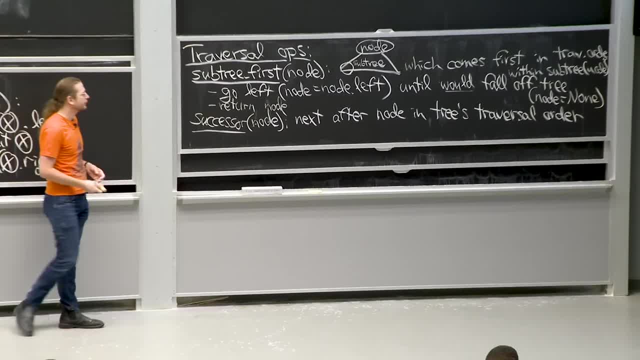 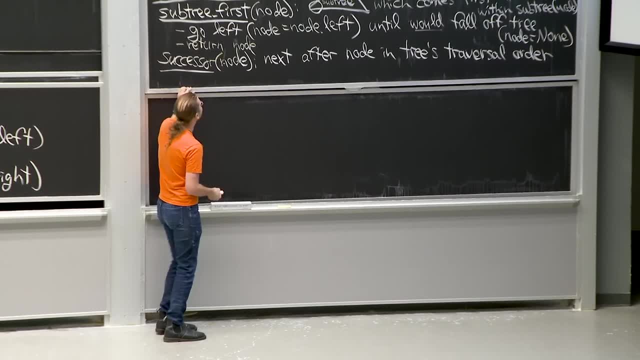 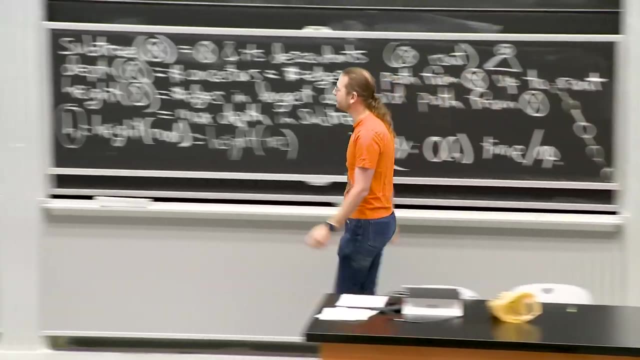 And given a node, I want to know which one comes next. Call this the successor. I feel like I should make some kind of royal family joke now, But I don't know how. So every node has a unique successor. Let's do some examples. 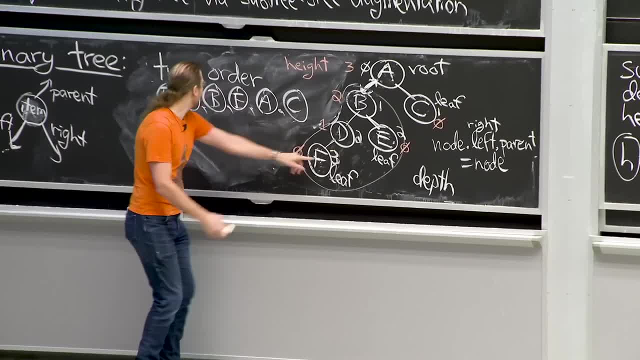 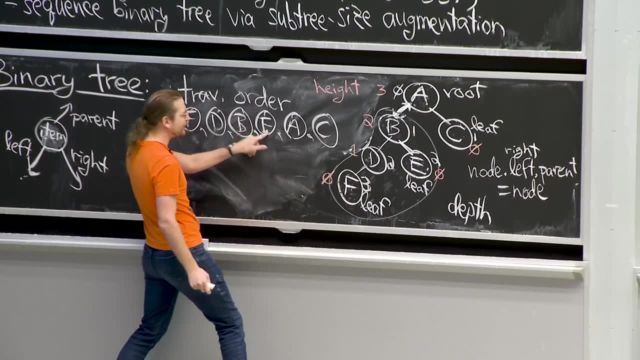 So we can start with f, the successor of f. If we just index into this list. the successor is d. Successor of d is b. The successor of b is e. It's very easy to read successors off when I have the traversal order written down. 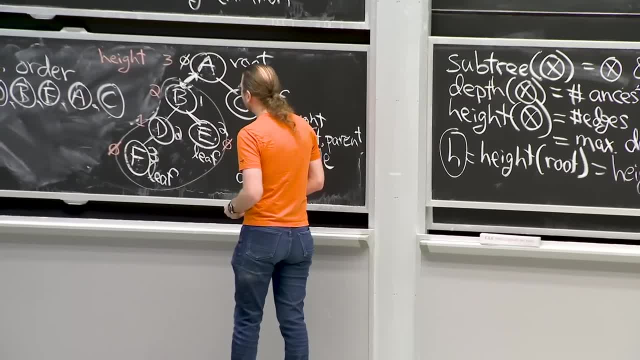 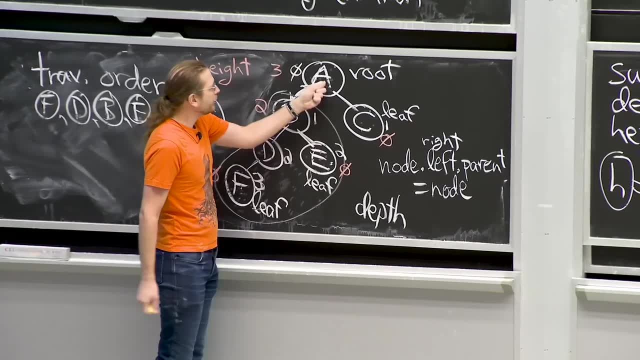 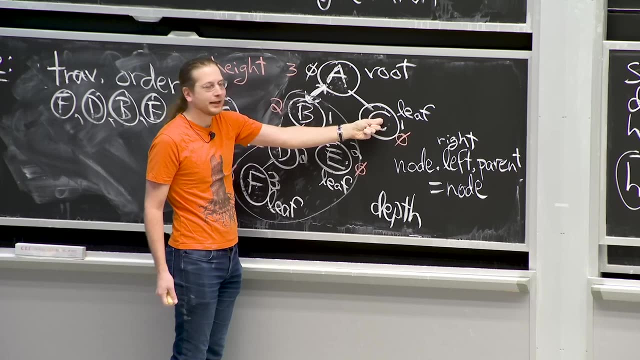 But let's think about how to do it in the tree. Let's see there are going to be two cases. If I look at the successor of a, it has a right child And in this case the right child of a is the successor. but that's not always the case. 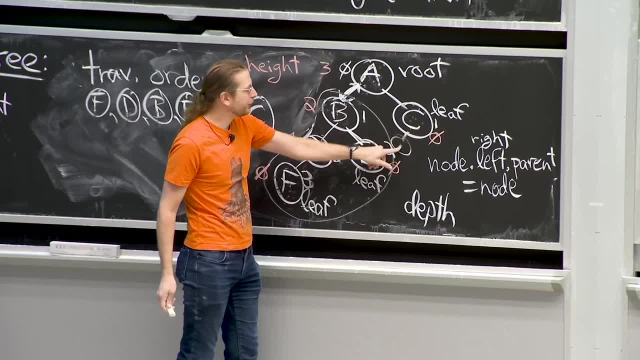 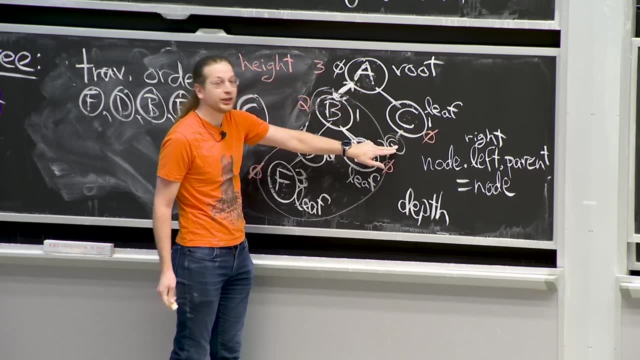 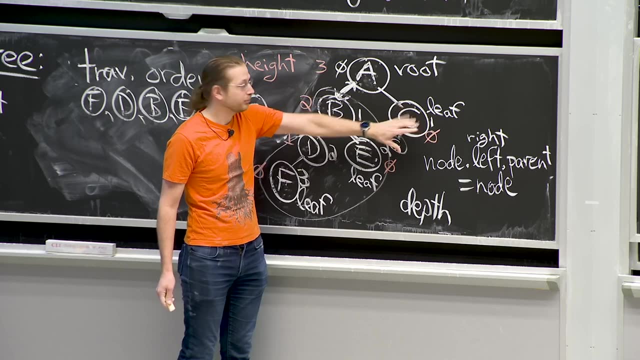 I don't have a good example, But if I had another node here, let's call it g. the successor of a is actually g, Because all of these items come after a in the order, But which one comes first? The leftmost leaf. 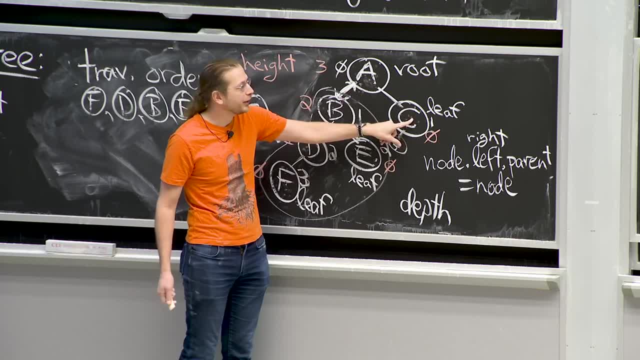 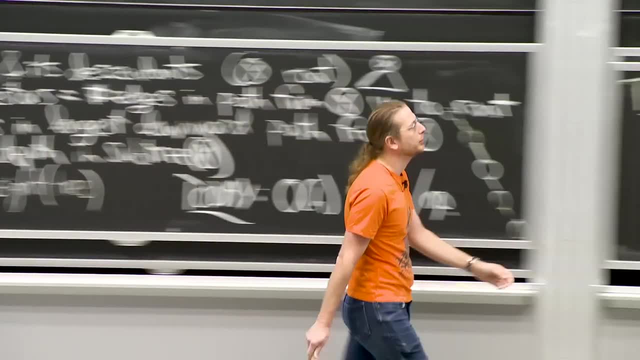 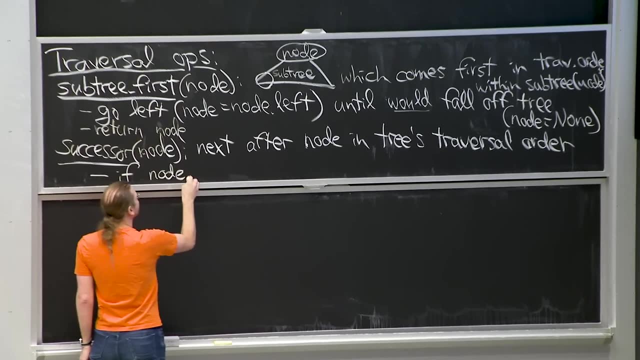 That's the problem we just solved. So if a has a right child, what we want is the leftmost leaf, the first thing, The first thing in that subtree, the right subtree, right child subtree. So this is case one, If node dot right. so if we have a right child, 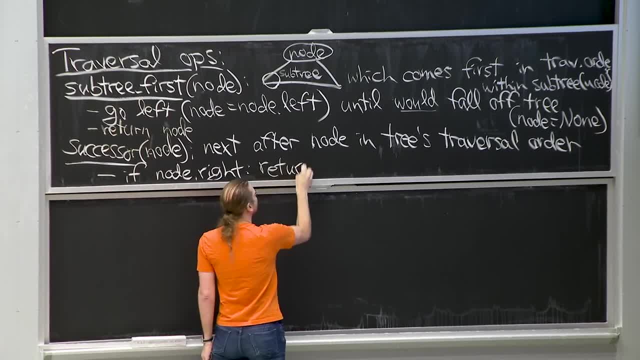 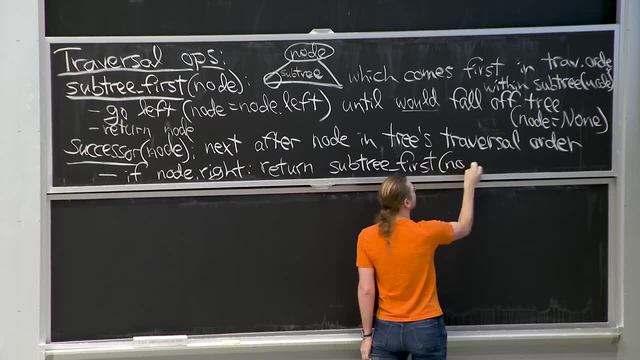 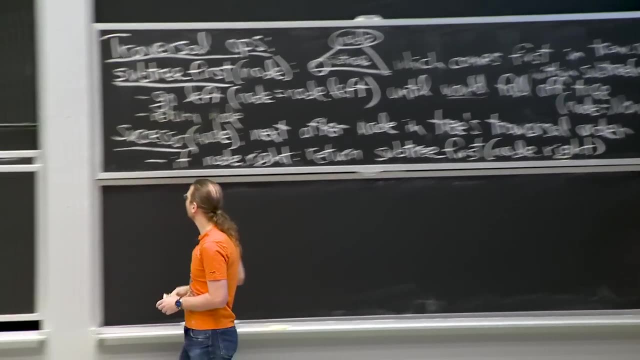 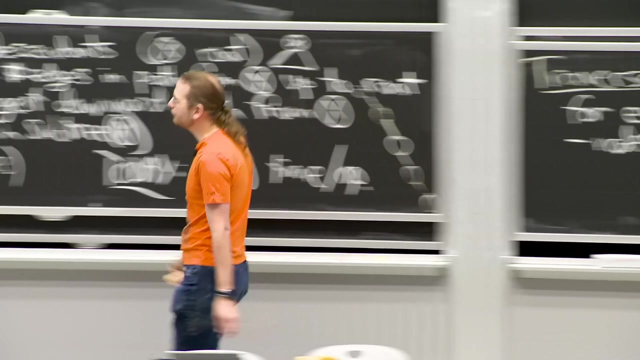 then what we want is subtree first of the right child. Great, We can reduce to this other operation. But what if the node doesn't have a right child? For example, it could be a leaf Say: we're taking the successor of 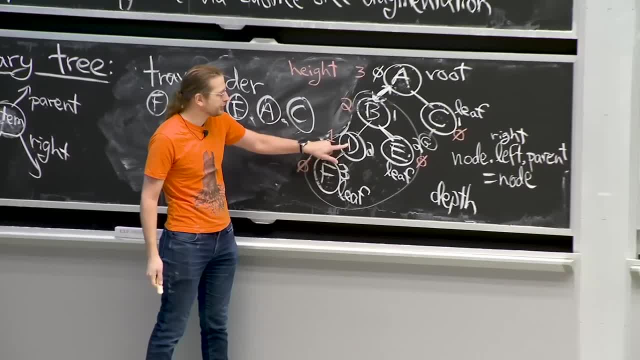 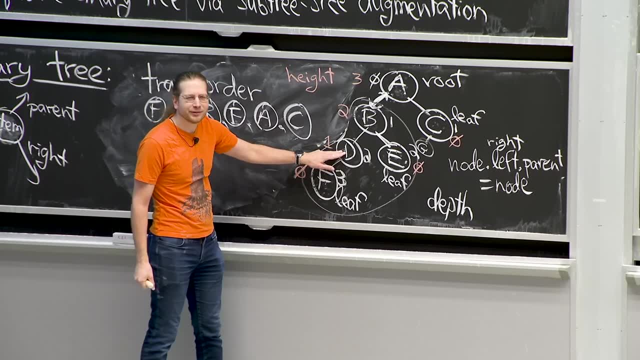 I mean, it doesn't have to be a leaf. It could be f, which has no children. It could be d, which has one child, but no right child. So what's the successor of f? Well, it's d which, in this case, is the parent. 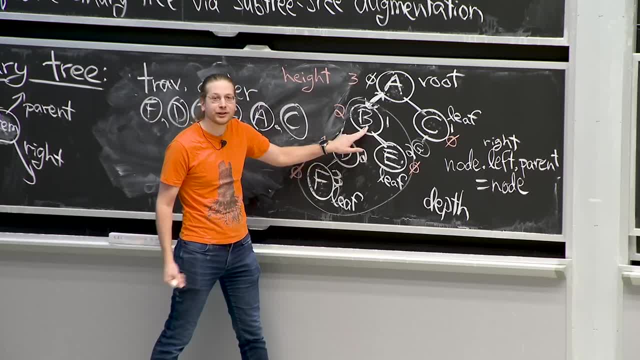 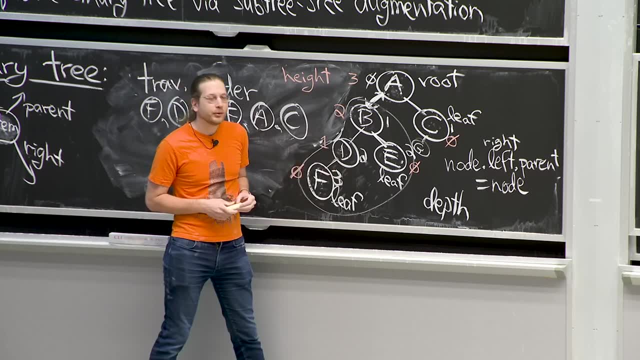 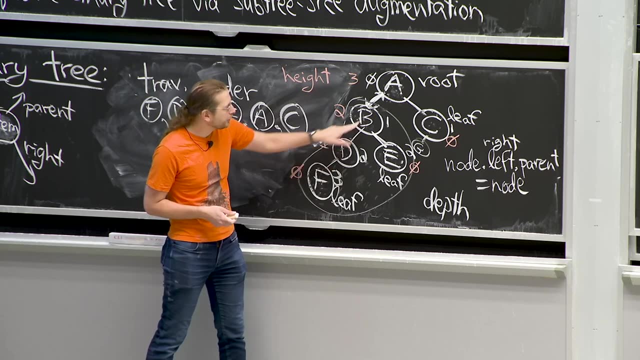 but it's not always. For example, if we do successor of e, its parent is actually earlier in the order, because e was a right child. Here, f was a left child and so its parent was after. Successor of d happens to be b because it. 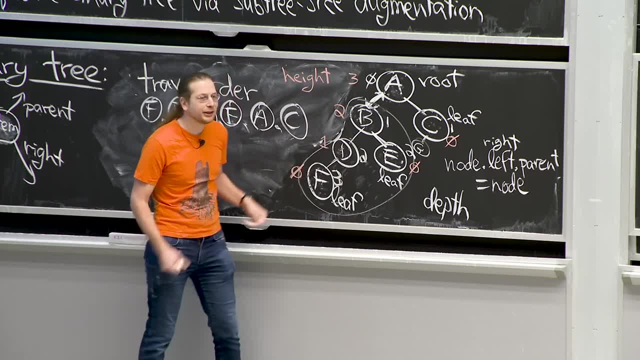 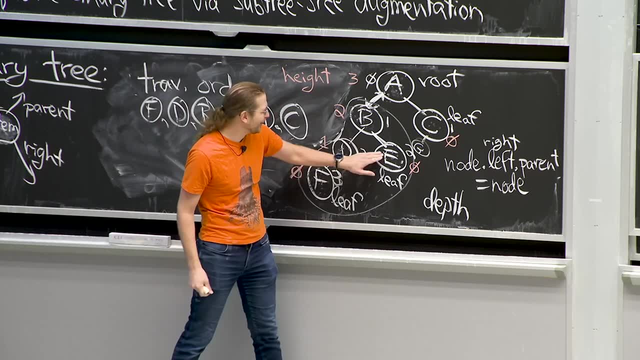 was the left child of its parent. So that seems like the easy case. If we're the left child of our parent, then our successor is our parent. basing on this small example- But we can argue it generally in a moment- What's the successor of e? 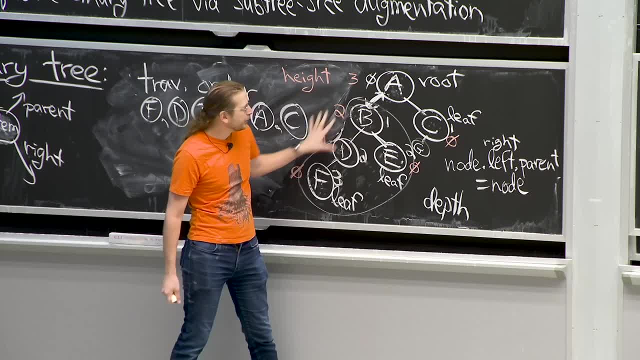 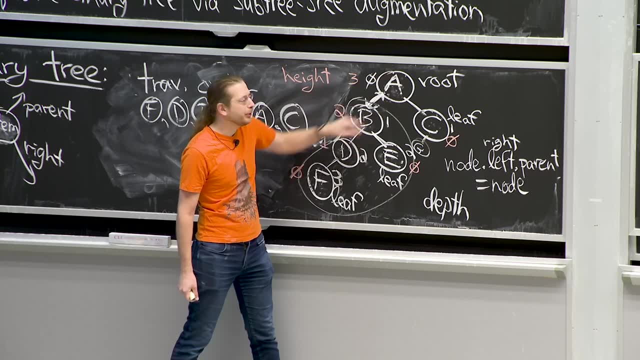 Well, it's not b, because that comes earlier. In fact, all the things in b's subtree come earlier or equal to e, So we have to keep going up And then it turns out the successor of e is a, because this subtree was the left child of a. 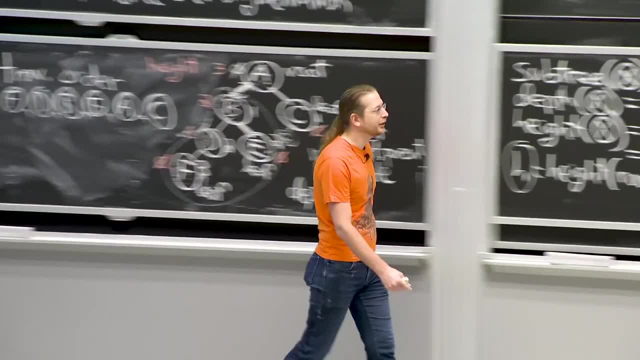 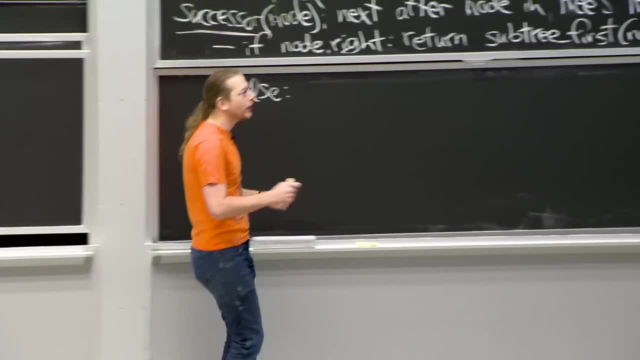 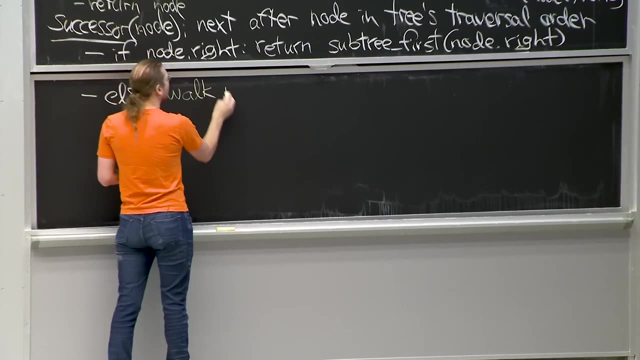 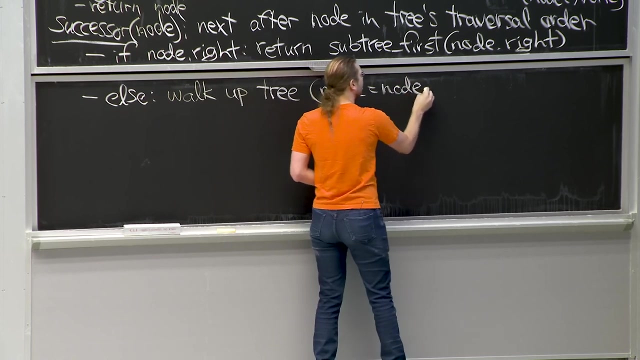 because b was a left child of a. So the general strategy is: walk up the tree until we go up a traversal whose reverse direction would be left OK, so walk up the tree. When I say walk up, I mean node equals, nodeparent iteration. 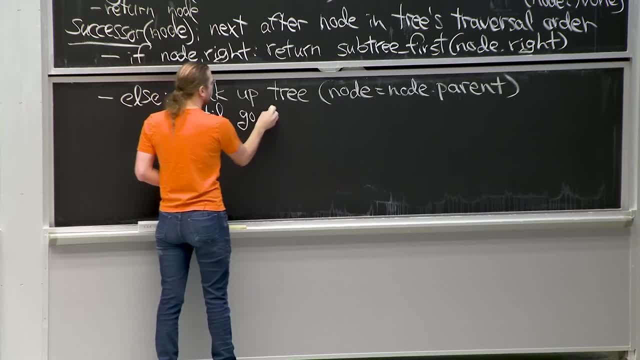 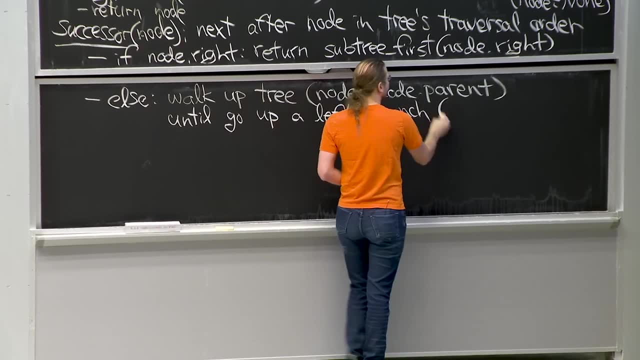 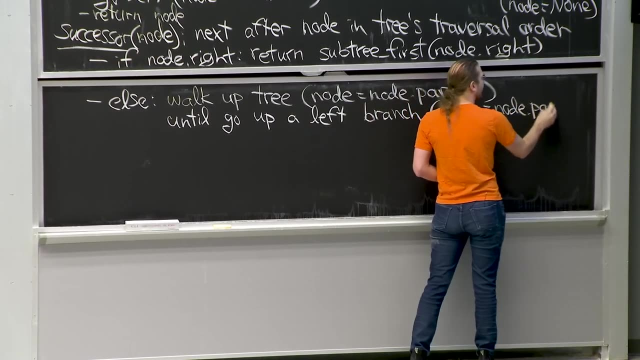 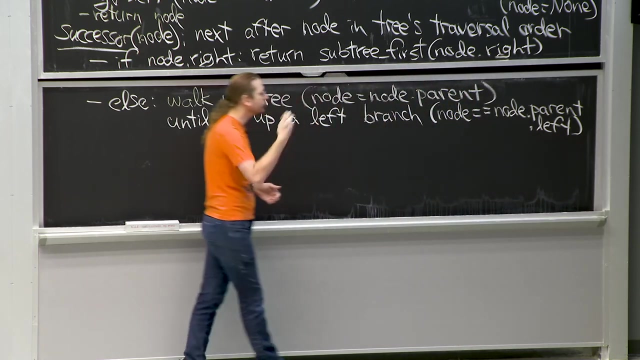 until we go up a left branch. So this would mean that node before we do the change, node equals nodeparentleft. OK, so we can check that. And then, after we do that traversal, that parent is exactly the node we're looking for. 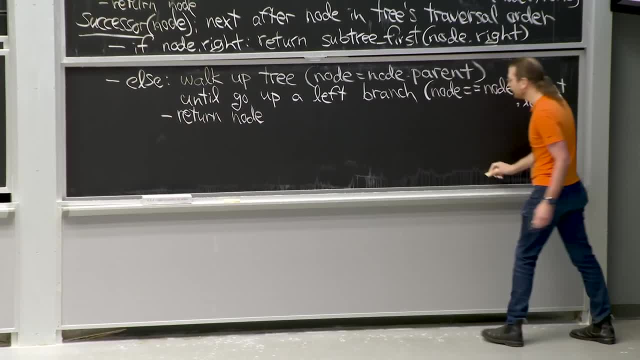 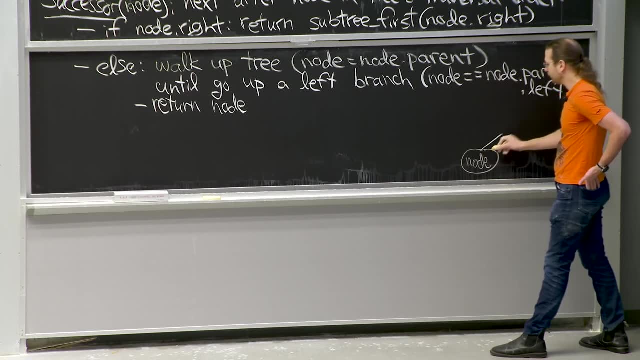 Why is this true in general? Let me draw a more generic picture. So we're starting at some node And let's say its parent is b. The parent is to the right, so it comes later in the order. for a while, Sorry, get this backwards. 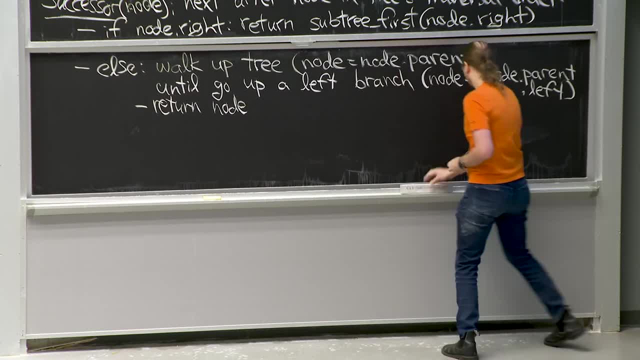 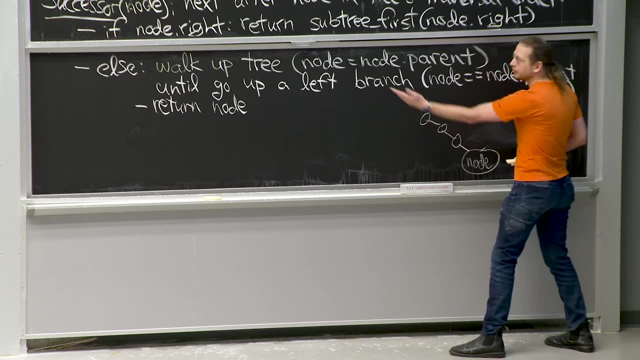 We're doing successor. It goes to the left for a while, So all these nodes will come earlier in the order because, by the definition, everything in the right subtree comes after And at some point we have a parent that's to the right. 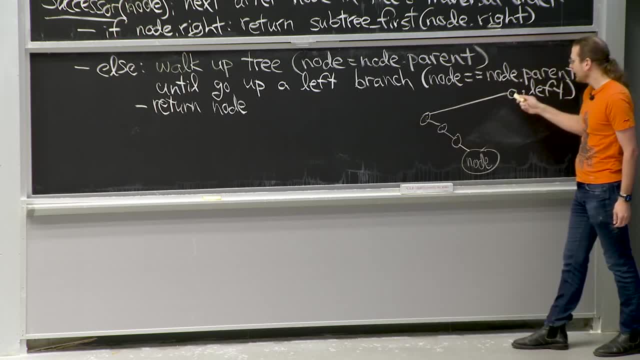 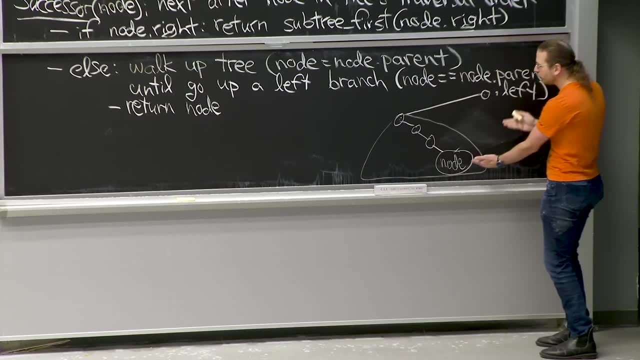 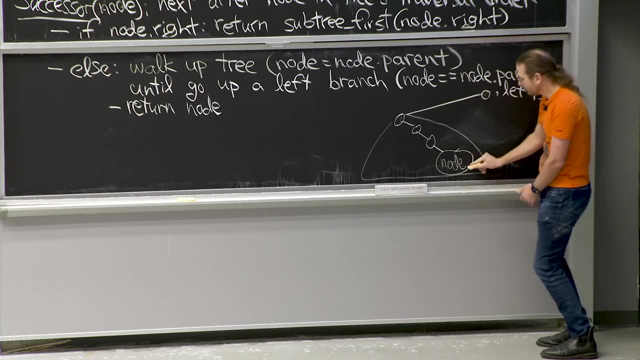 meaning this node was the left child of this parent And that node, by definition, will come after all of the nodes in here. And could there be anything in between node and this parent, grandparent, ancestor? Only if there was something in this subtree. 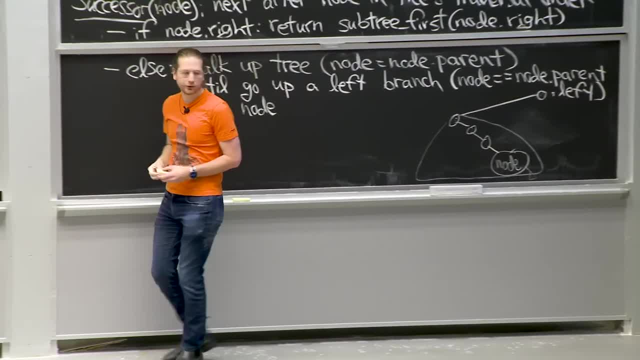 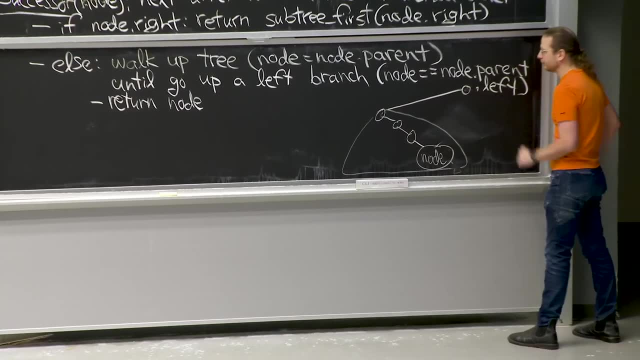 And we're in the case here where there is no right subtree of our original node. So this is where all the nodes in between node and here would be, but there aren't any And therefore this is the successor. So that's sort of the general argument why this works. 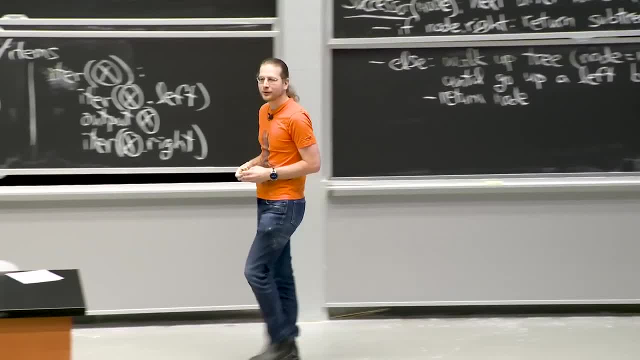 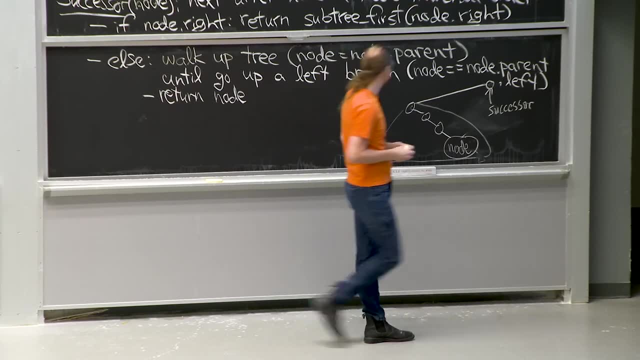 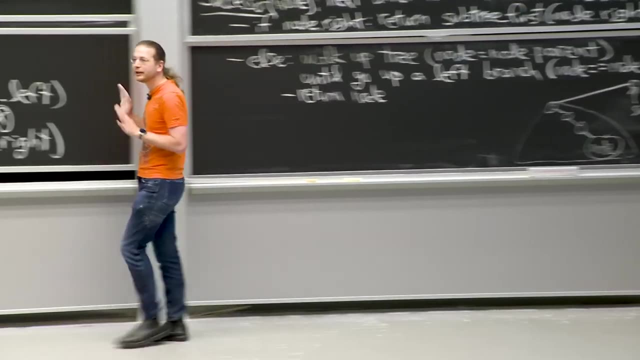 I see a question. Yeah, Can you say that? the goal of the left branch is that we are to place the node of the subtree that is in the left child into the traversal order. Placed into the traversal order, So the traversal order is never explicitly computed. 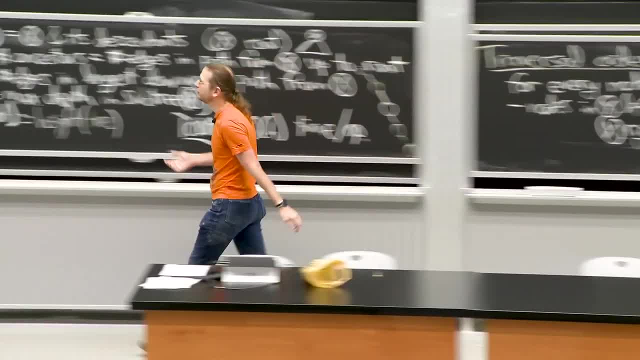 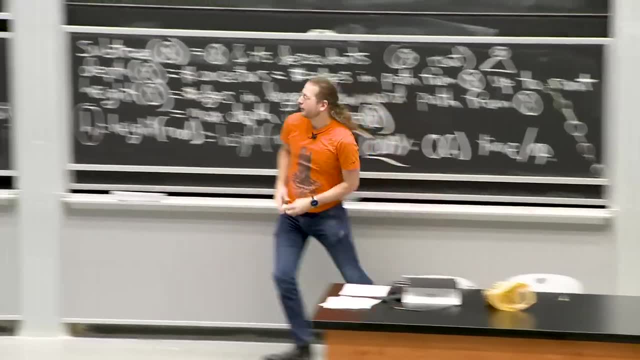 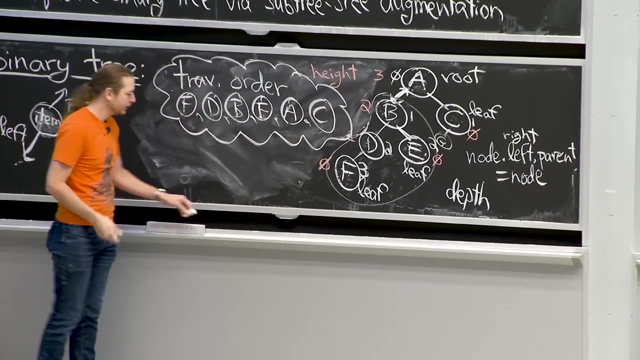 It's always implicit. We can't afford to maintain this as, say, an array. This is just in our heads. Maybe I will draw it with Cloud around it. We're just thinking this. It's not in the computer explicitly. 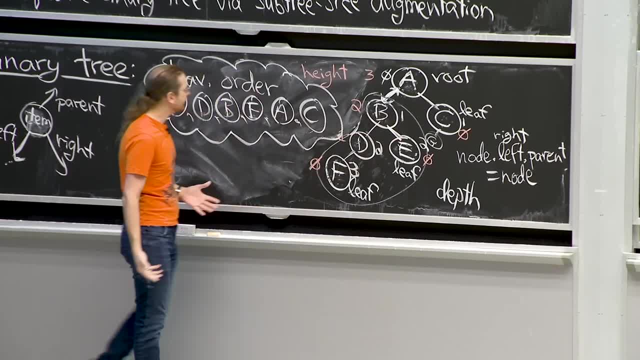 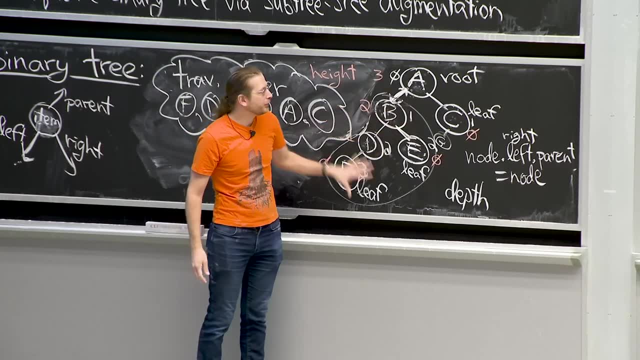 In the computer, all we store is this, And the reason is this is expensive. We can't maintain an array of things and be able to insert it in the middle. whereas this is cheap, I can afford to maintain this structure and do all these things. 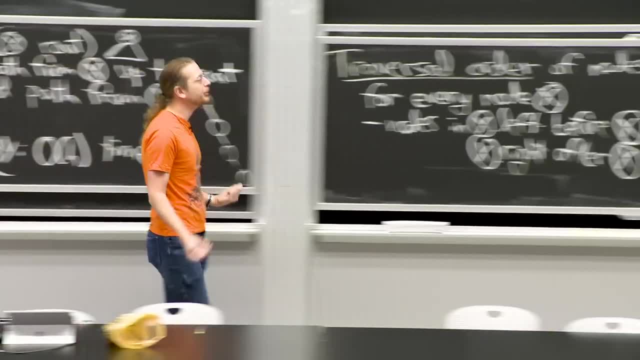 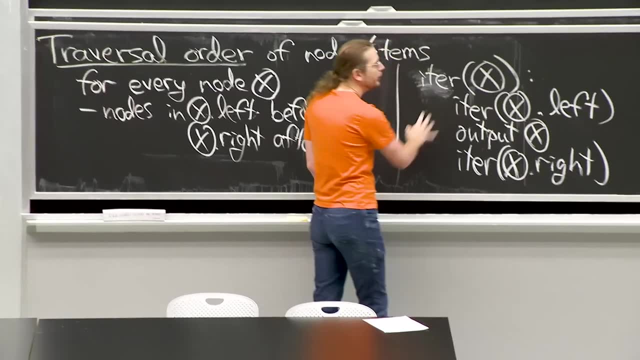 And so the reason we're talking about these operations is they're letting us manipulate the order or, in this case, letting us iterate through the order. So this was an algorithm for iterating through the entire order, But that takes linear time. This was getting started in the order. 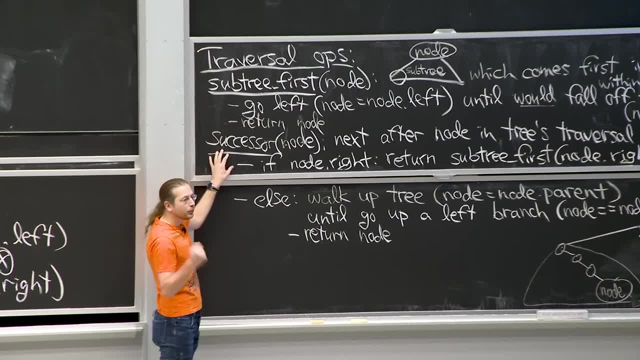 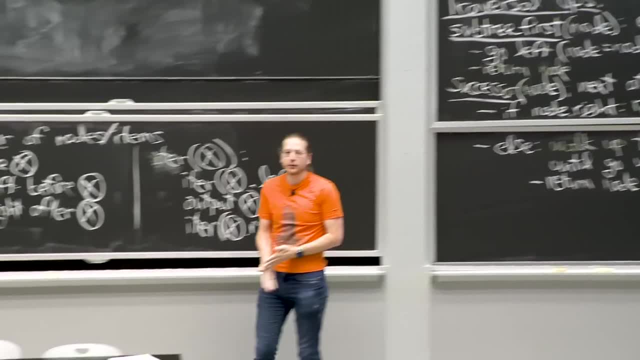 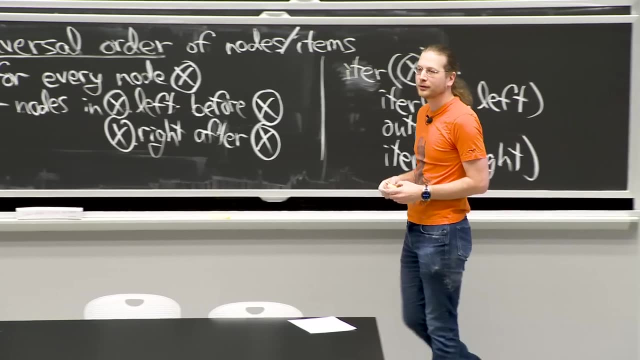 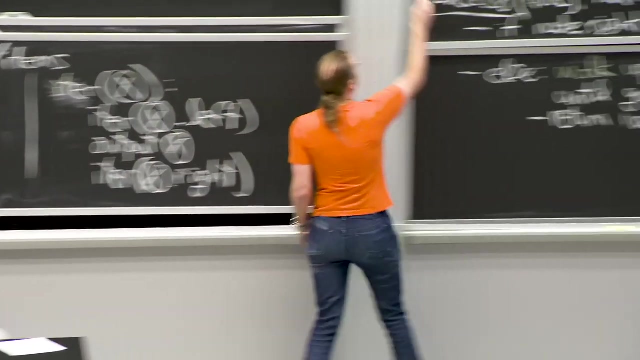 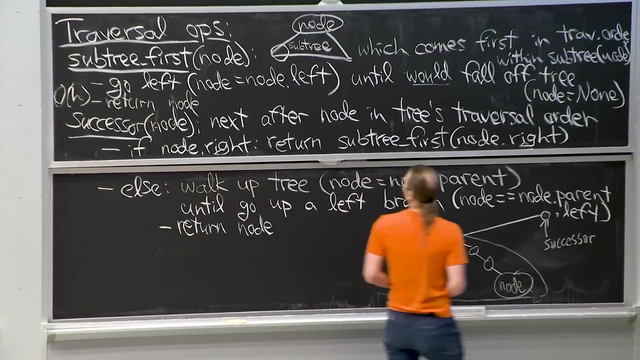 Find me the first thing in the order, And this was given one node. Find me the next one. How long did these operations take? Yeah, At most the height of the entire tree. In fact, it's going to be the depth of that first node. 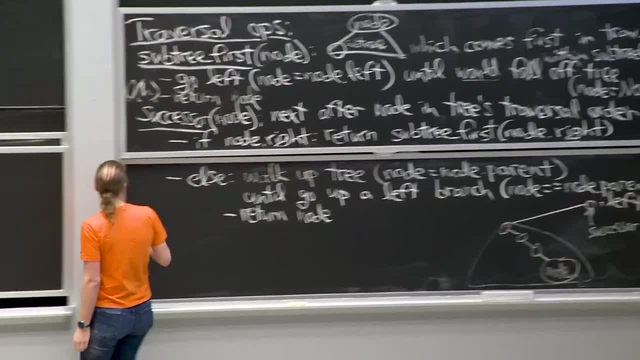 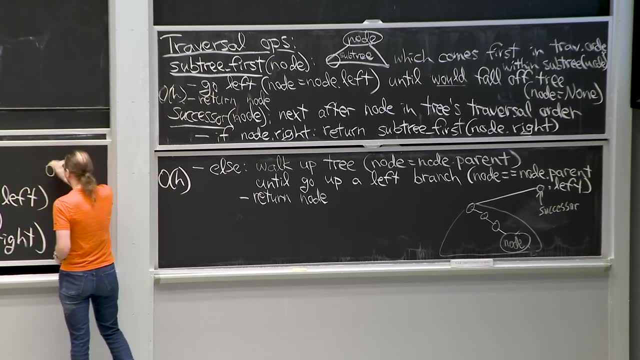 But in the worst case that's the height of the entire tree. In general, all of these operations are going to be order h. We need to think about it in each case, except for this one, which is order n. So we're iterating through the whole thing. 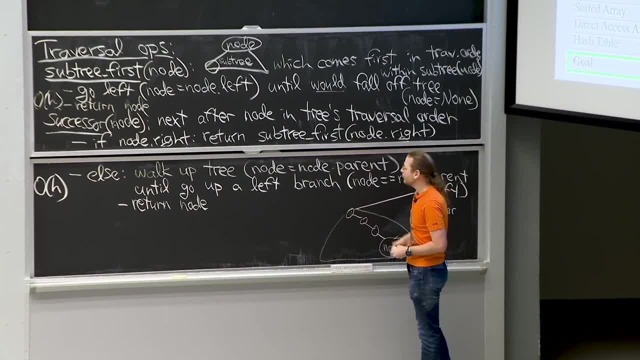 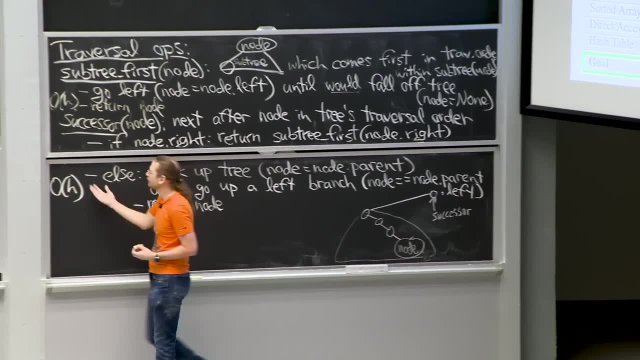 In this case we're just calling subtree first, So that takes order h time. Here we're walking up the tree instead of down, But that's going to cost exactly The height of the node. We happen to stop early, But worst case, order h. 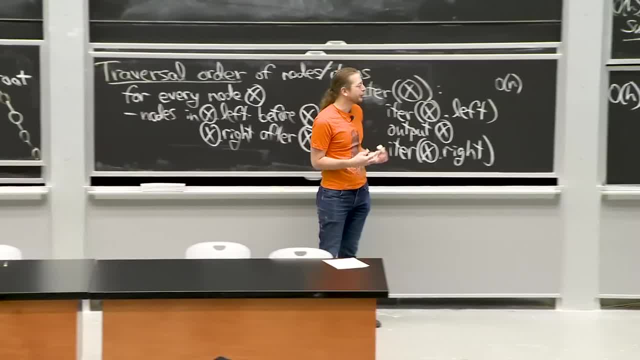 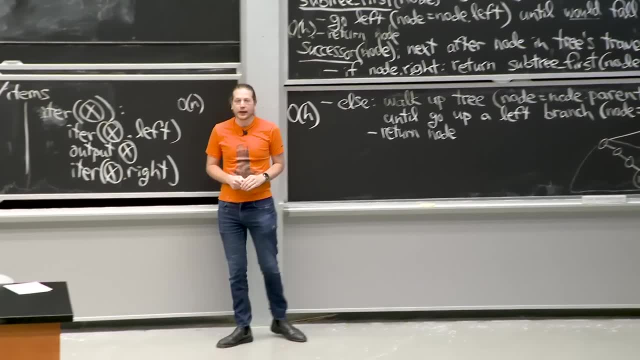 For all the operations we consider. today we just want to get an order h bound And later we will bound h. So the point is these are fast. If h is small, like log n, these are almost instantaneous, Whereas if I had to update the explicit traversal order. 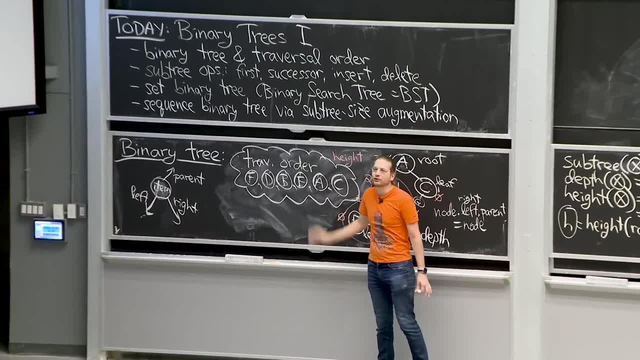 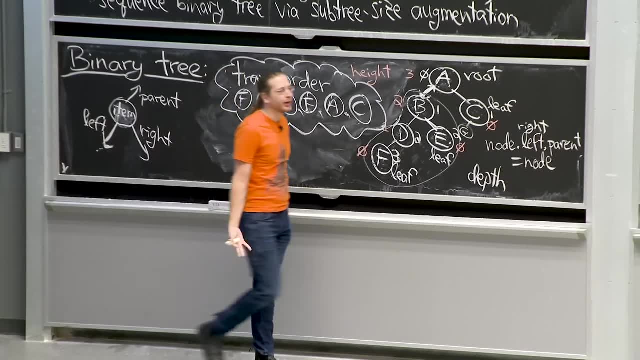 say, as an array, I would have to spend linear time every time I make a change. And, yes, it would be fast to do successor if I had this stored explicitly, But maintaining it would be impossible, Maintaining it efficiently would be impossible. 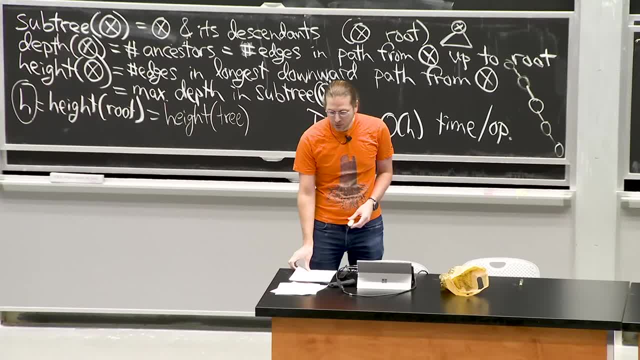 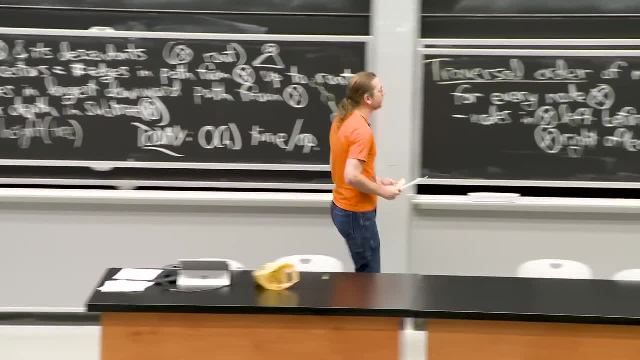 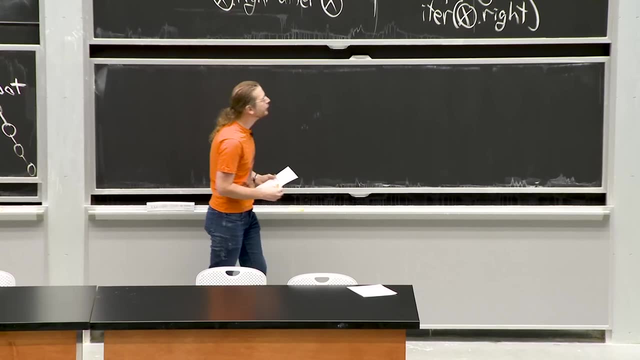 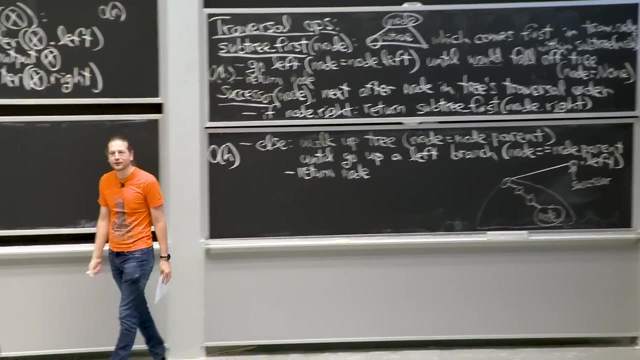 Question, Question. So for the traversal time it's a very fast, Yes, Cool. So these were queries where I want to follow see what's next in the traversal system. So let's talk about the traversal sequence. Now let's talk about actually changing the traversal sequence. 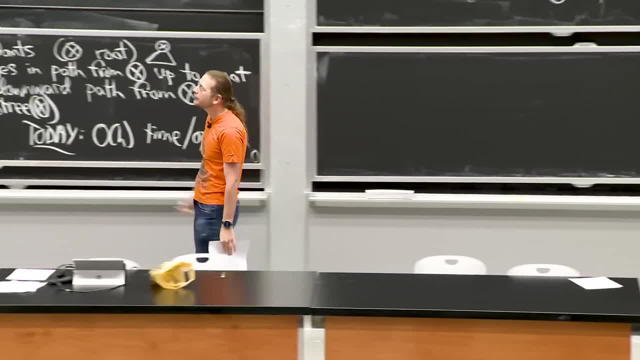 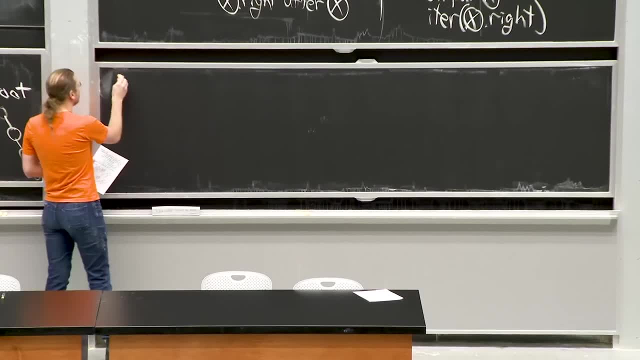 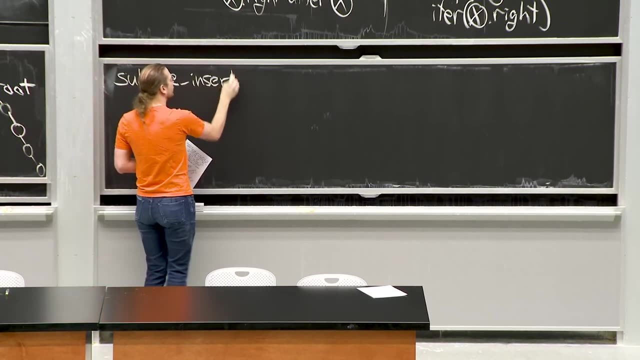 So these are insert and delete operations. These will correspond roughly to insert at or delete at, But we're not quite in the sequence world yet. Instead, we're going to focus on inserting or deleting in the middle of a subtree. So I'm going to have two nodes. 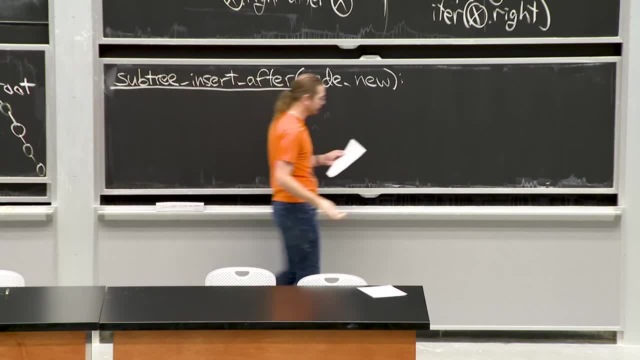 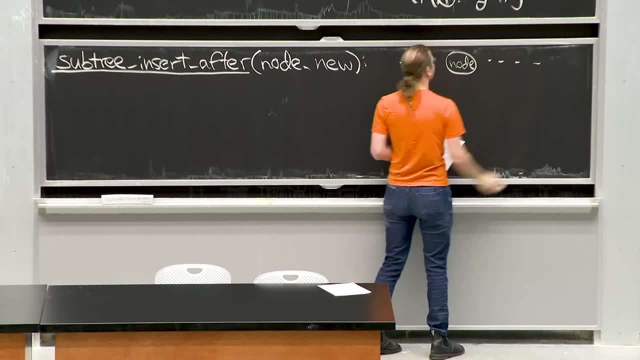 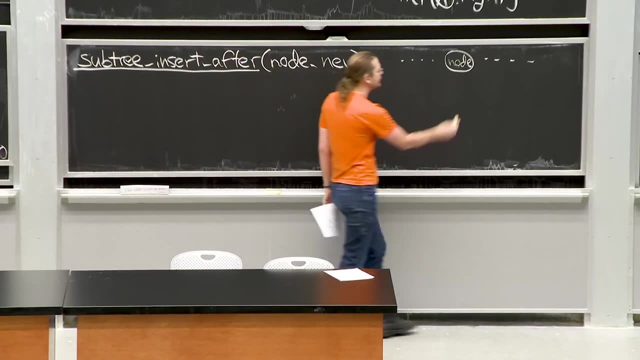 So in the traversal order. so node already exists in the tree, New is a new node that does not yet exist in the tree, Hence I call it new, And what I'd like to do is insert new right after node, And there's a symmetric operation. 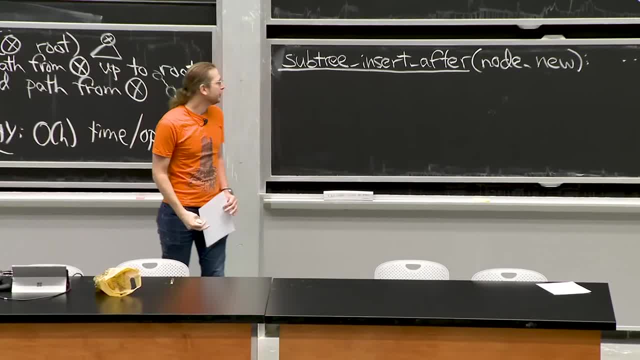 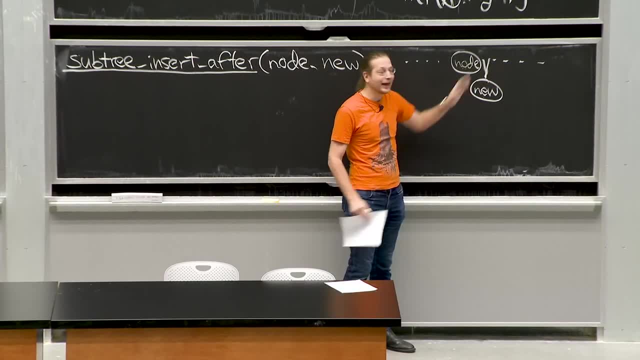 which is insert before It will be implemented almost identically, So we'll just focus on after. So I want to insert this new node in the traversal order which again is in our heads. This is all in our thought bubble. 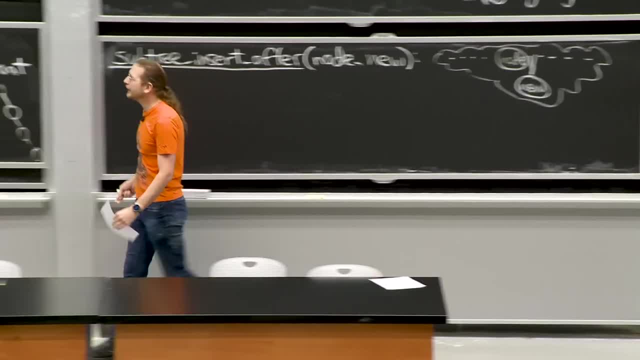 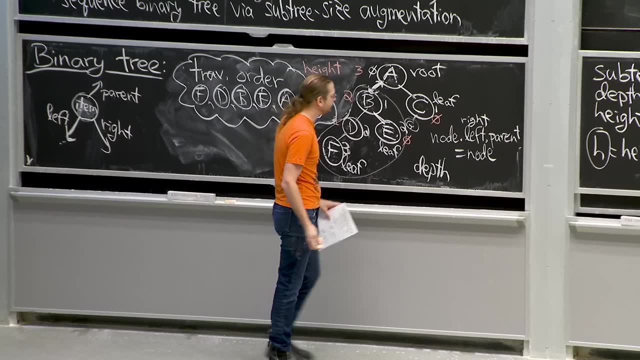 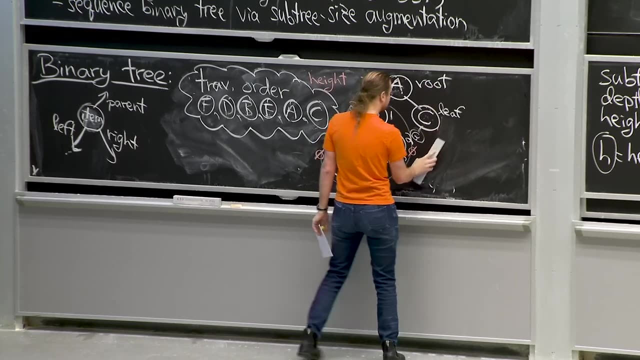 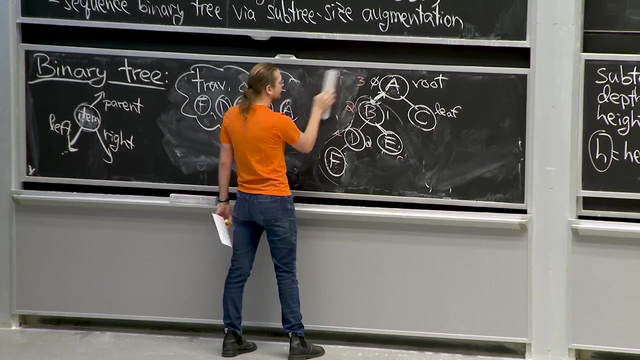 That's what we want to achieve, And we have to do it by manipulating this tree, And however we change the tree, it defines a new traversal order. So maybe let's do an example first. Actually, I probably want this in traversal order. 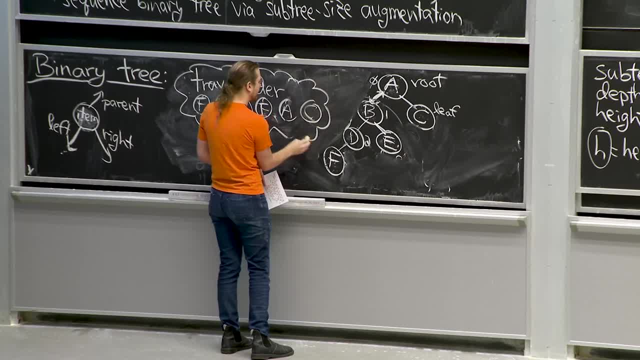 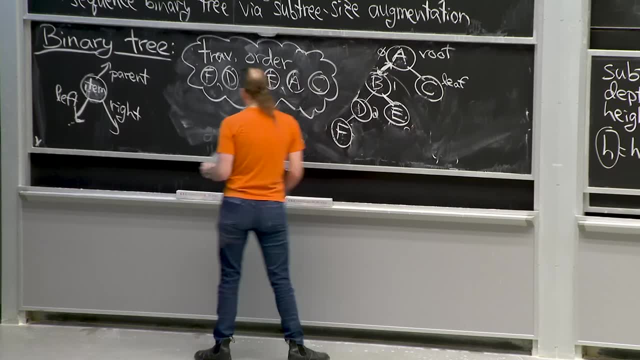 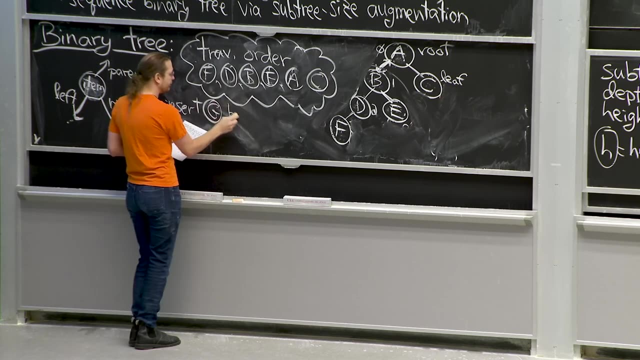 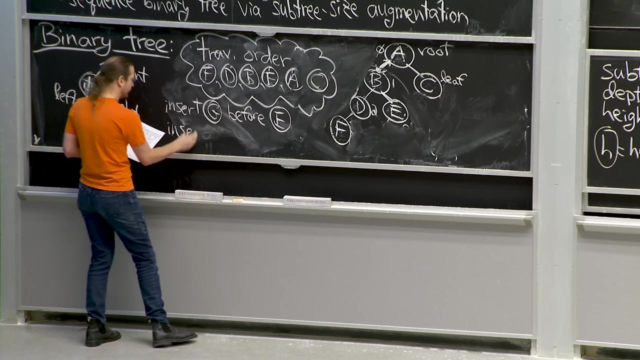 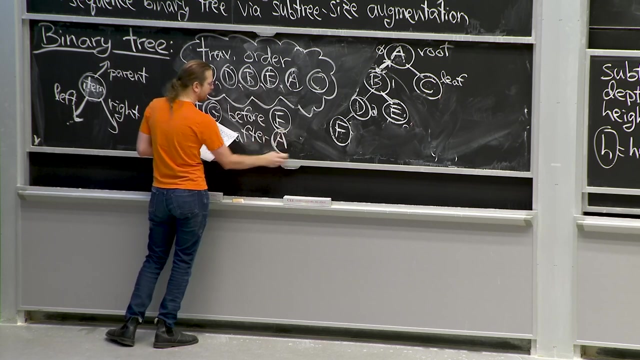 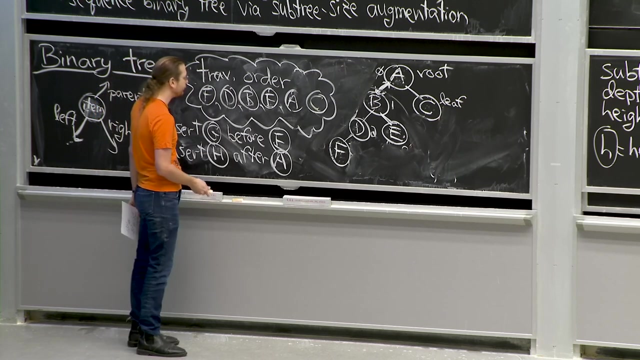 Keep track of that. So let's say the first thing we want to do is insert g before e. So that's going to be a new variable. I want to illustrate both of the operations. Insert H after E. A- OK, so insert G before E. 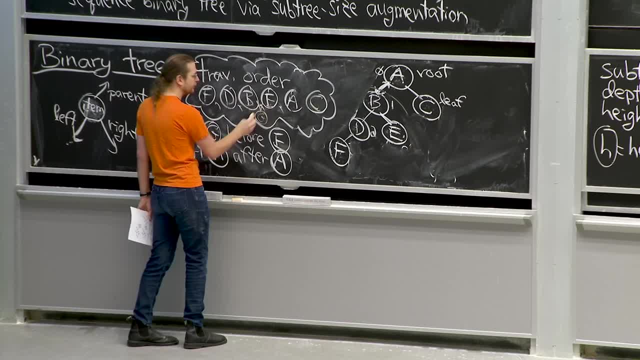 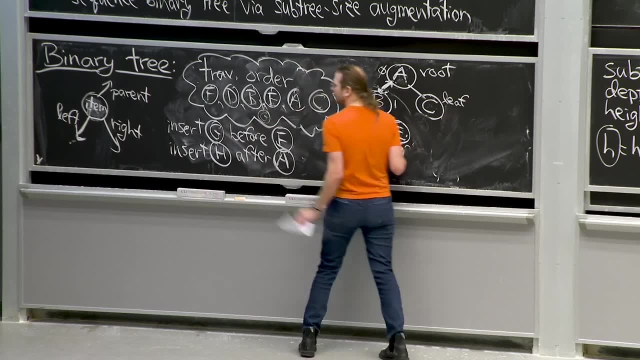 So, conceptually, what we want to do is insert G here, And so we're given the node E and we're given a sort of empty node, I mean a node that just contains G. It doesn't have any pointers yet. 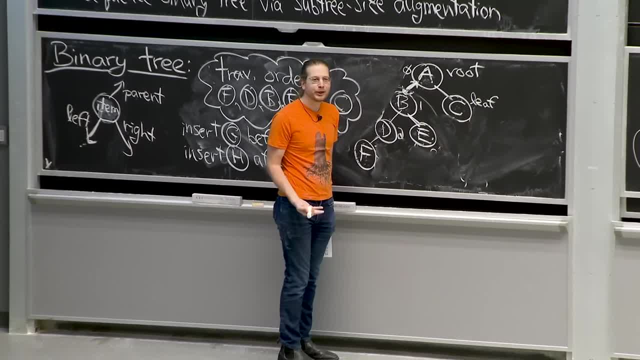 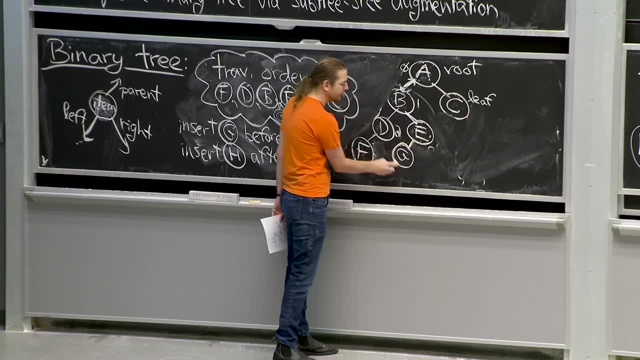 And we would like to put it before E. Where should I put it? Left child. So this is an easy case: If I'm trying to insert before and there's no left child, stick it there. If I'm trying to insert after and there's no right child. 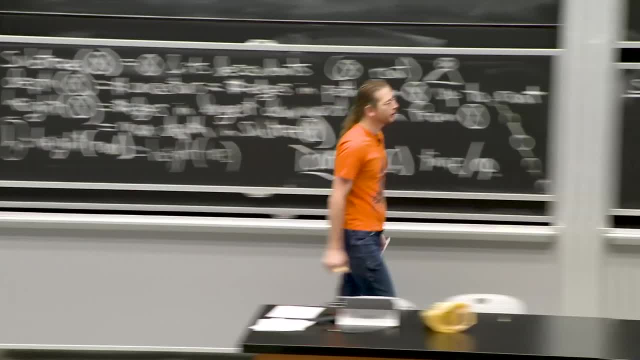 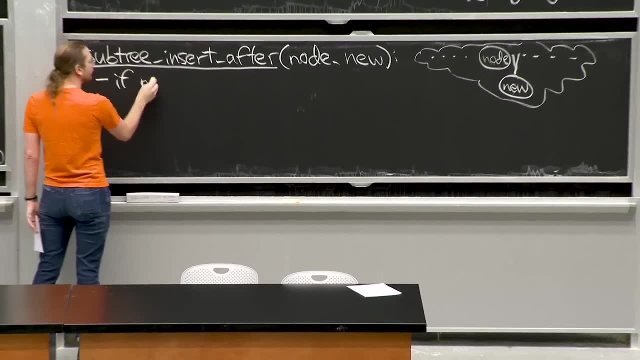 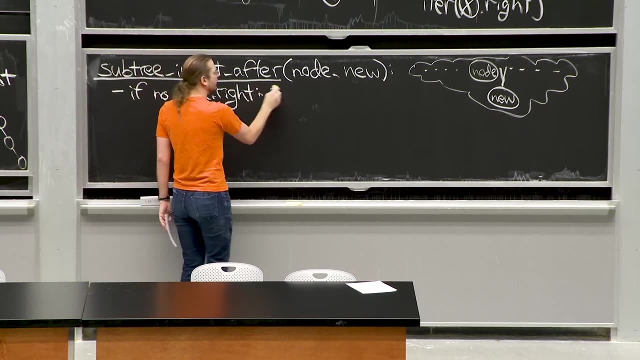 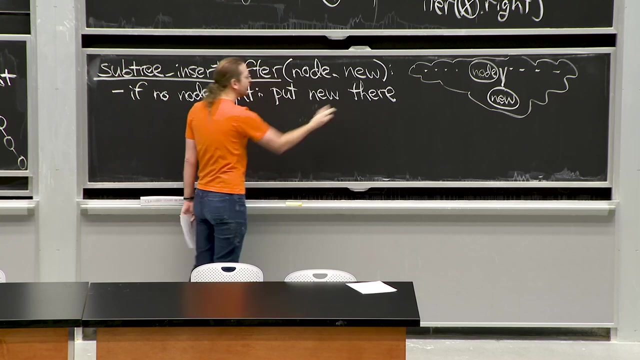 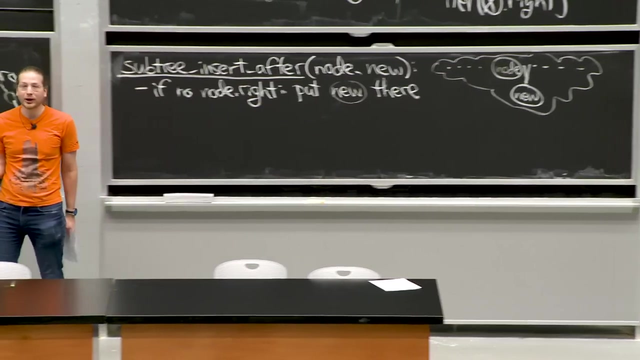 stick it there Easy. So let me write down case one. So here we're inserting after. So if there's no right child, put new there. I'm using informal language here, putting this new node there Instead of writing, for example, node dot. write equals new. 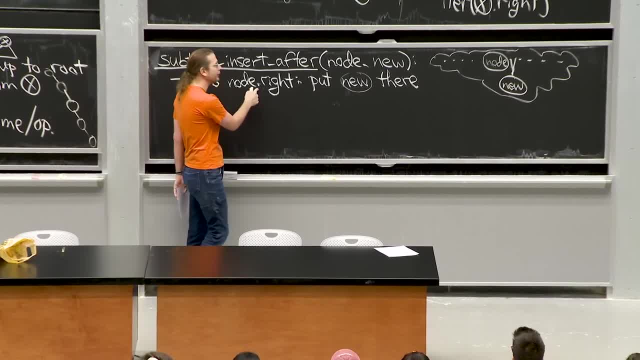 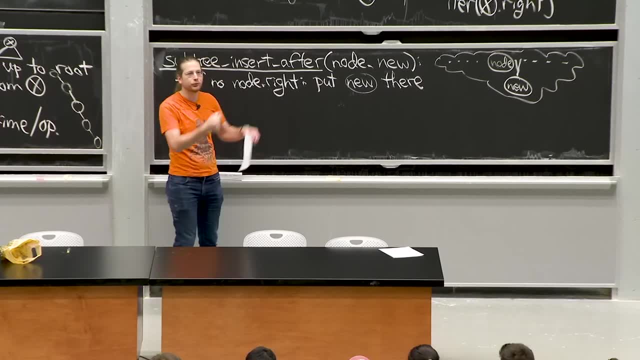 because that's, That's only one operation you need to do. One thing you would do is set node dot write equals to new, But you also have to set new's parent to be node dot write. So, instead of worrying about those two pointer changes, 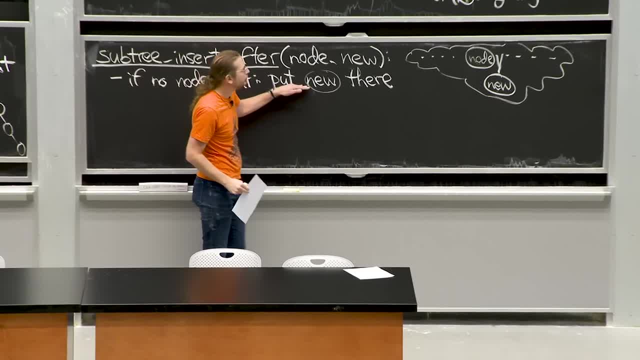 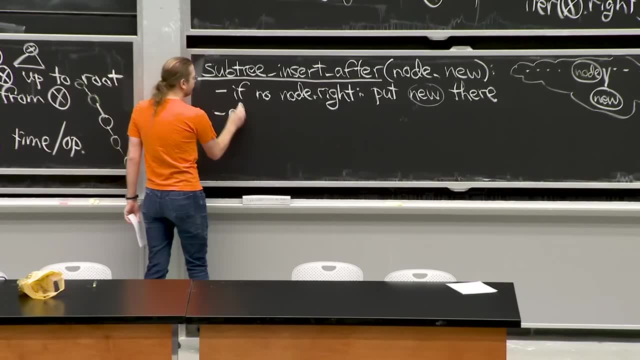 because we always do bi-directional pointer changes. I'm just going to use pseudocode And then in recitation you'll see actual Python code that does all this. So then there's the other case. So that should be the second example. 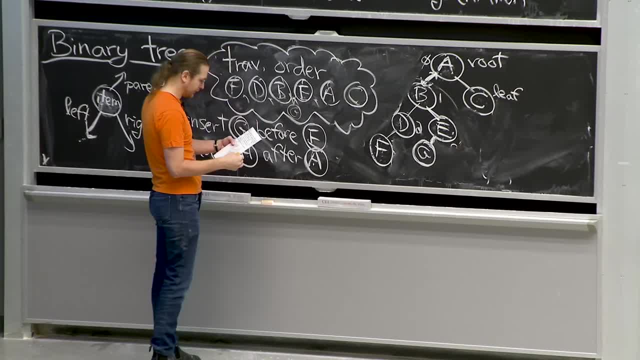 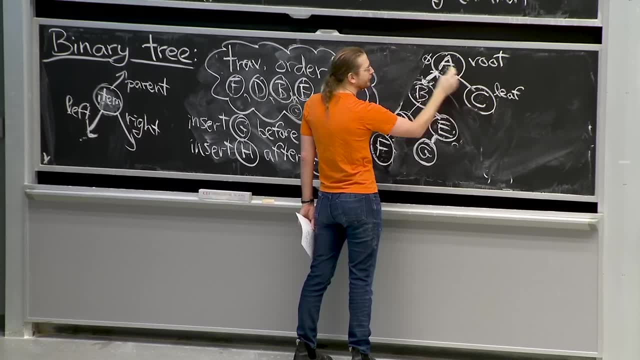 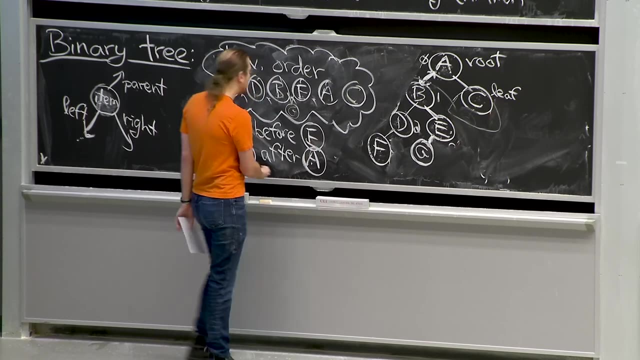 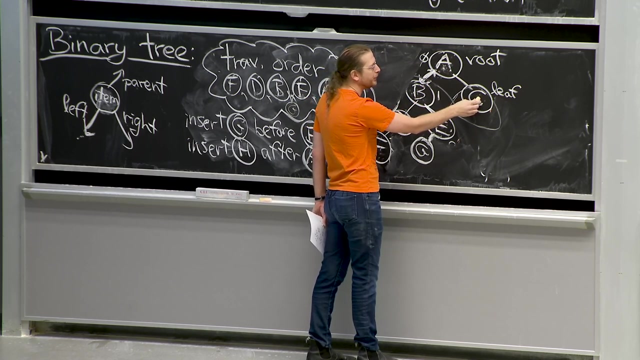 Insert H after A. Get it right. Insert H after A. So we already have a node after A in the right child in this right subtree. So where do I want to put H relative to A? Well, it should be to the right of A, but it should be before C. 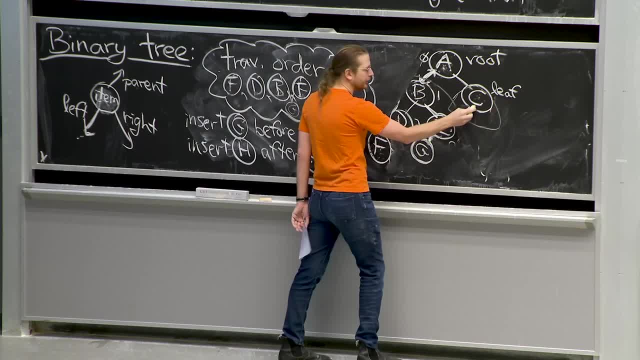 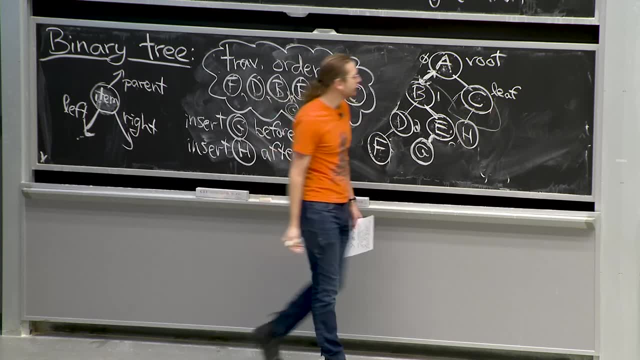 It should be to the left of C, So that would mean we want to put it here. OK, In this case it was pretty easy. It was pretty easy because this tree was small. Where do I want to put it? in general, 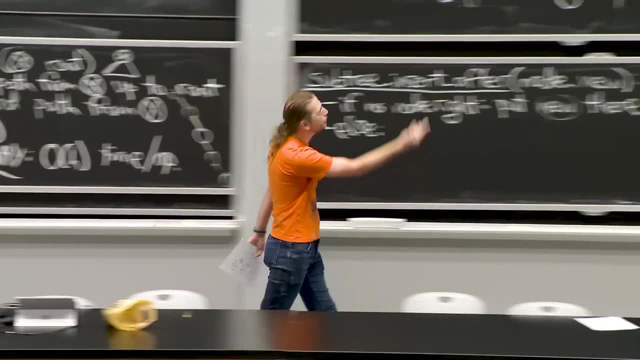 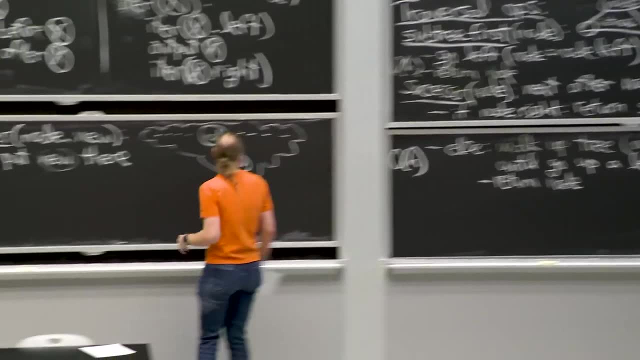 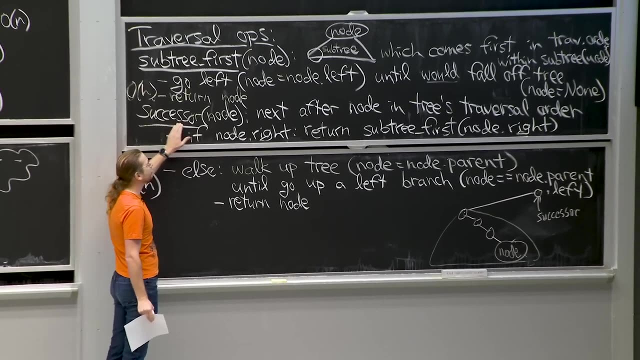 Well, wherever subtree first tells me to put it right, Subtree first is going to give me the successor. These are all kind of parallel. We're in the case now where our node has a right child And then successor tells us where the successor is. 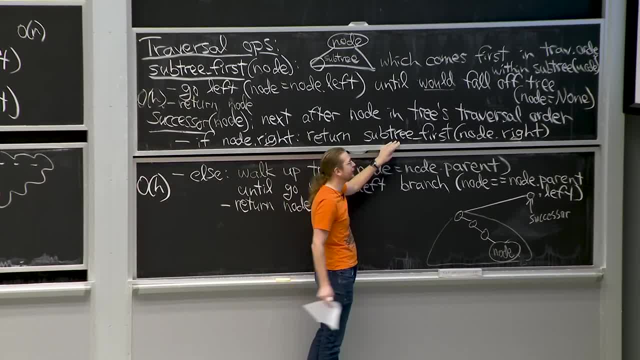 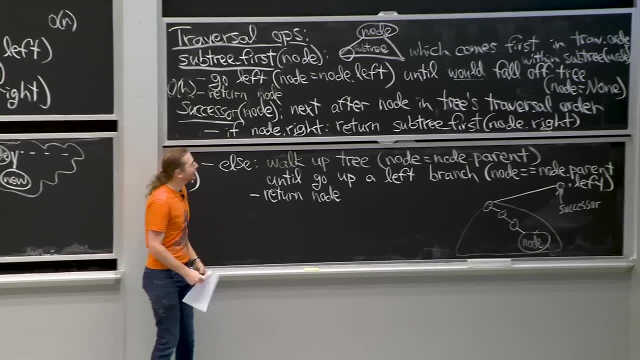 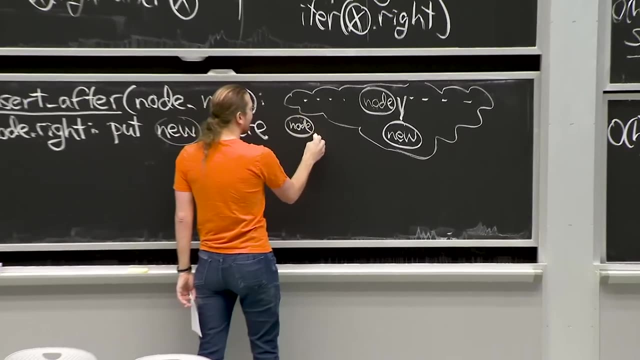 It is the first node, which is the leftmost descendant in the right subtree of the node. OK, A lot of pointers to follow in that sentence, but it's clear in the picture. So in this case we had node And there was no right child, so we just 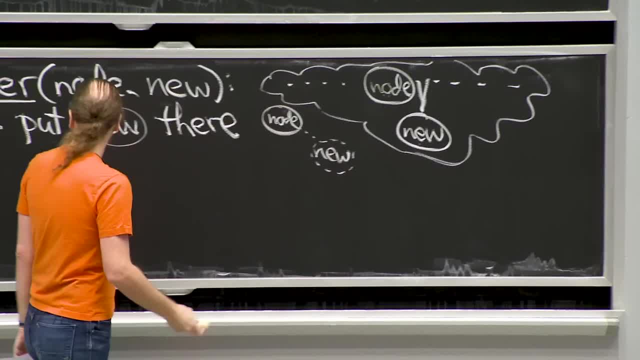 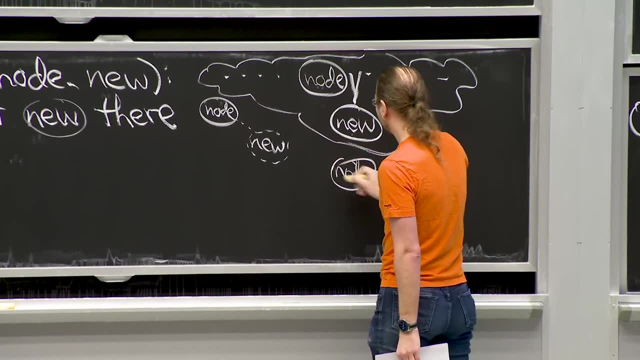 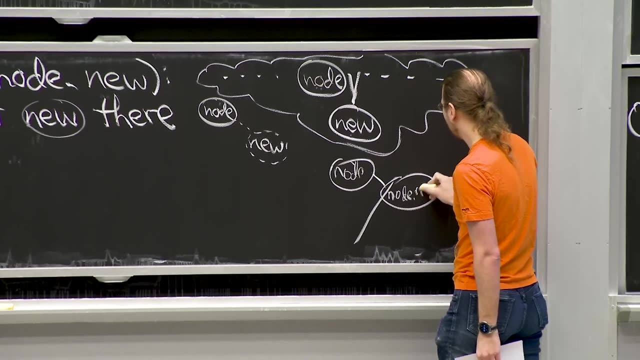 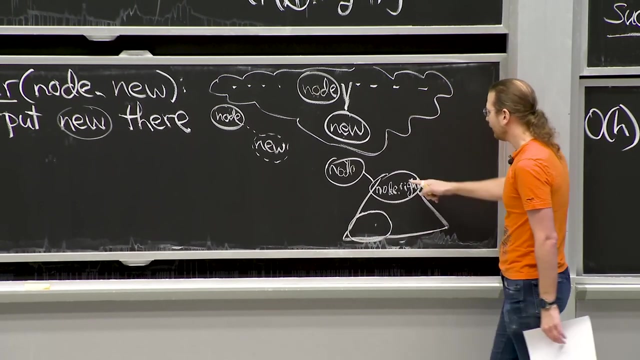 added new to be its right child. OK, In the other case we had a right child. So here is node. There's this node, here, noderight, which now we're supposing exists, And it defines a whole subtree. There's this one, which is the first node. 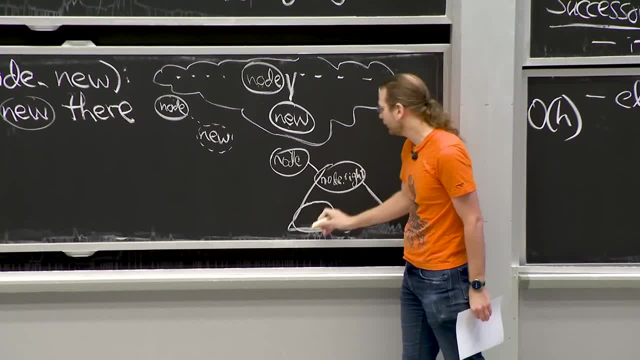 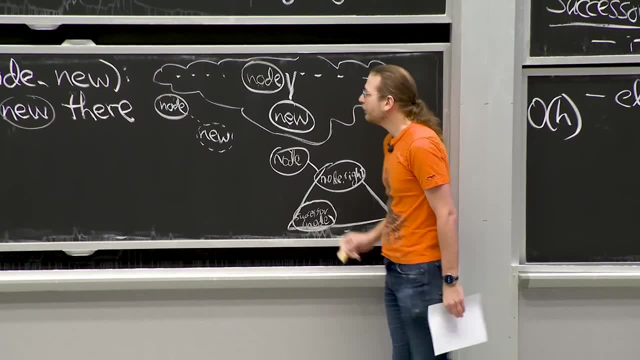 in the traversal order of the subtree, also known as the successor of node. So I'll call this successor of node in the current traversal order. But of course we'd like to make new the new successor of the node. So where does it go? 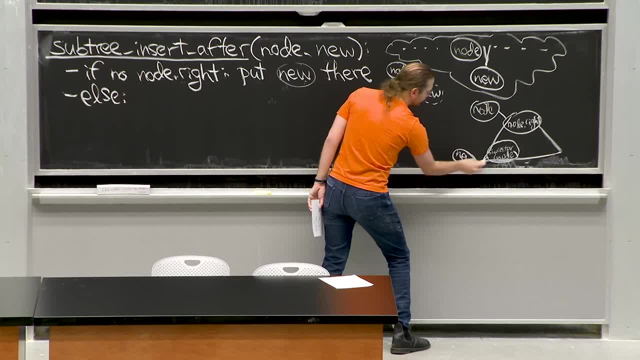 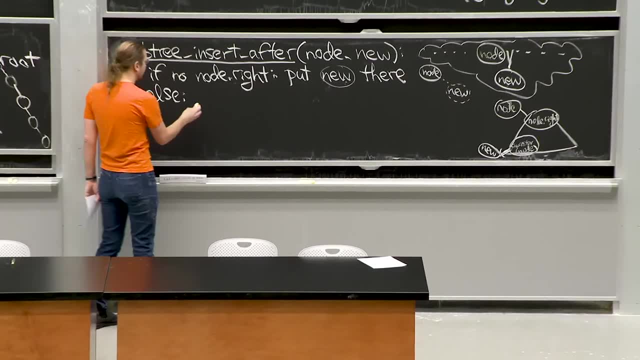 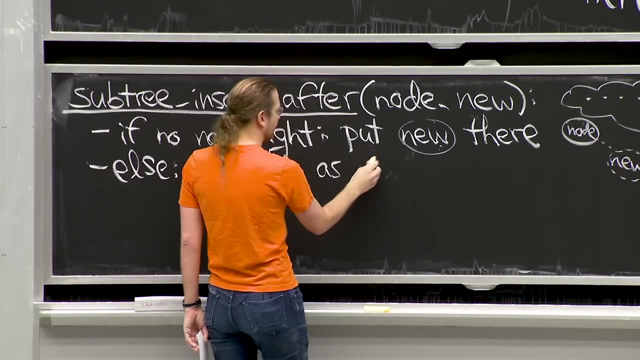 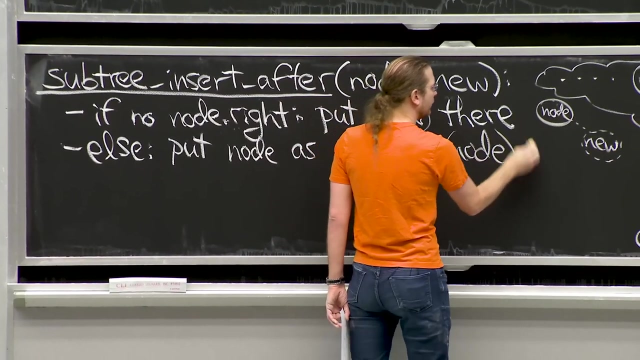 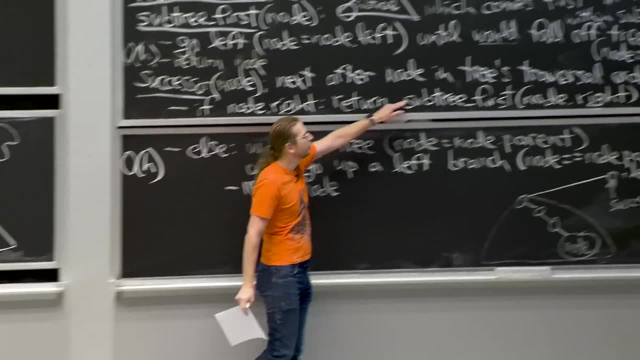 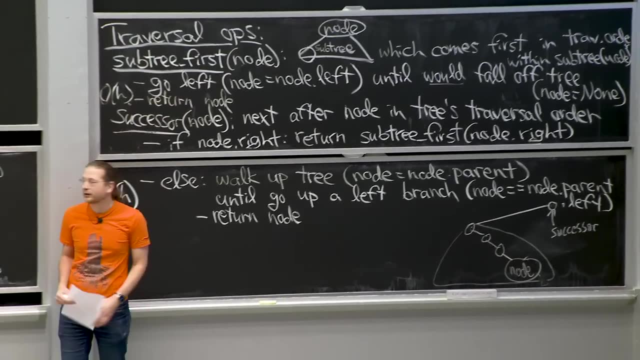 look at the code for successor. we're in this case So we know it will just call subtree first of noderight Right, And remember subtree first went left as much as it possibly could. So what that means is this successor node is guaranteed to not have a left child right. 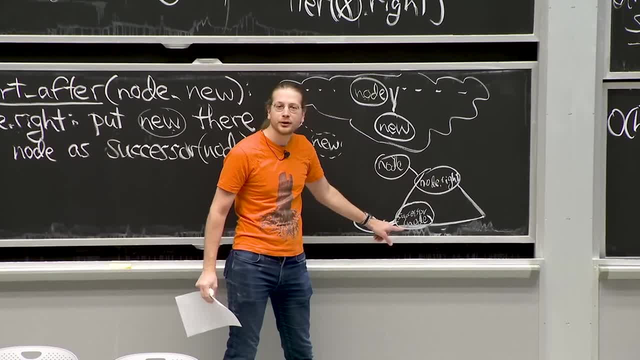 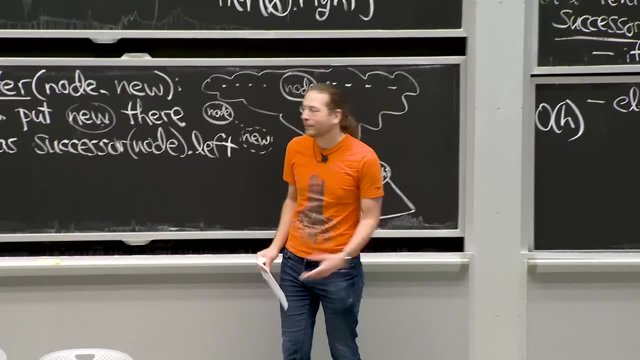 Because it was defined by going right once and then going left as much as you could. So there's no more left, which means we can make one more left. just add new there and we're done. Now, if you look at the traversal order, it will be node, then new, then the old successor. 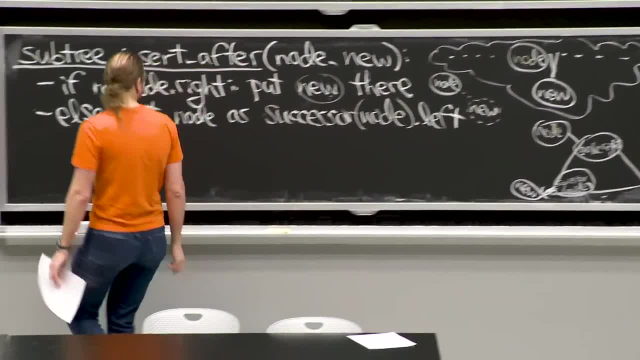 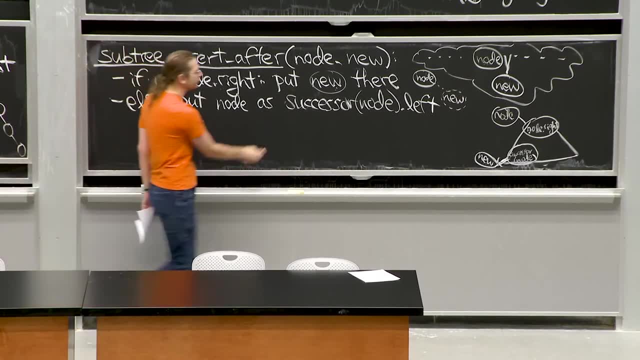 and then the rest of that subtree. OK, It's kind of cool In all cases. I mean, this was constant time Here. we spent constant time after we called successor, Successor costs order H time. so this is order H. 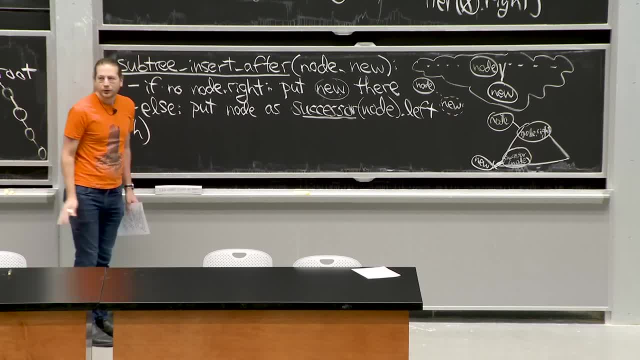 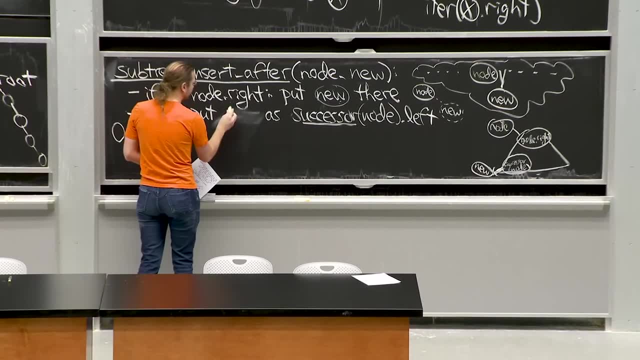 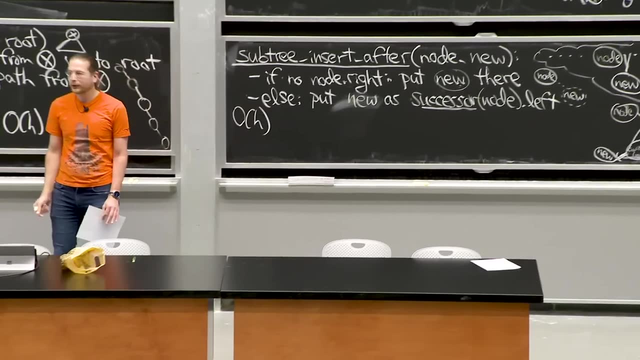 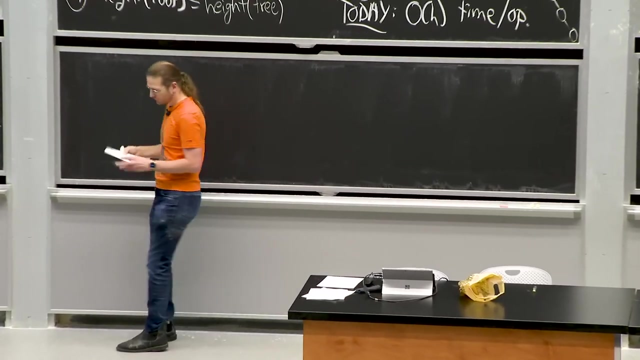 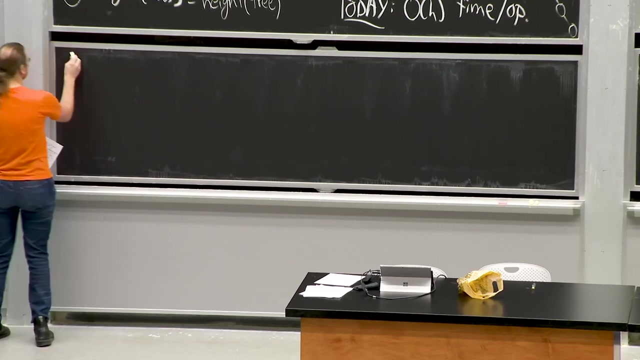 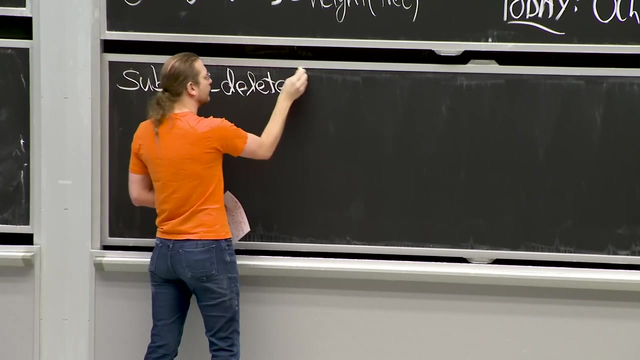 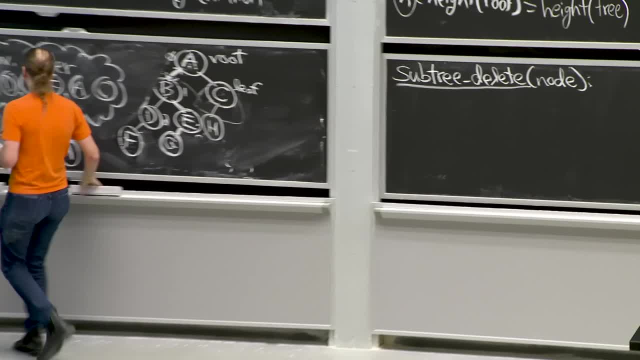 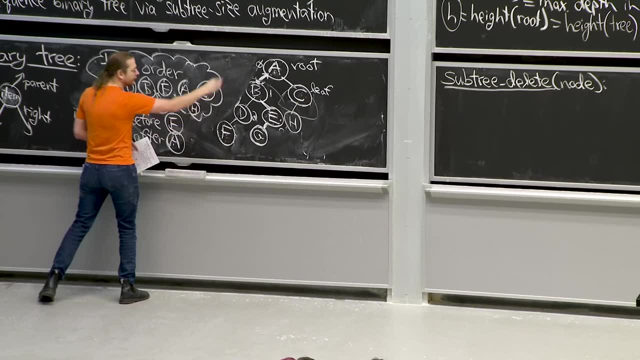 All of these are going to have two cases, So let me OK, Oh, I did an update, So now H is after A. It should be like this, And you can check: the new traversal order of this tree is exactly that. 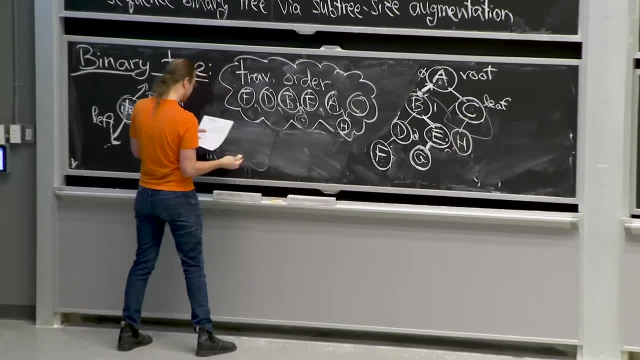 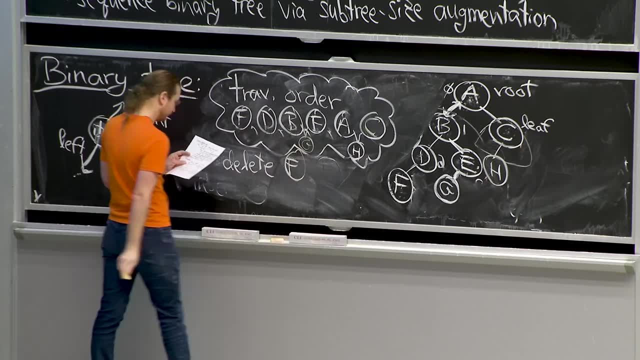 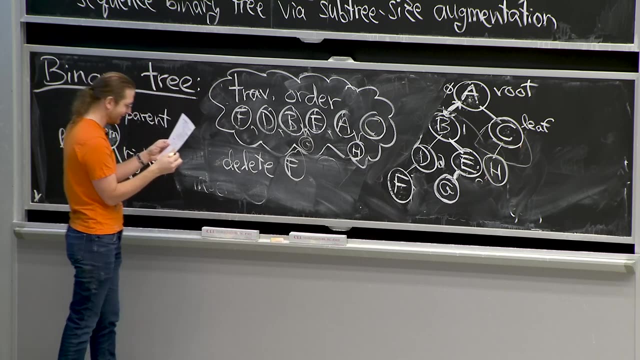 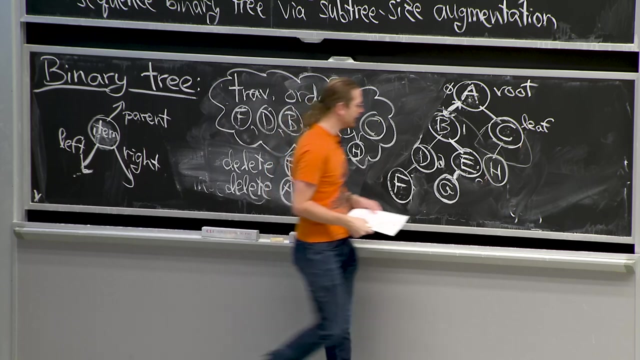 Next, I'm going to do a couple of deletions. Let's delete F first, and then we're going to- This is confusing, All right- And then we're going to delete a. So where's f? We're supposing we're given a pointer to f this node. 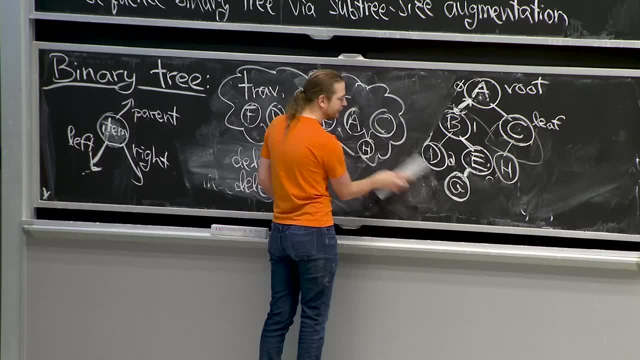 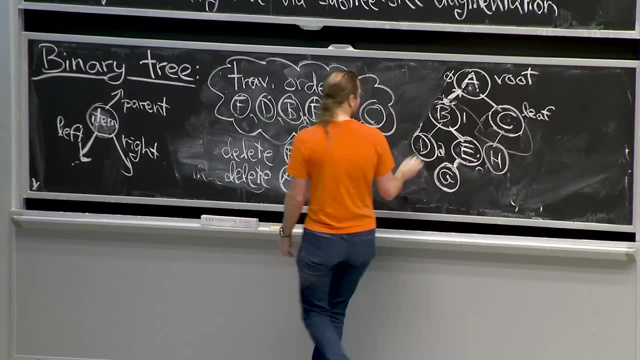 Well, it's a leaf, So if I want to delete it, I just erase it. Easy Leaves are easy to delete. There's no work to do. So what that means is I'm removing the pointer from d to f, We just erase that guy. 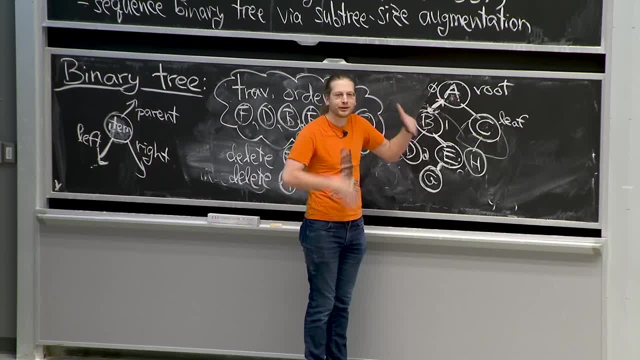 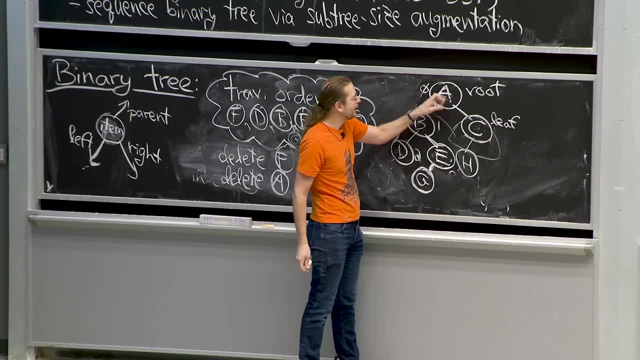 OK, now here's a trickier one. Suppose I want to delete the root of the tree. This is kind of the hardest case, But in general it would be somewhere in between leaf and root. So if I want to delete a, if I just erased it. 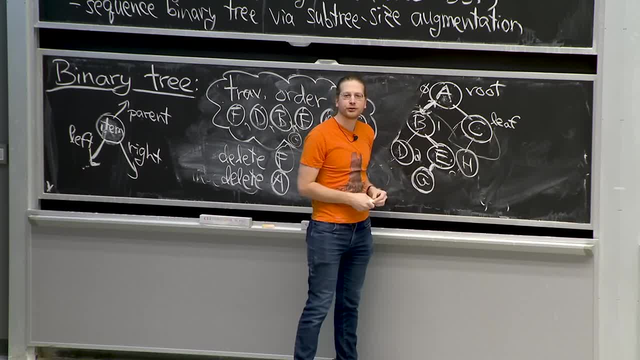 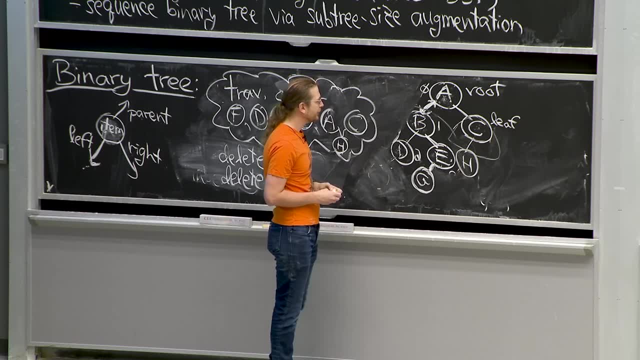 then suddenly, there are these pointers to nowhere and I disconnect the tree into two parts. I don't want to do that. I need to keep my tree connected. So I'm going to play this trick, which is I forget if I use successor or predecessor. 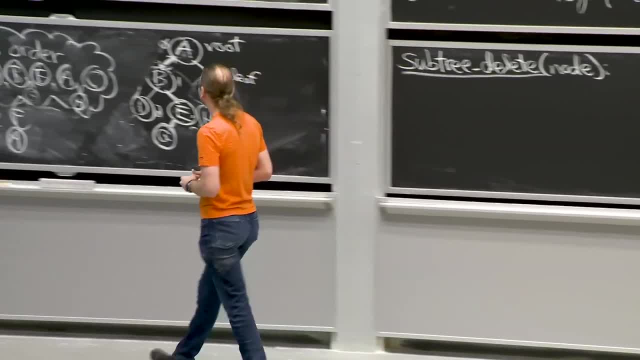 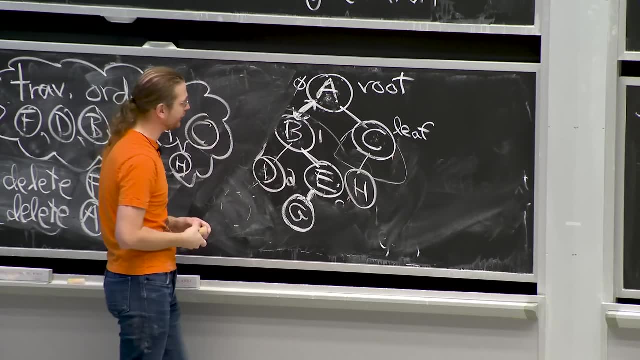 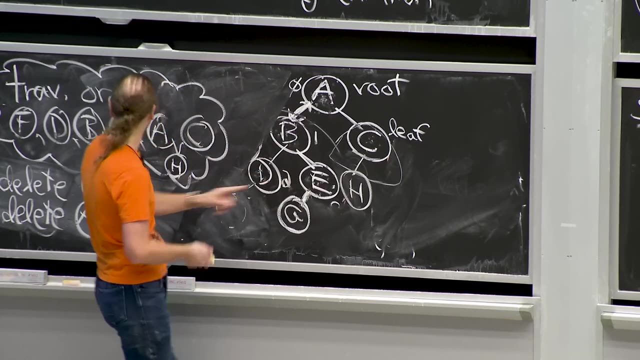 Predecessor, So I'm going to look at a. We already have defined successor and thereby predecessor, So I'm going to look at the predecessor of a, which is e. You can check that here. The one before a is e. 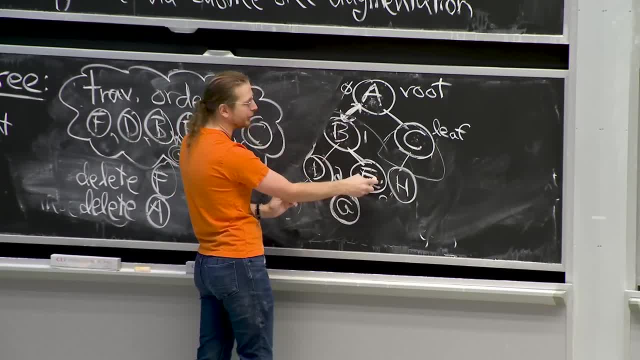 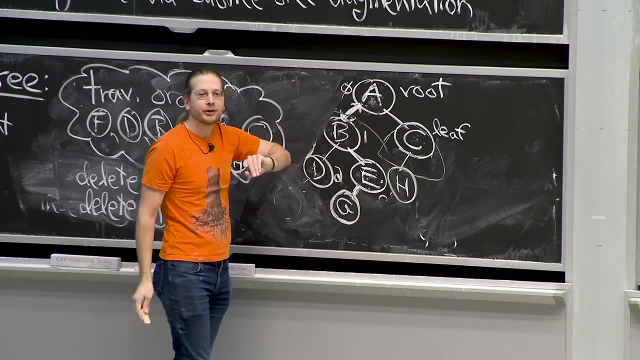 This is in the left subtree. Find me the rightmost item. Keep going right until I can't. That's e. So now these guys are adjacent in the order and I'm about to remove a from the order, So I can momentarily cheat and swap. 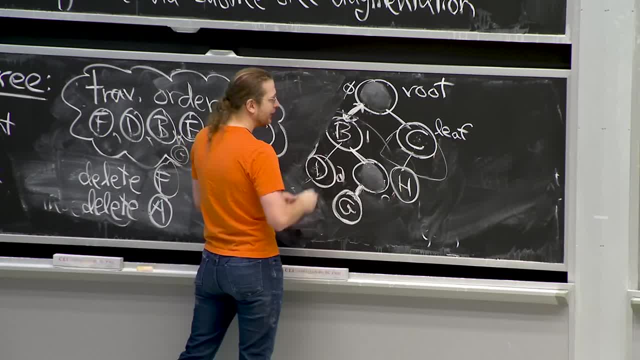 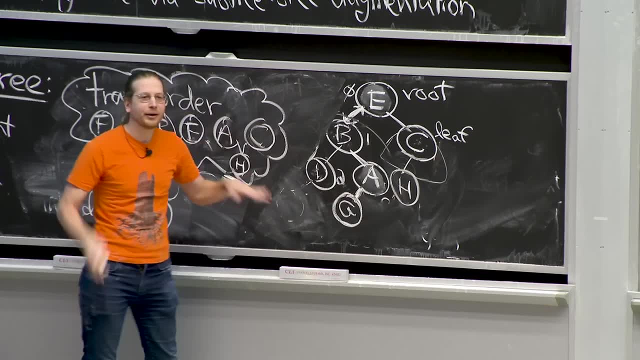 They're labels. I'm going to erase a and e here and put e after a. Why? Because it moves a down in the tree And if I get to the leaf I'm done. So I'm not quite done, because this is not a leaf. 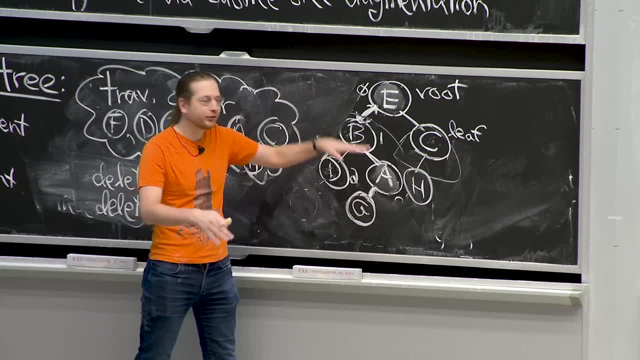 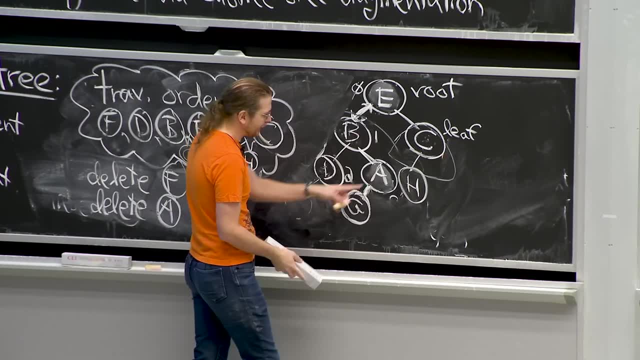 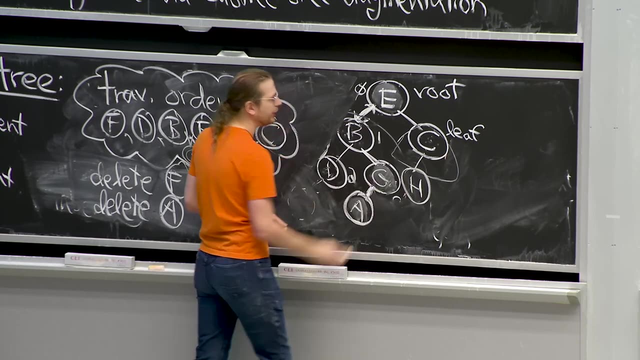 So again I look at a's predecessor. It's now g Predecessor. we hope is always farther down in the tree. And then I swap a with g. I have preserved the traversal order, except where a falls just by moving a earlier in the order here. 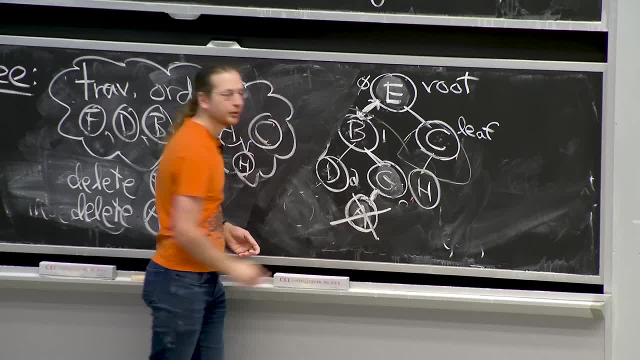 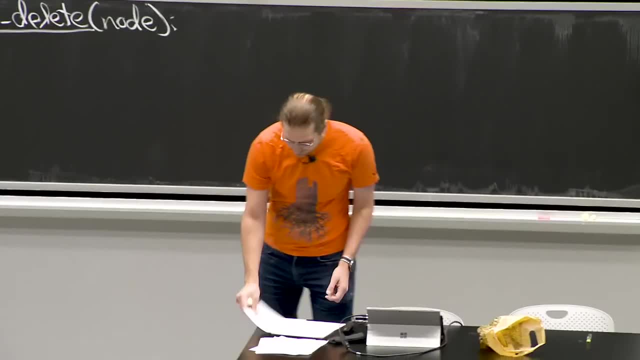 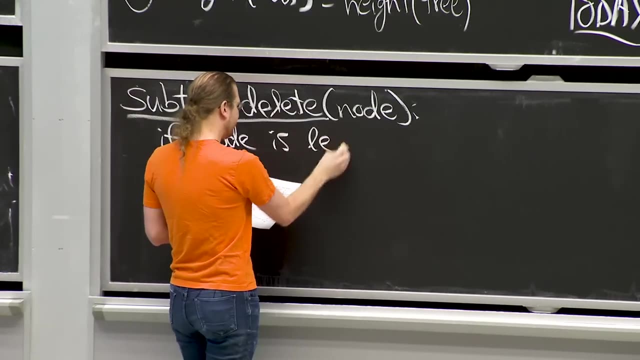 And now a is a leaf and I can erase it, So that's what we're going to follow. Now, in actuality, it's a little tricky. Sometimes we need to use predecessors, Sometimes we need to use successor. So the cases are: if the node is a leaf. 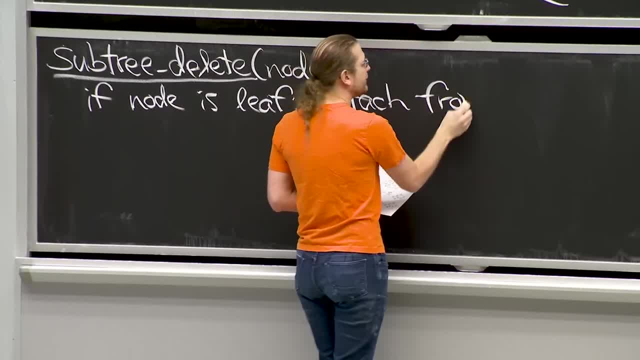 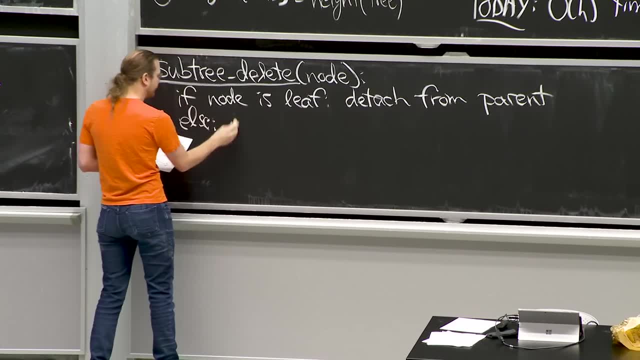 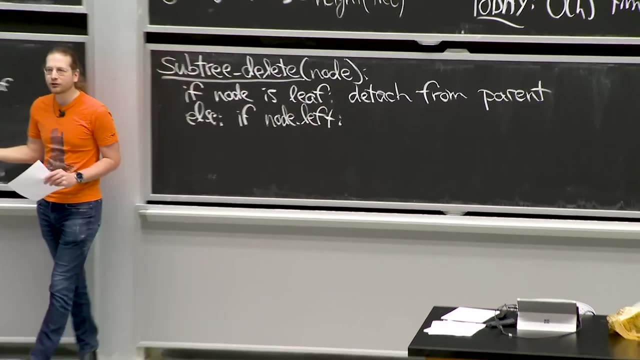 just detach it from the parent Easy. That's sort of our base case in the recursion. Otherwise there are two cases. So if we're not a leaf, that means we have a left child or a right child or both. Both is going to be the easy case. 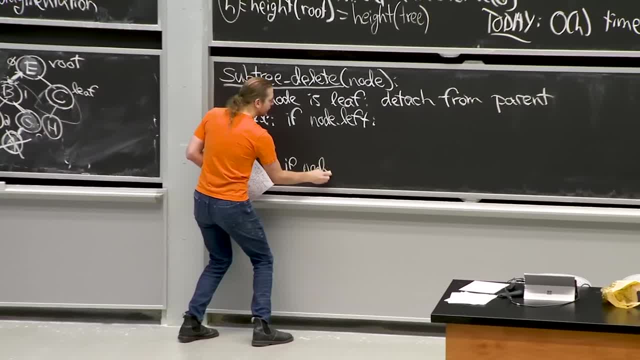 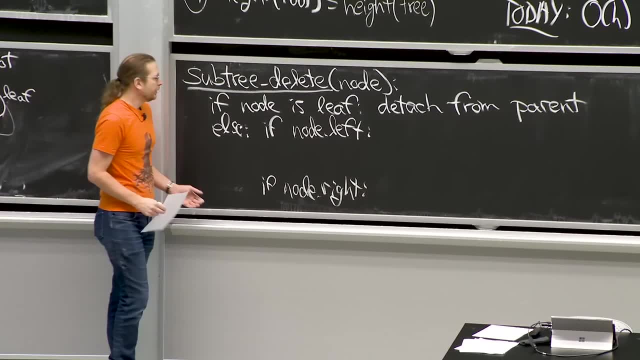 But in general I have, either there's a left child or there's a right child. In either case I'm going to be happy, so I don't need it A both case. So what do I do If I have a left child? that guarantees to me. 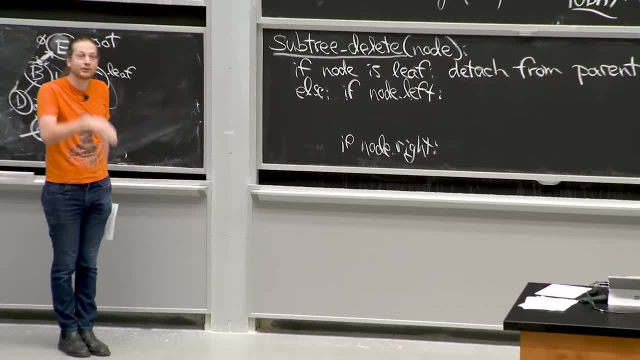 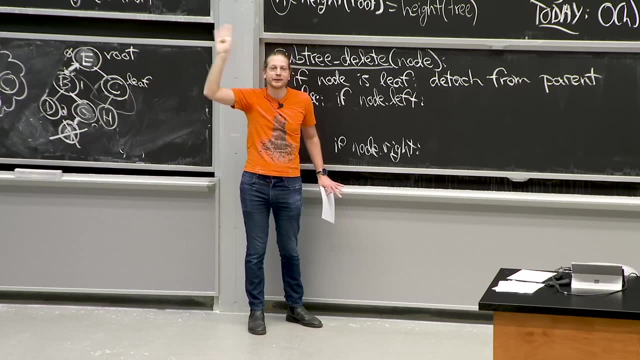 that the node's predecessor is inside that left subtree, which means it's lower in the tree. If I didn't have a left child, the predecessor would actually be higher in the tree and I don't want to go higher. So if I have a left child, I know the predecessor is lower. 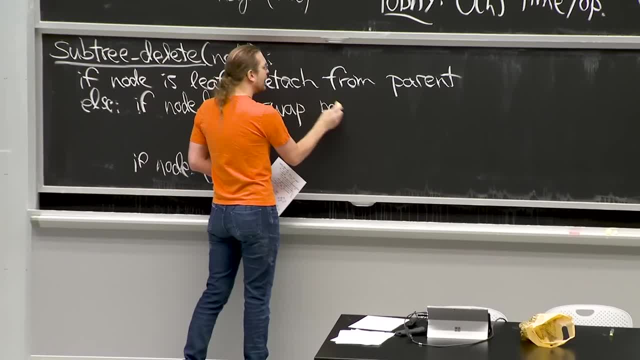 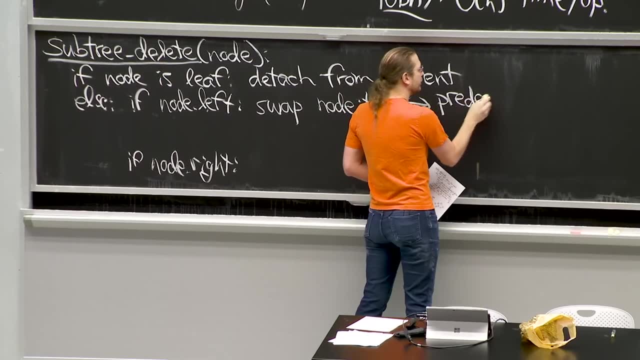 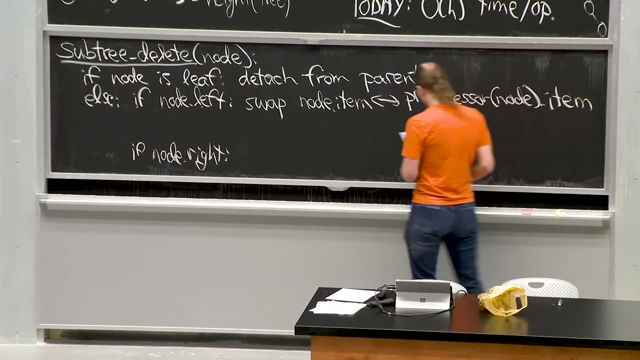 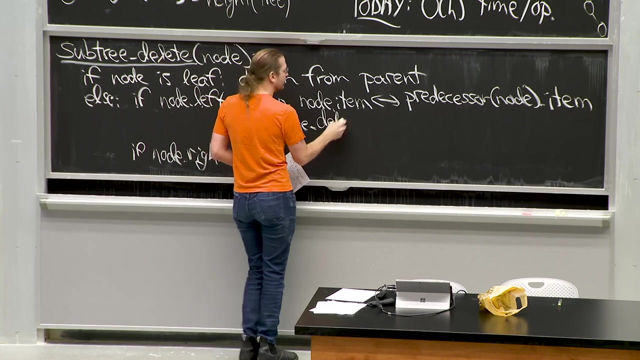 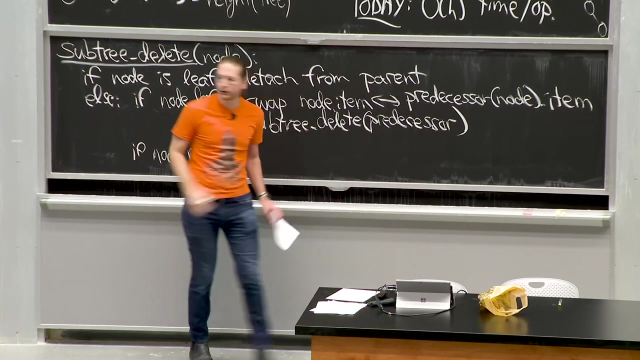 and so I'm going to swap my item, the contents of my node, with my predecessor's item and then I'm going to recursively delete the predecessor. And that's the case that we looked at in this code, in this example, because we always had a left child. 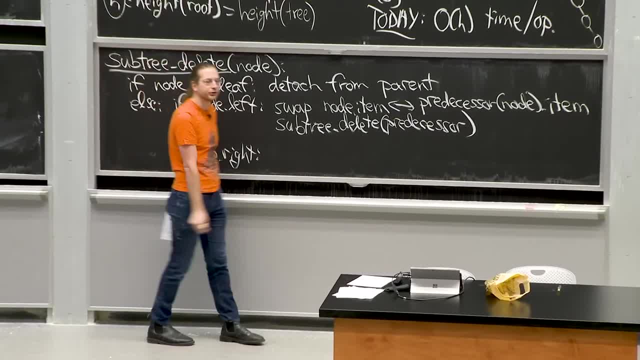 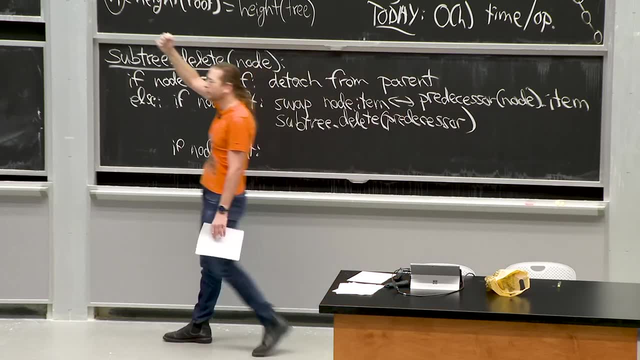 If we have a right child but no left child but no left child, we just do the reverse. We swap with our successor's item and then delete the successor. In either case we're going down, And so if we start at some node like the root, 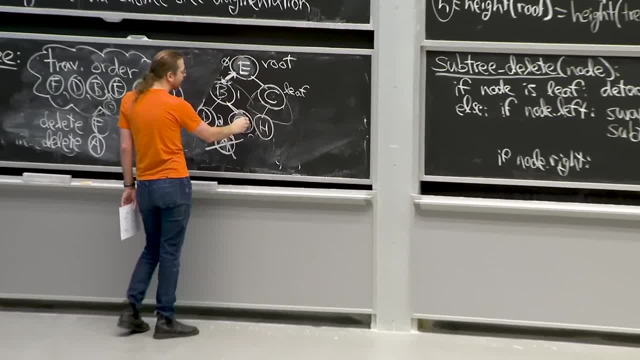 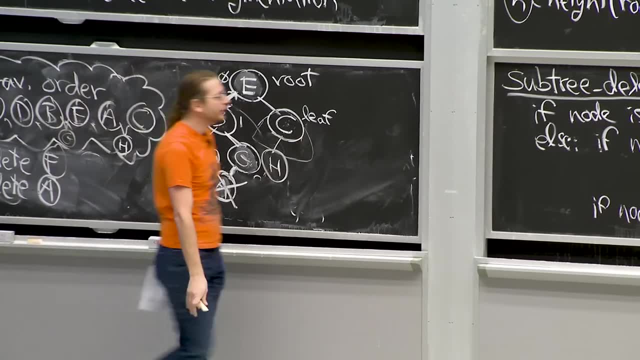 every time we do this operation, we're walking down and then we're walking down And in general, we'll keep walking down, resuming where we left off, which means total amount of time we spend is proportional to the height of the tree in the worst case. 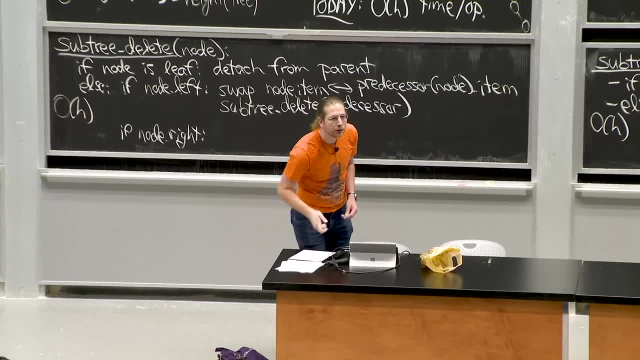 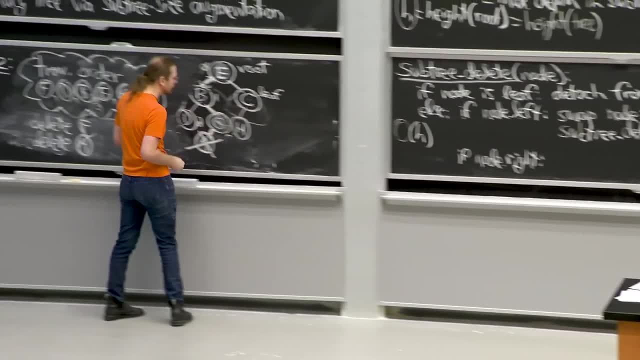 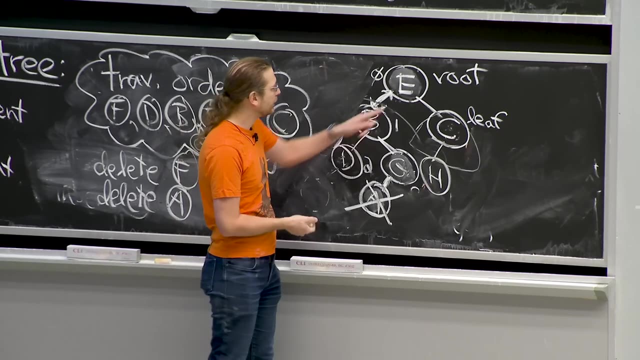 Question: Why isn't there a What would be the Right? so e didn't used to have a right child. So we're changing identities of nodes when we do this, because we didn't actually move this circle. The circle stayed in place and what we changed? 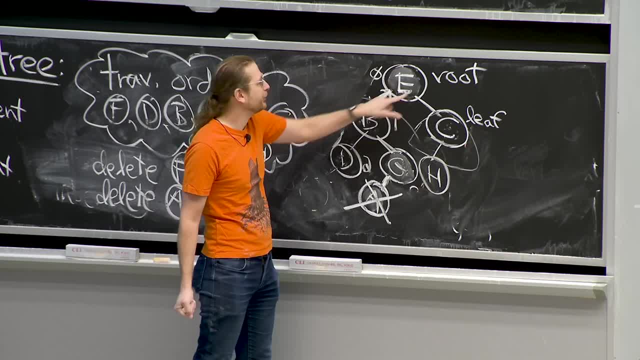 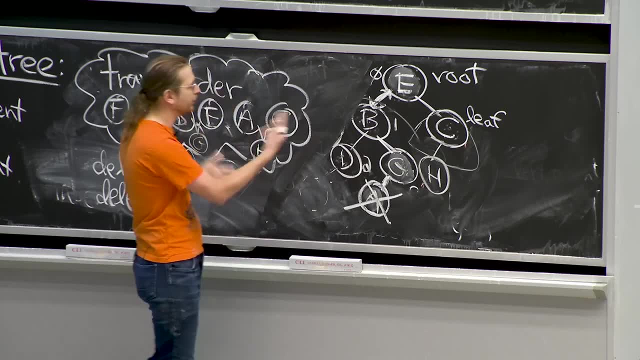 was the item that was stored in that circle. So whether you call this node e or a, it doesn't really matter, It is just the root node. So we're going to play a lot of these tricks of moving the items around. So far we hadn't been doing that. 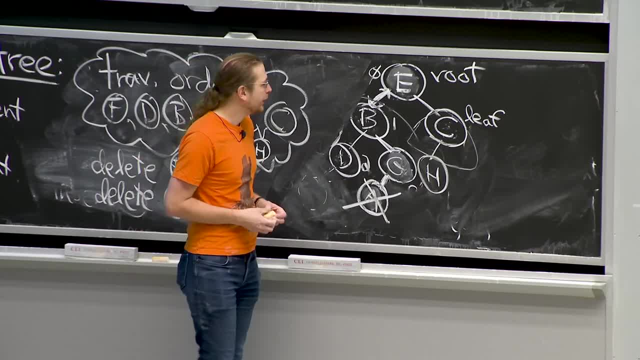 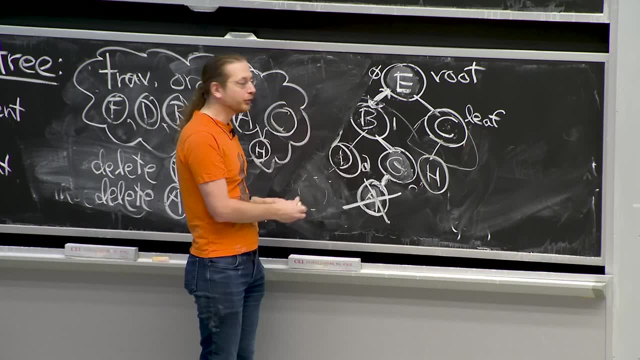 We've just been creating nodes and placing them somewhere, But now, in this delete operation, this is the first time where we're changing what's stored in the nodes, But we still can define the traversal order. The traversal order of this tree is d, b, g, e, h, c. 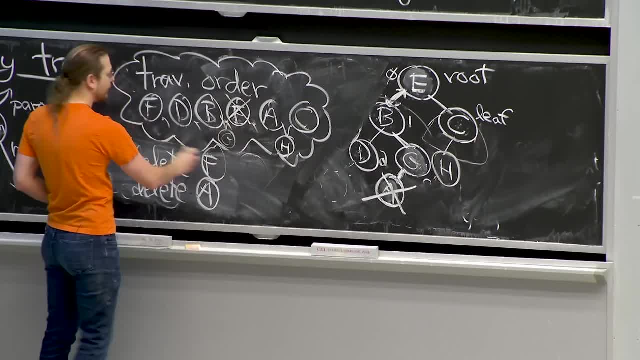 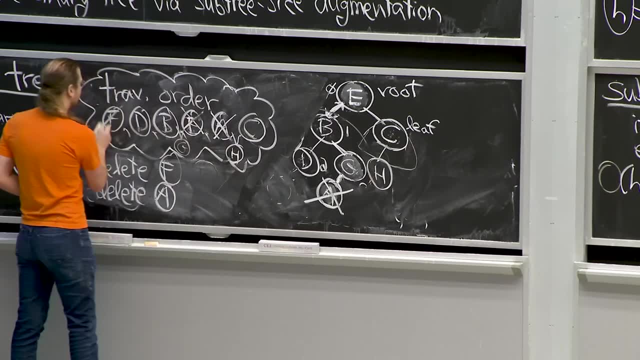 which should be what we get here if I delete f and a. What if you created a tree and, Sorry, can't f? It really matters, It really matters. You're really mad at the tree, so you're going to connect it that way. 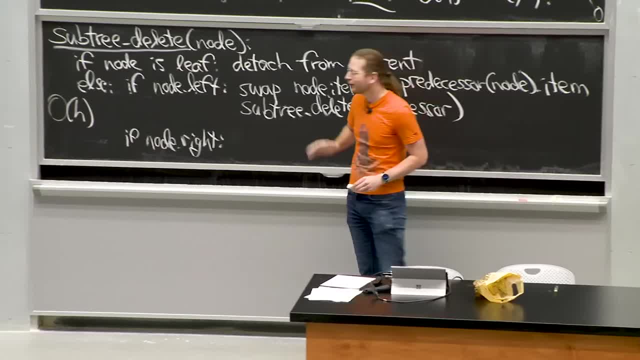 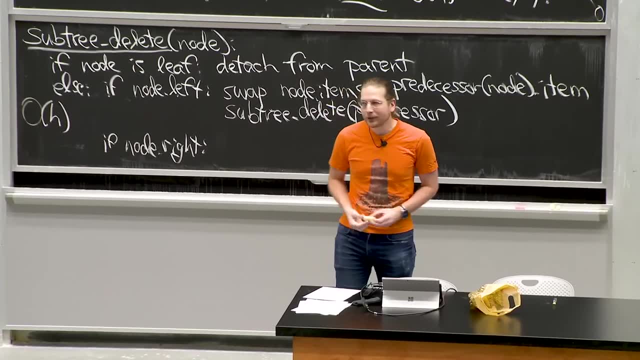 Trees will not preserve connections. That's just the name of the game. We have to allow this, otherwise we can't do anything. That's the short version. In the last few minutes let me talk about how we take these trees and implement. 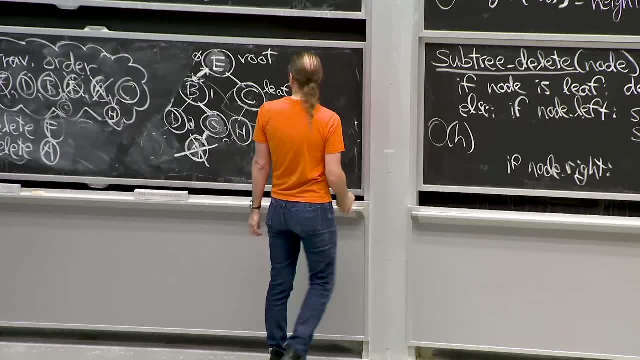 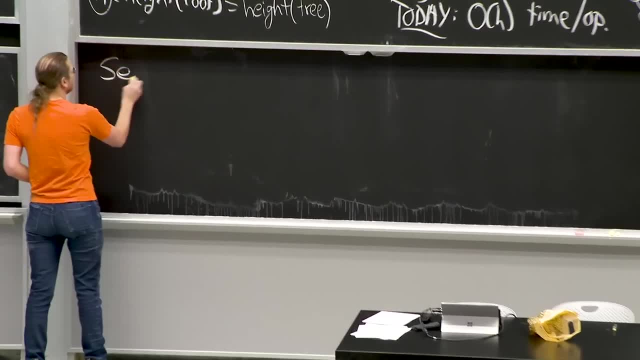 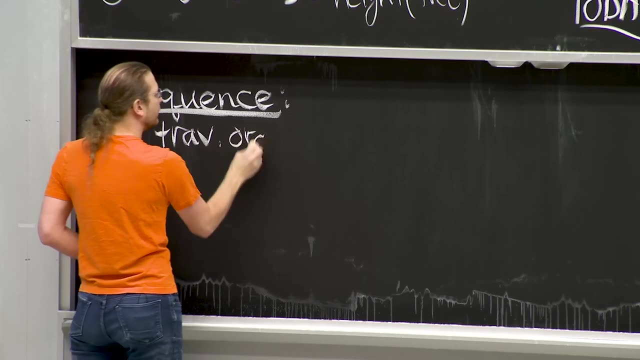 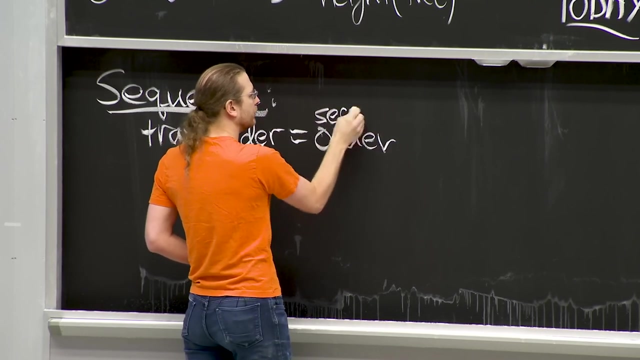 a set or sequence. I've already alluded to this. So for a sequence, We just make the traversal order equal to the order that we're trying to represent- the sequence order- And if we're trying to sort a set items with keys, 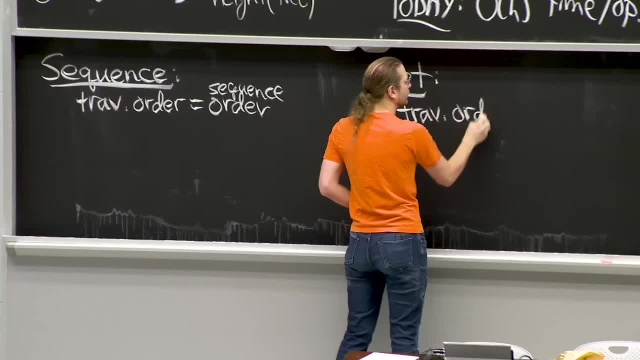 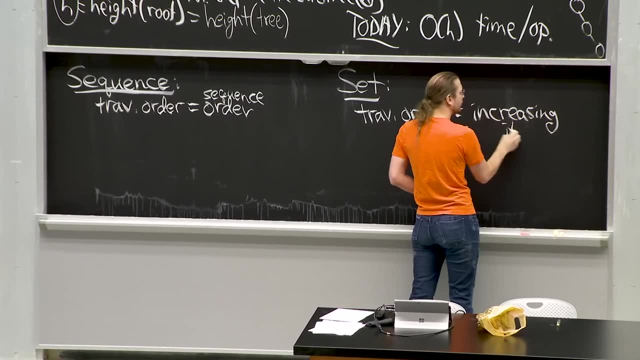 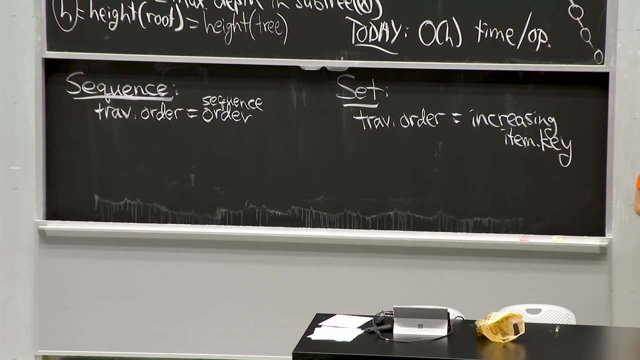 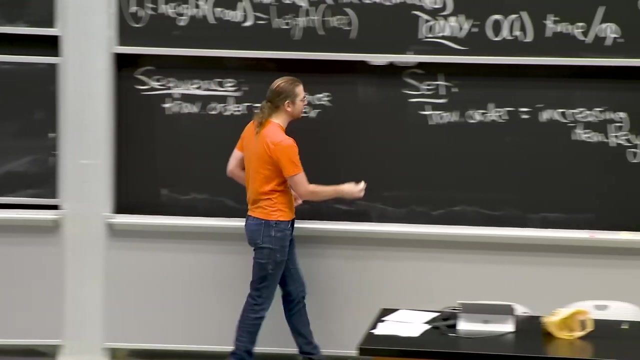 we're going to make the traversal order equal to ordered by increasing key Increasing item. Increasing key Increasing item. In some sense that's it, But then we need to think about how do we implement all of these operations. So maybe most enlightening is for starters, 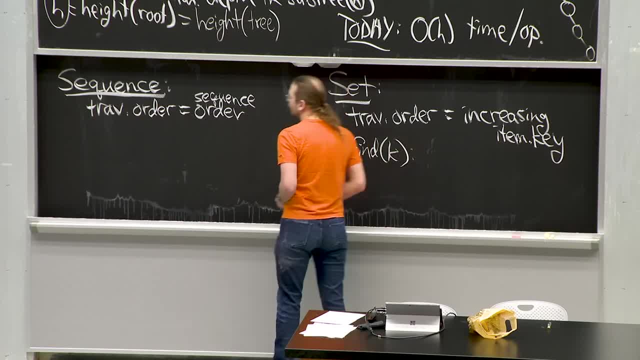 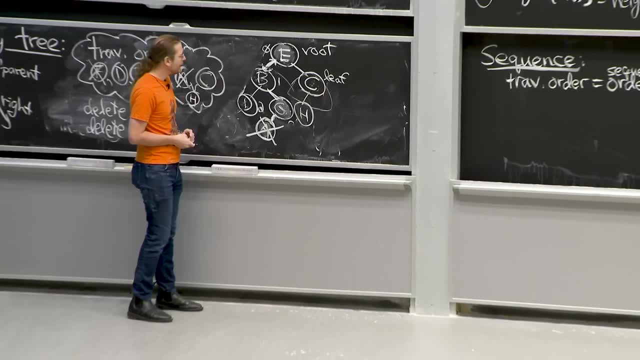 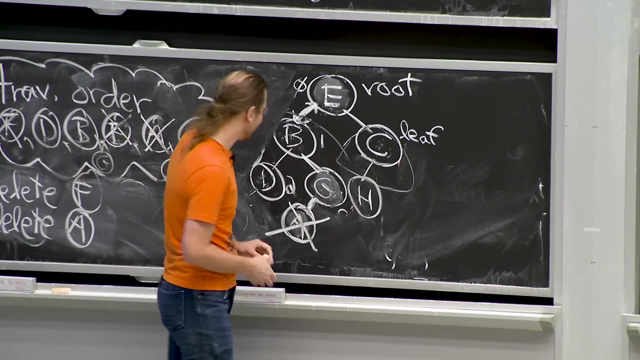 is finding a key in a tree, So this is going to correspond to binary search. If I'm searching for a key, let's say I'm searching for G's key, And I know this may be hard in this example. maybe I'll replace these all with numbers. 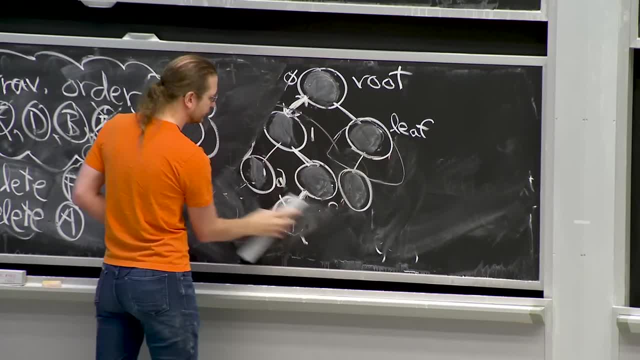 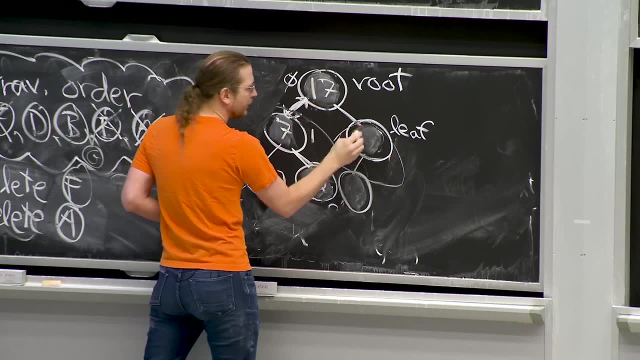 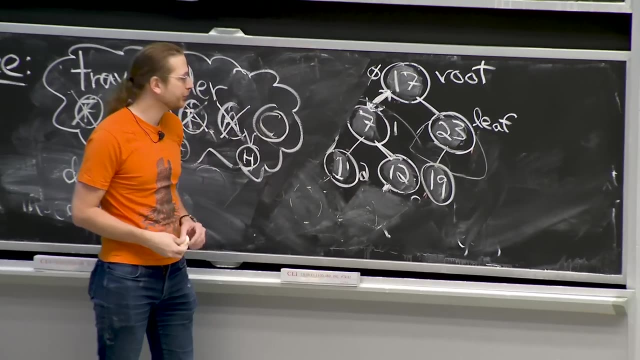 so I can think about key values. So let's say 1,, 7,, 12,, 17,, 19, and 23.. This is now in key order. if you think of the traversal order, The property is that all the keys in the left subtree of the root. 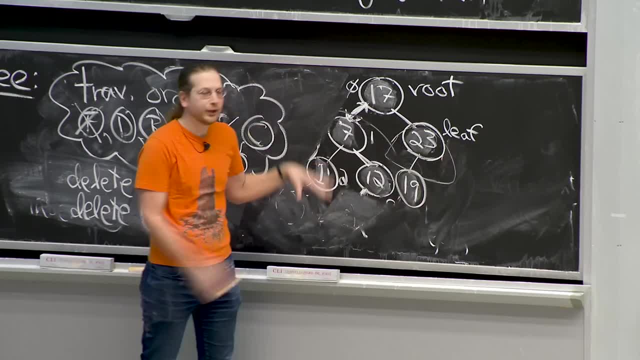 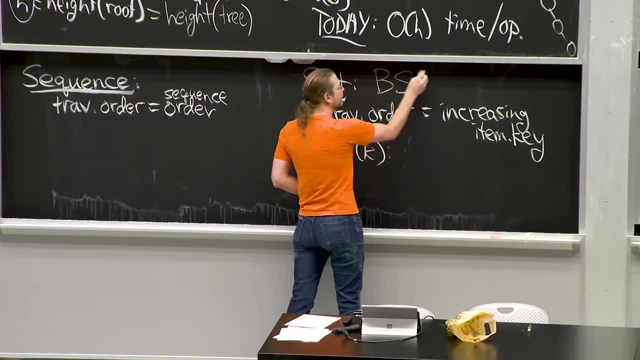 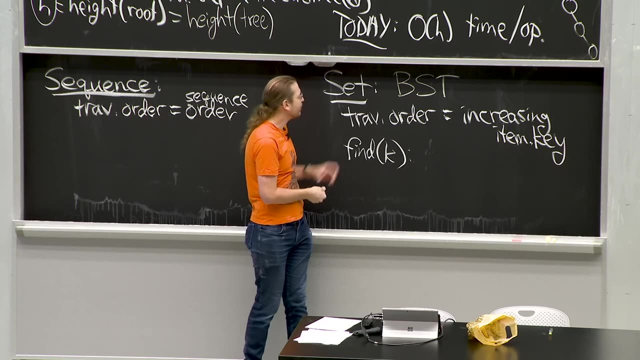 are less than the root And the root is less than all the keys in the right subtree and recursively all the way down. This is something called the binary search tree property, BST property- Here we're calling them binary tree sets or set binary trees. 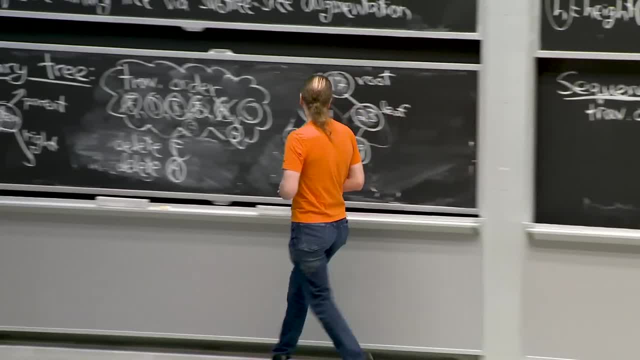 But they're also known in the literature as binary search trees, a term you may have heard before. So this is a special case of what we're doing, where we're storing the keys in order And then, if I want to search for a key, 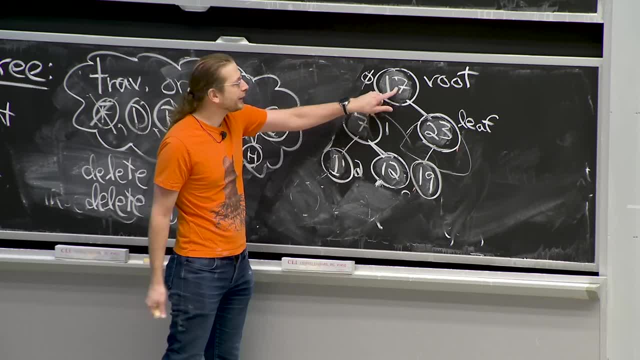 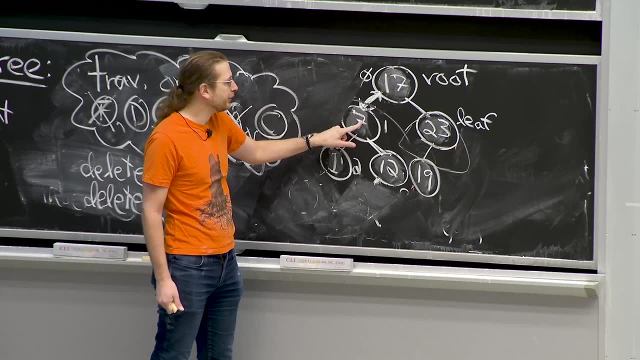 like 13,. I compare that key with the root. I see, oh, it's not equal And it's to the left because it's less than 17.. So 13 is left of here, 13 is right of 7.. 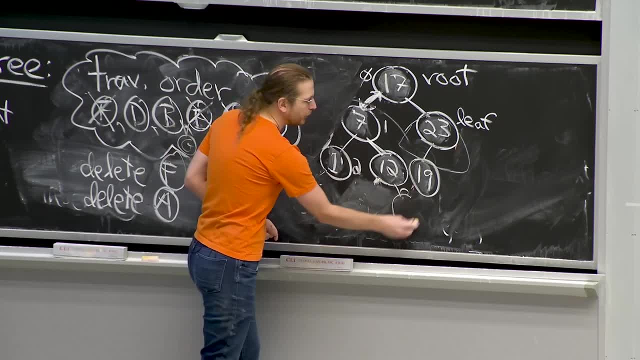 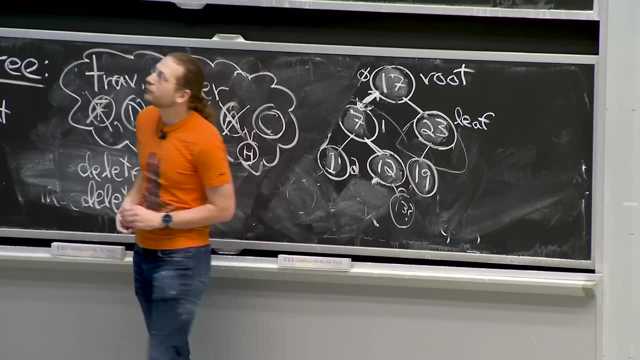 13 is right of 12. And so I know that this is where 13 would belong, But there's no right child there, And so I know in find I just return nothing. If I was doing find previous, I would return this node. 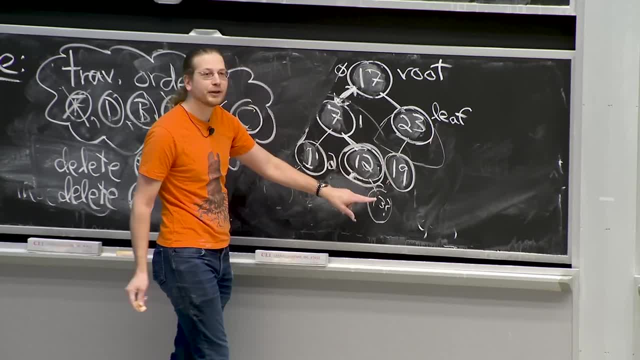 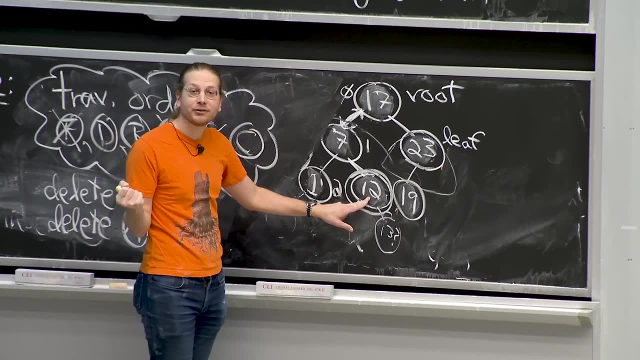 Because I have tried to go to the right. the last time before I fell off the tree I was trying to go to the right And therefore that last node I had was the previous item. If I was trying to do find next, what would I do? 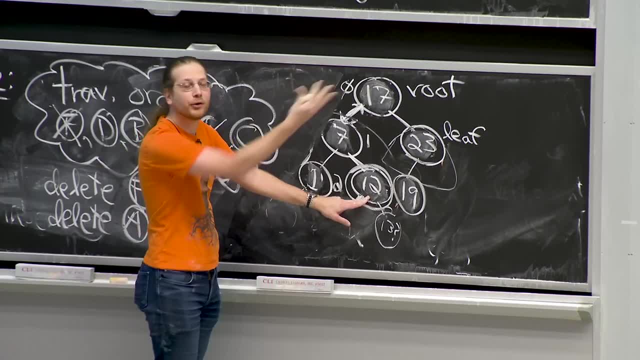 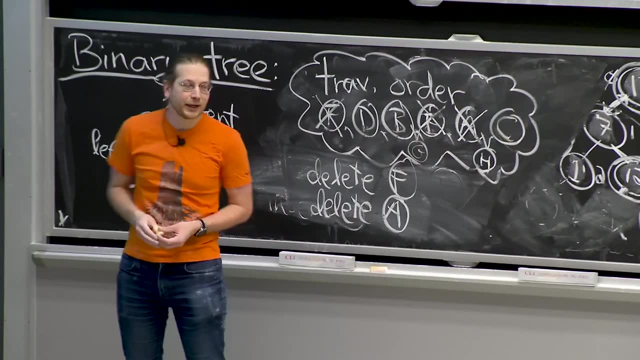 I would just take this node and compute its successor, which we already know how to do, And that happens to be the root. So now I can do these inexact searches When I do find previous and find next when I fall off the tree. 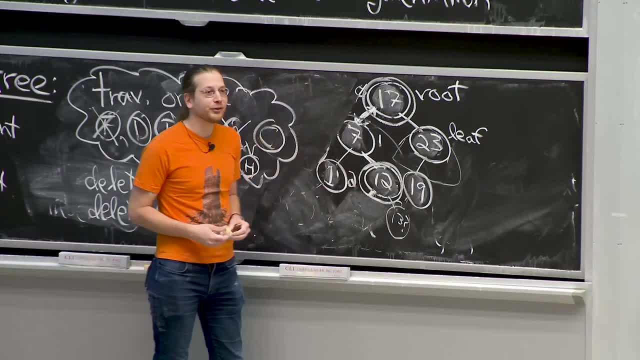 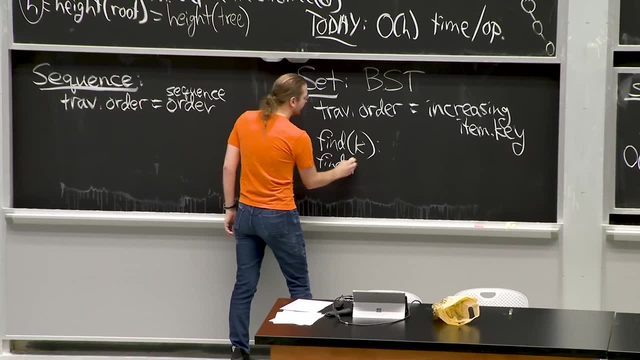 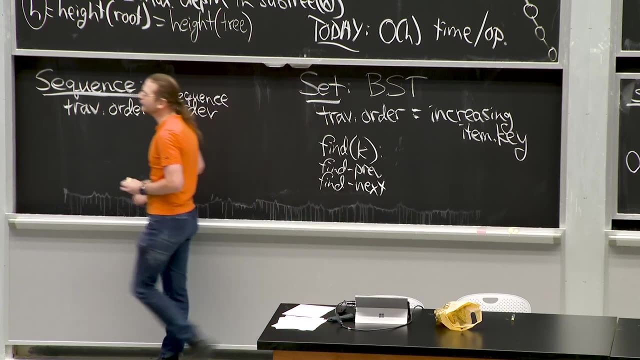 I find either the previous or the next, And then, with predecessor or successor, I can find the other one. So that's how we can do So: find and find previous and find next. To do sequences, we need a little bit more work. We'll do that next time.